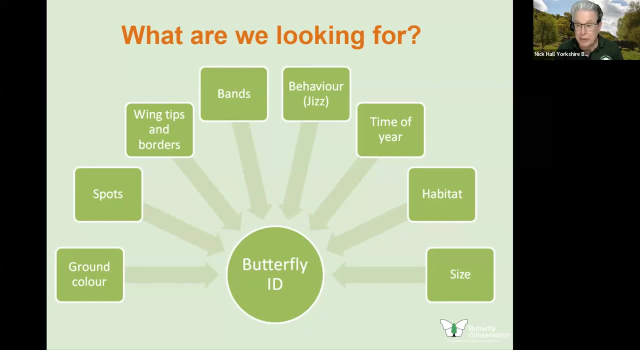 the brown species all have different arrangements of spots and we can use those for determining species. When it comes to the whites, which I know for most of you is the most tricky family of butterflies, wingtips and borders are really important, And the big showy. 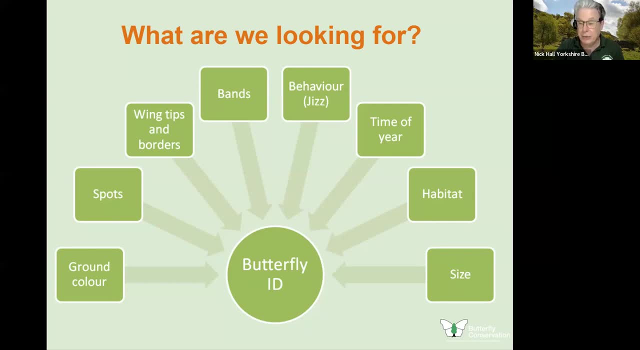 butterfly is what we call the venesids, like the small tortoiseshell and the peacock. They're all to do with bands. They have wide bands of colour across them. They're very showy different colours. The next, most important probably, is behaviour. What a bird person would call the giz of a? 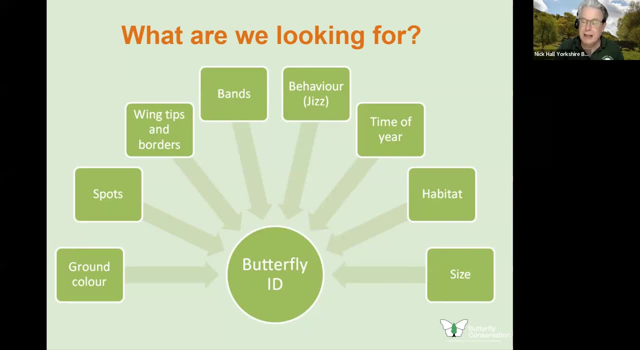 species, how it flies, how it's behaving- Really important one Time of year. obviously, butterflies only live for well, some only live for a day or two, Some will live for a whole year, but the average is about 10 days And they're within certain flight periods, So it's very 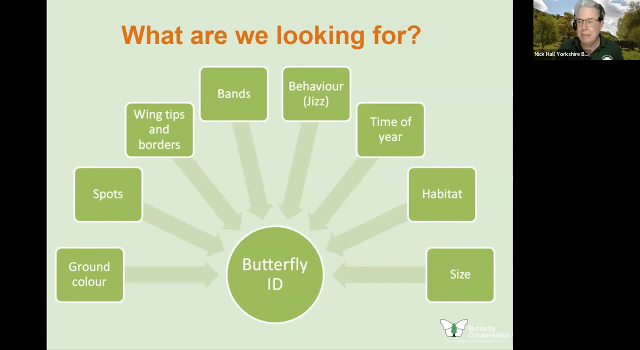 important that we know a little bit about what we should expect at any particular week of the year. Equally important, whoops, is habitat, where they're actually flying. So you only see woodland butterflies generally in a woodland habitat And heath butterflies in a heath, etc. When we 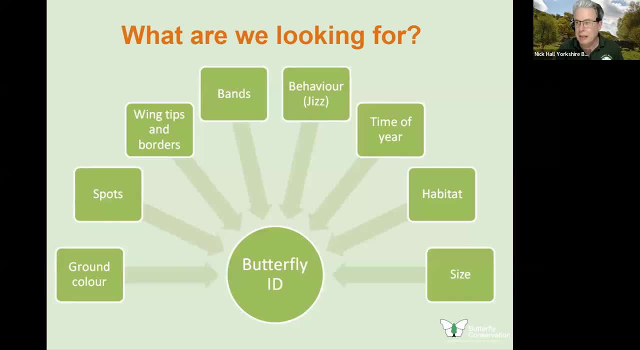 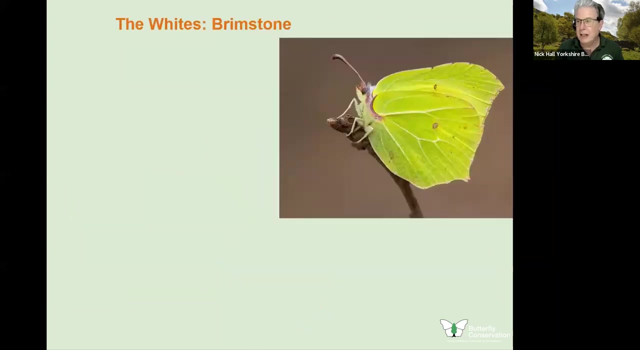 move from open countryside into woodland, those species are going to change quite dramatically. Size, of course, is very important because it gives us a lot of clues as to what the species is. So let's carry on and see our very first butterfly. 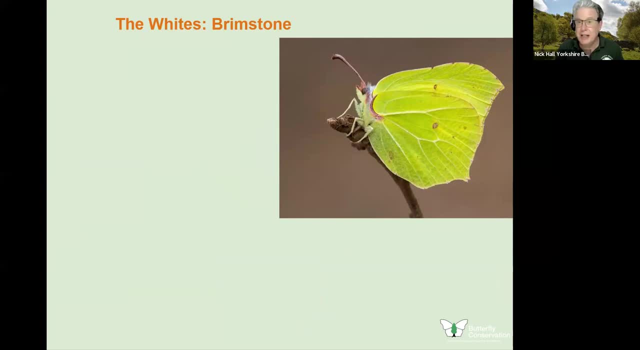 So this is the family called the white. So this is the family called the white. So this is the family called the white. Tonight is divided into families, So at the end of each family, we're going to invite you to ask any questions you have. right then, while it's fresh And just to break it up a bit, 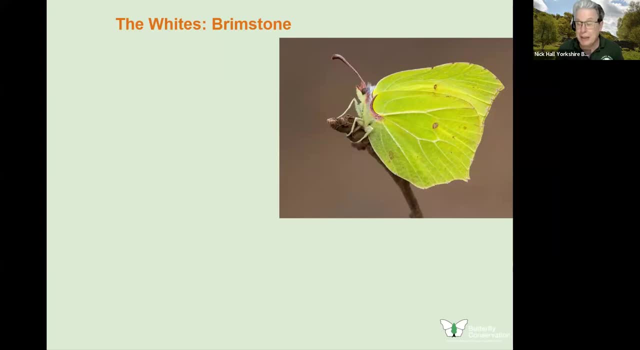 because it could get a little bit monotonous. death by PowerPoint. I'm trying not to keep putting a load of text on the screen. I'm going to put it in in bits and pieces so as to keep your eye in roughly the right place on the screen. Otherwise it's going to get a little bit tiring. So let's proceed. 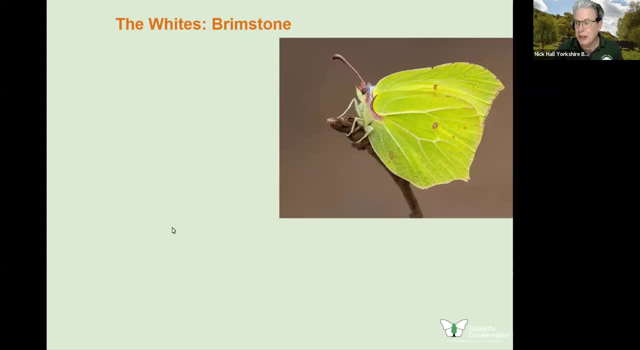 The brimstone and I hope some of you have already seen one. this year I've seen two or three, not big numbers. It's a large butterfly. It's often the first butterfly to emerge from hibernation, but can actually be seen in almost every month of the year, all the way through. Quite characteristic. 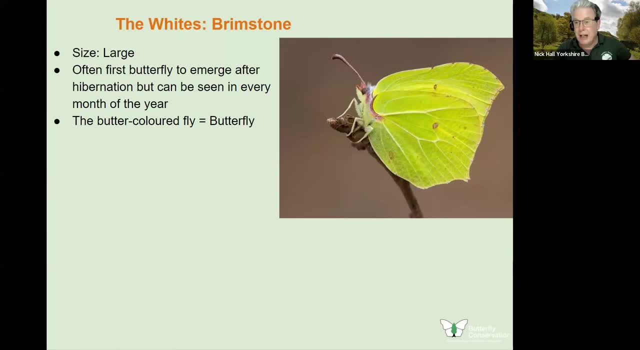 In olden times it was called the butter-colored fly, which then was transformed into the word that we know, butterfly. So that's the origin of the word The male. of course, is this distinctive yellow color a joyous color. when you see the first one of the year, It's a wonderful sight. 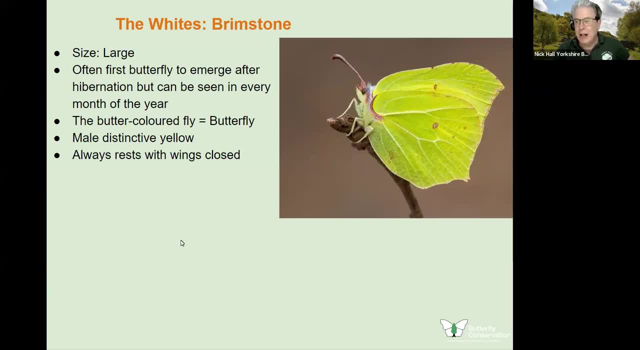 Always rests with its wings closed. It's almost impossible to get a picture of wings open with a brimstone. It's a very good reason. is it's camouflage? You see all those wing veins. It's trying very, very hard to look like a leaf. And if you're going to look like a leaf, 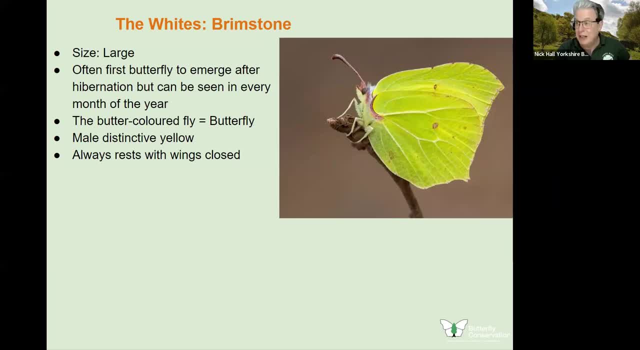 you've got to be closed up and hiding on a leaf. And you'd notice, in its effort to look like a leaf, it has these points on its forewings and hind wings. Now, if you're lucky, if it's flying slowly, 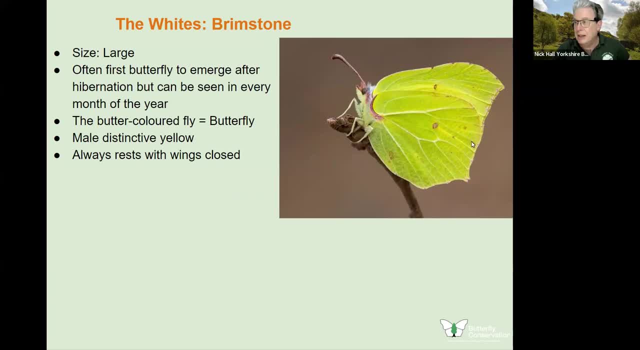 you can actually pick out those points on the wing. It also has these wonderful like broken veins with little red marks and little orange spots like fungal infection on the leaf. It's a quite remarkable feat of camouflage And there's good reason, because they are heavily predated by birds. 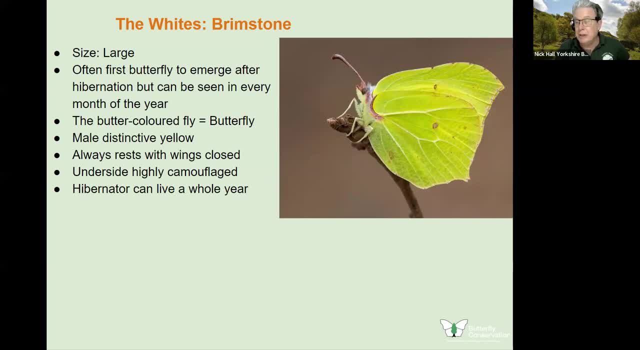 Now. a individual butterfly can live for almost a whole year, So the insects that we're seeing right now were emerged back in probably July, beginning of August, So they're already what nine, nearly coming on 10 months old. They have remarkable longevity And also 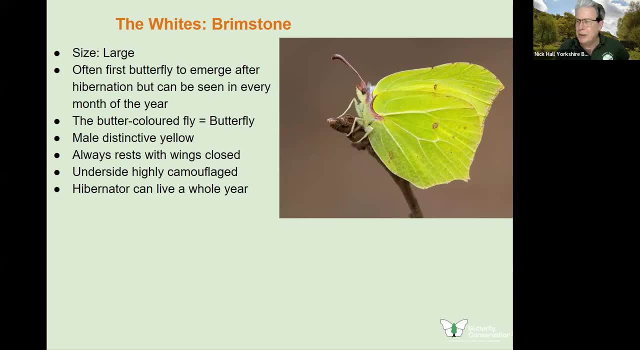 you will notice a lot of butterflies get tattered and torn and bits missing. The brimstone never. it's always almost pristine. A remarkable feat. It's a great wanderer. It does favour the woodlands If you want to see large numbers. 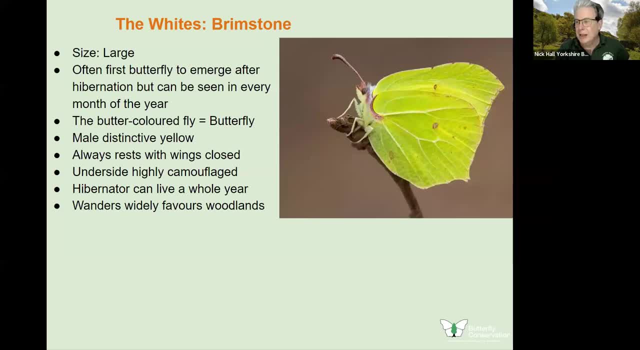 of brimstones go to woodland and there's quite a few in Yorkshire and there are transects in some of those woodlands. So I know on my particular transect I can get on a particular day 20 or 30. Well, normally 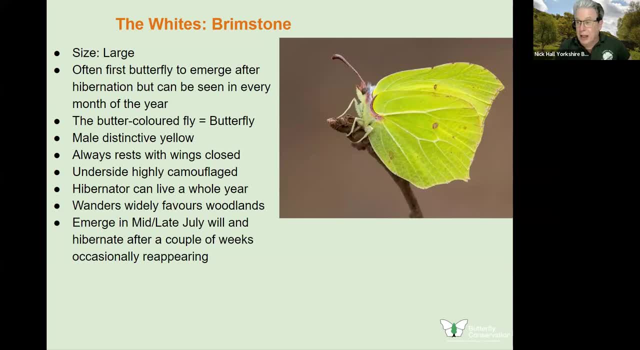 our garden if you only see an odd one. So they emerge from their pupa in mid to late July and will hibernate usually after a couple of weeks. so they will be feeding up in that period and then they will occasionally reappear. It depends on the weather. nobody really knows what causes them to. 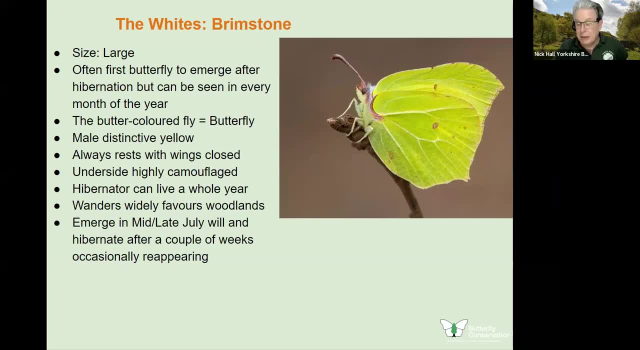 reappear, but they will reappear in the autumn, quite sometimes in good numbers, but it's very variable. The fact you see none in September and October doesn't mean they're dead or gone away, they're just hibernating. Now the females are very different, and obviously because they're white, 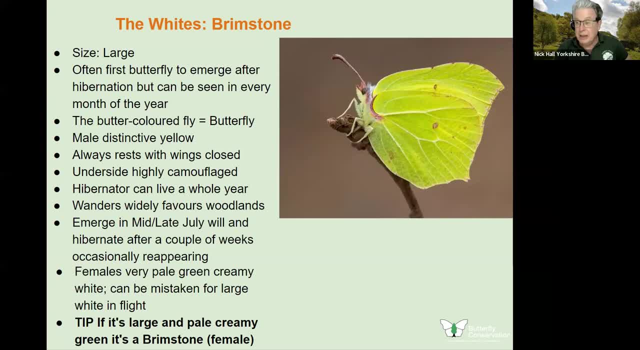 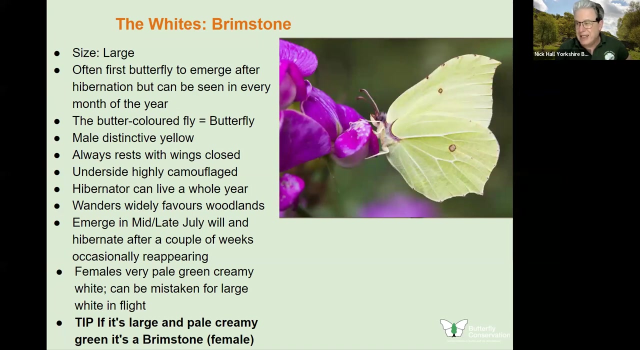 they are very easily confused with large whites. They share a lot of similarities in terms of size, about the same size as the large white butterfly. So how you tell them apart is obviously: the males are the yellow color, but the females are this. are this, I'll show you- are this wonderful, slightly green, greenish shade of. 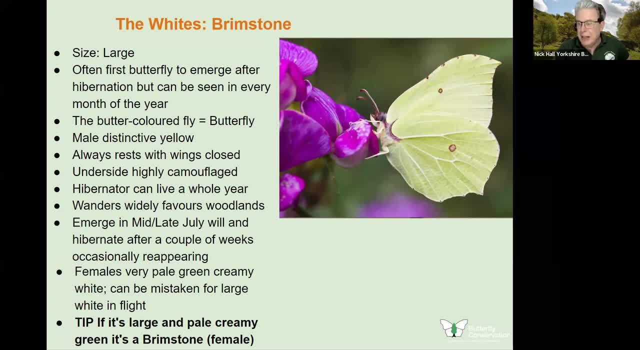 cream, kind of a creamy green. It's difficult to tell when they're in flight, but they do give out a little bit of green as they go past you, And you can occasionally, as I said before, just see those little white butterflies that are in the middle of the garden. 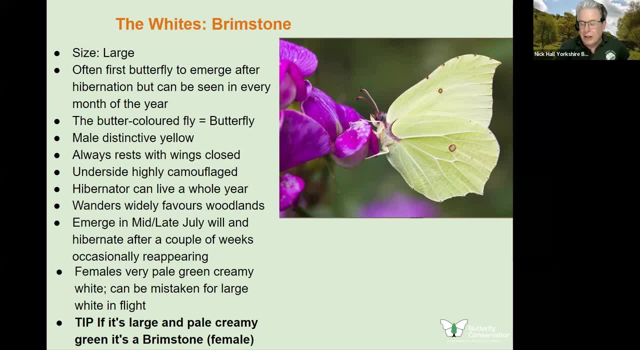 So you can see those tips on the wings. So if you get the chance to check them, if they land, just check them and just see if it is a large white or a brimstone, and then you'll know brimstones are around. So that's my tip for brimstones. 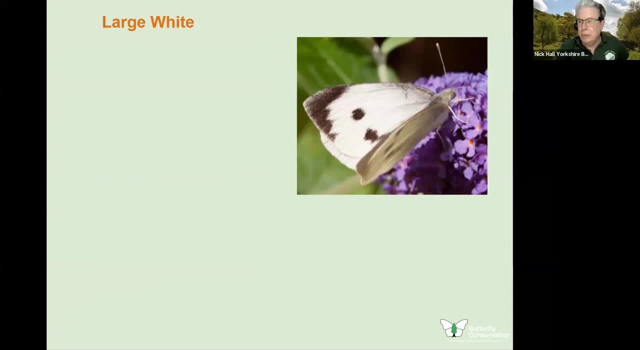 So a large white, Probably the easiest of all the whites to to determine. So it's a pest, The dreaded cabbage white butterfly. It's the largest. The main characteristic which you can use to pick it out when it's flying is it has a very purposeful directional flight. 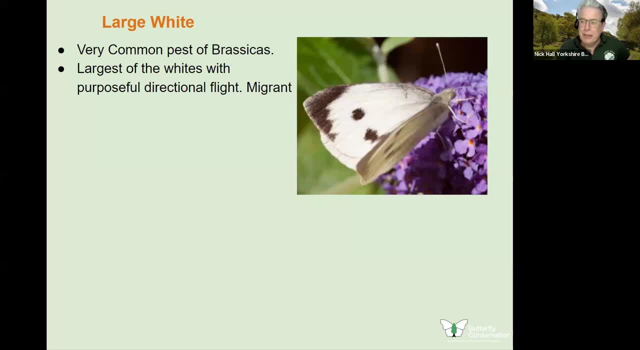 And that's important. when all the different, when we're looking at all these different species of whites, when we're covering five tonight, This one probably has the fastest, most purposeful, and it's generally flying in a particular direction. It's also a migrant and a good. 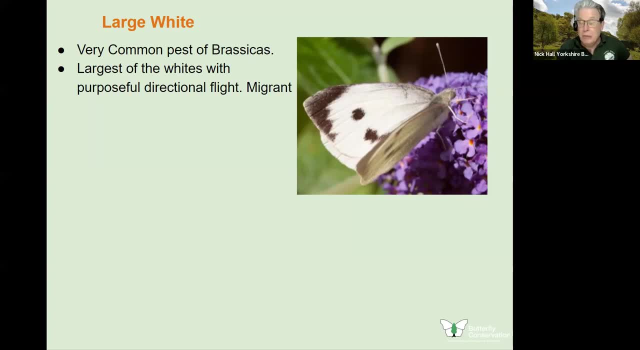 many of the specimens we see will have come from abroad. Certainly last year we had a big influx and that quite often can take you by surprise. on your transect You get a big influx and a large number of large whites appear. It has two generations. First one's in April, so it's already. 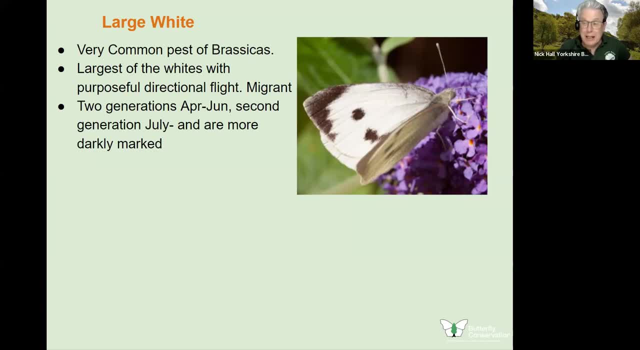 started. I haven't seen one myself yet, probably later in the in the month. It generally is the smallest of the generations. The second generation, usually bigger and it's supplemented with lots of migrants, is the July one, And the other difference is- and this happens with all the whites- is the. 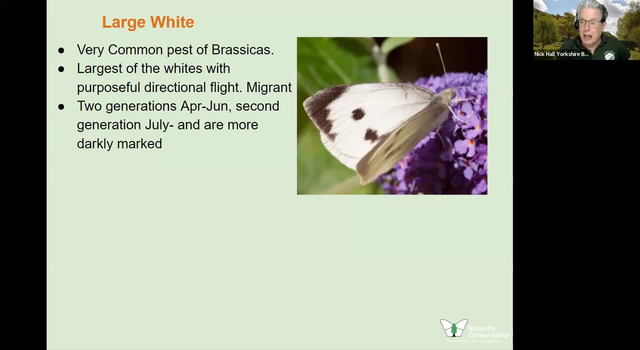 later generations are much more darkly marked, which can help you with identification. Now notice the tips, the important bits i mentioned about using the tips as a means of identification- and this is the key where it wraps around that corner and comes way down this edge here, and it's a dark black. 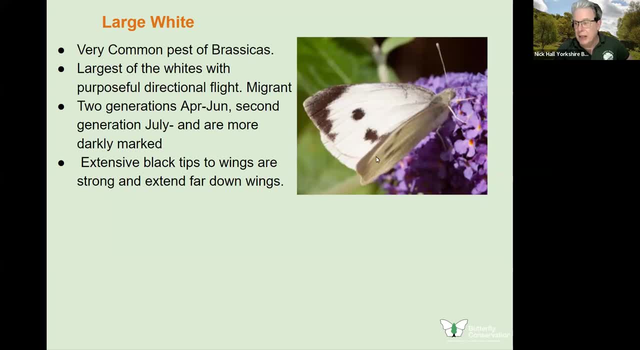 if you see that, you know it's a large white. and also if you see these large black spots, you know it's a large white. you can see these black tips when it's flying. so a good tip is: look first for that personal directional flight and then see if you can see the black. if you can see. 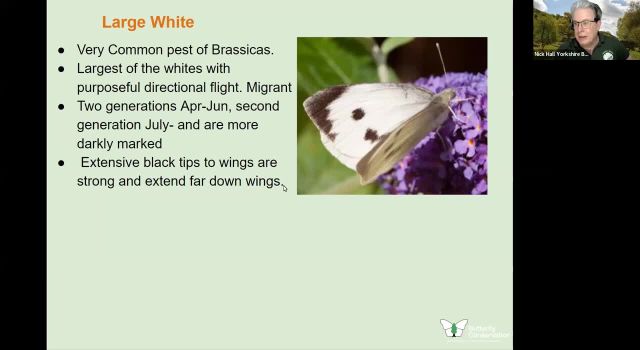 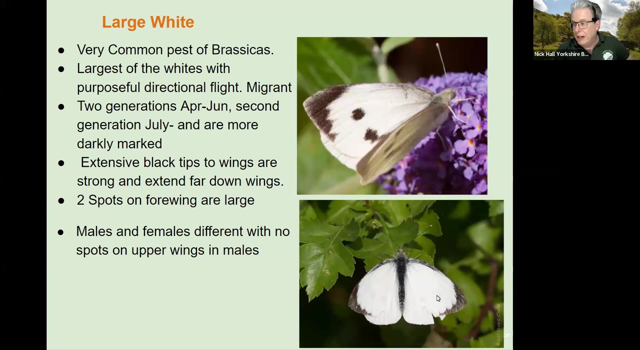 the black. you know, it's a large white. two spots on the four-way and they're large. males and females are different, at least on the four-way, the upper wings. so here's a male. no spots still got that wrap around black. but if you look very carefully there's a spot there and the spot there, but it's only on the. 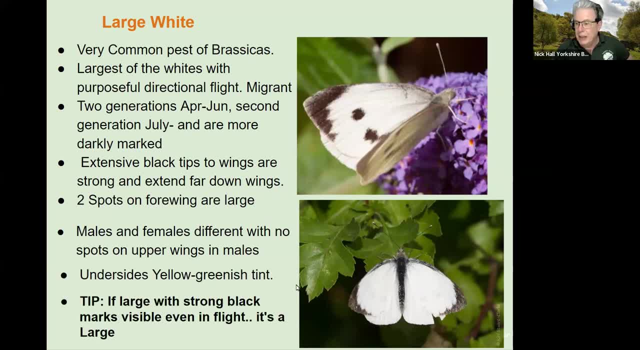 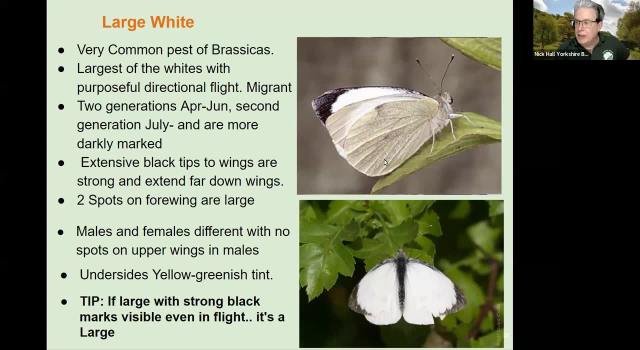 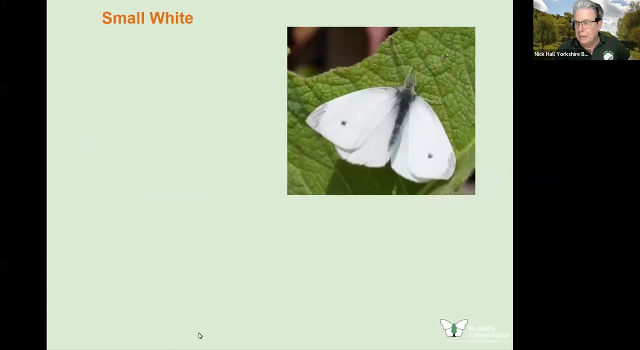 underside. and the underside is a kind of a yellowy green color which is quite different from the small white which is much more yellow. so the big tip. if it's large, the strong black marks are visible in flight. it has to be a large white, okay. moving on small white, also common pest Nebraska. but also on a. 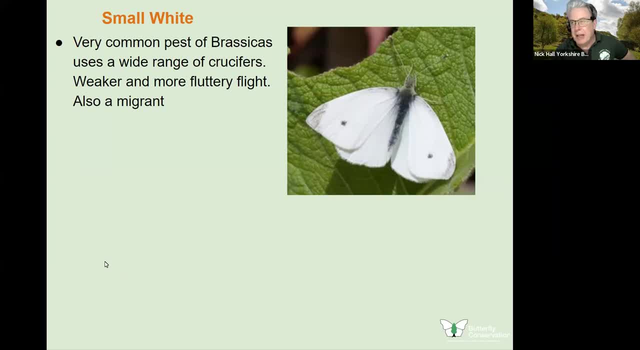 wide range of other crucifers. it has to have this: the mustard, the mustard oil, which gives it a degree of unpleasantness for a bird to eat. it's his main protection. now, compared with the large white, it's much weaker, much more fluttery flight. it's also a migrant, two generations very similar to the large white, and this is a spring generation. 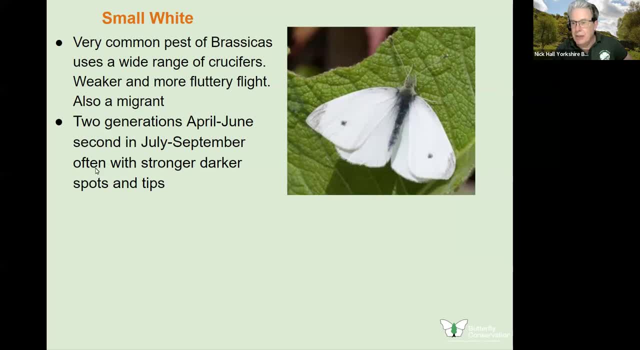 the markings are quite pale, but the July- September generation has a much stronger black color. Note the spots are much smaller. And also notice this tip. This tip does not wrap around the corner, It just goes along the top edge. It does not wrap around the edge. 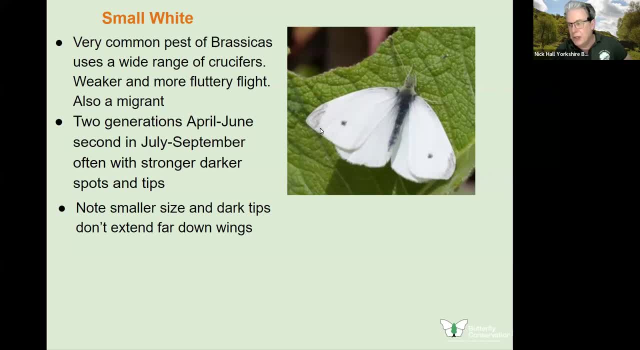 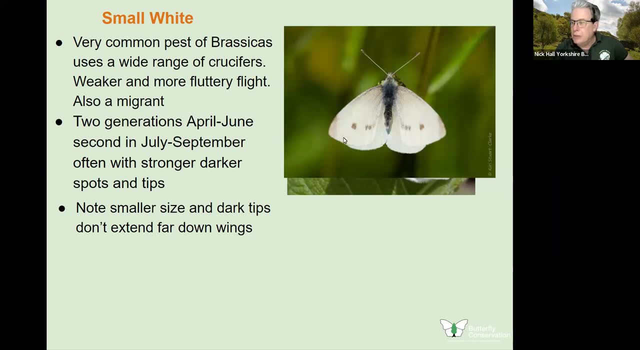 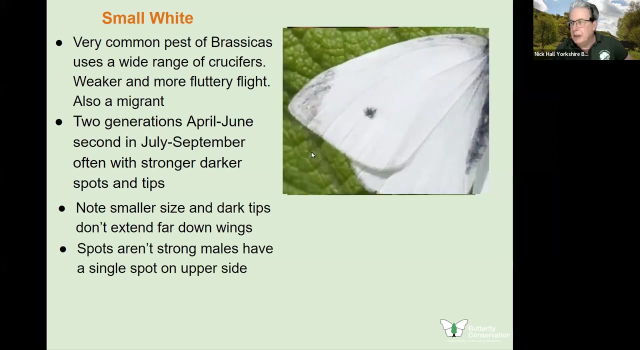 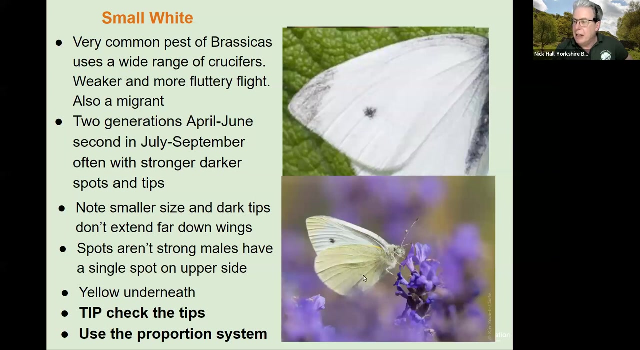 That is the main way of determining which it is. As you can see there, this is the female. You've got two spots And the dark tip there. This is a male single spot. Yeah, The underneath is much more yellowy than the large white. 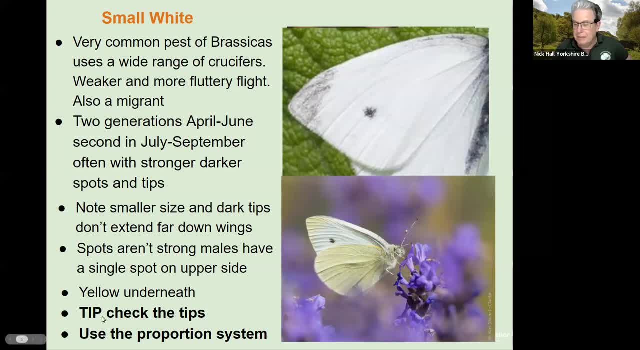 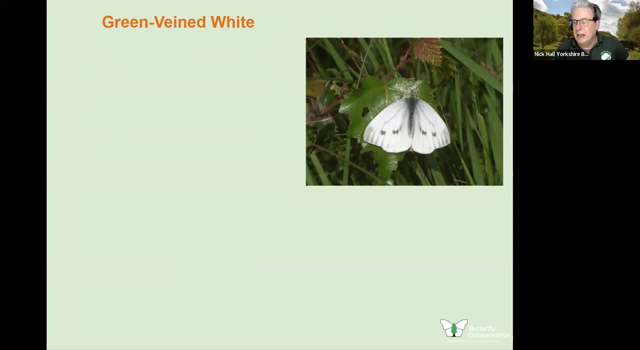 So the tip is: check your tips Now. there's also a mention here: Use the proportion system. Now the next species. we'll get into that a bit more carefully, But we're not expecting you to identify all the whites. It's impossible. 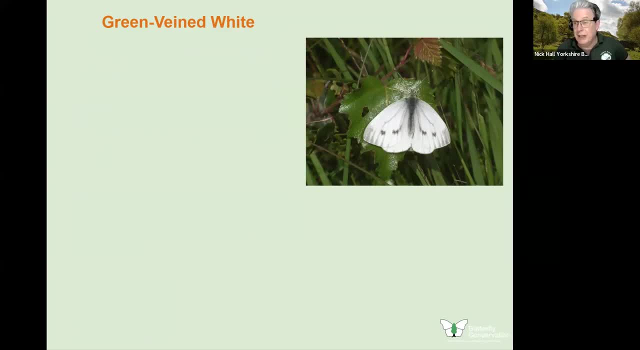 And the difference between a flying small white and a flying green, vein white is very, very small. I don't think you can determine it by just looking. You have to be lucky and find one that's landed- So we have. You have to use different systems, which I'm going to come to in a minute. 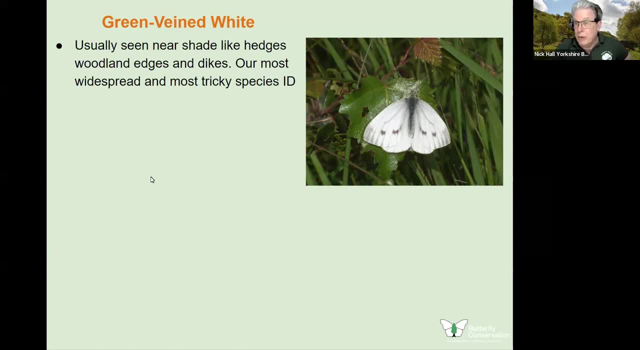 The important thing to say about the green vein white is: it's much more. It's much more. You always find it nearer shade Hedges, woodland edges, dikes. It's a damp lover. That's where it is food plant which is. 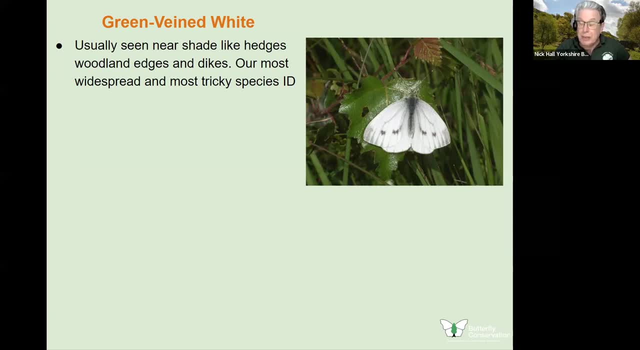 Well, it has a variety, Also brassica species, but it's most common. It's the same as the orange tip, which is the garlic mustard. It's also our most widespread And it can live up to, I think, 300 meters in altitude. 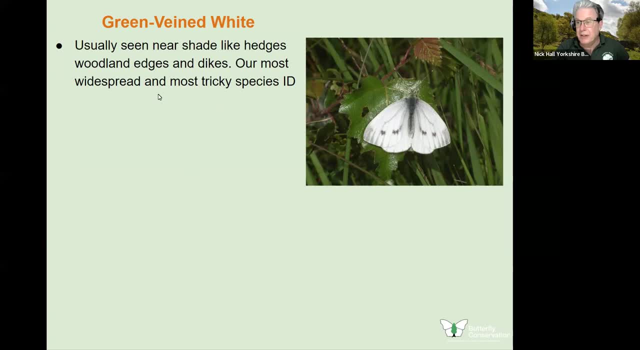 But it's also the most tricky species to identify. So let's get into it. First thing to say it's even weaker, fluttery flight, aimlessly wandering. Well, at least a small white will be going in one direction For a little while the green vein white just wanders aimlessly. 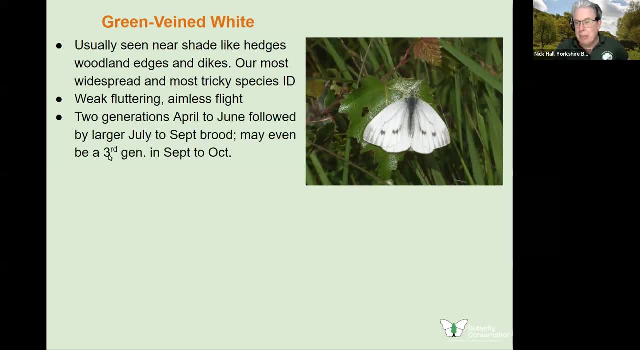 Two generations. The second generation bigger. Occasionally you get a third generation in a warm year. The later generations have stronger marks. This, I would say, is a second generation butterfly. It's much darker. The veins are very obvious. 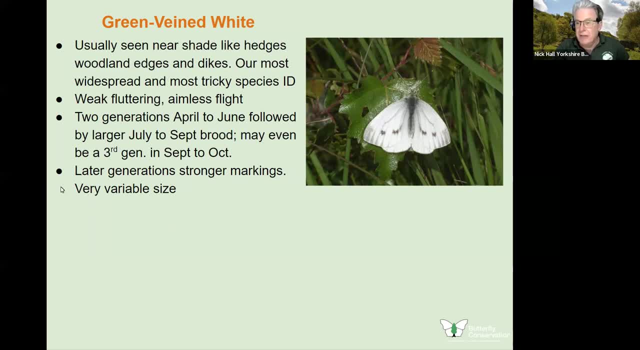 The spring generation is also very variable in size, So you get small ones and big ones, which does make it even more confusing. It has the dark tips, and the dark tips wrap around like a large white, but they are broken by white, So it's only the veins which are dark towards the edge. 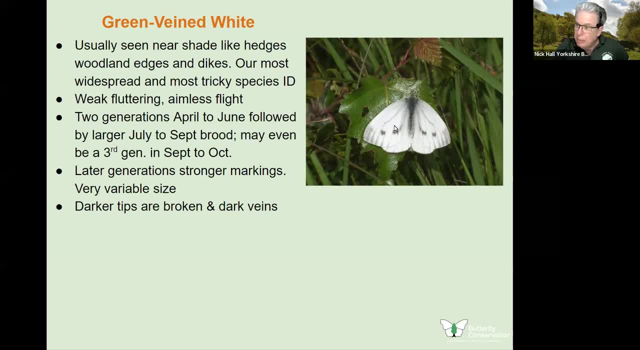 And each of the veins is tinged black. It also has the two spots, but the tip gives the story away. That probably will be your main way of telling them apart at a glance. Very difficult in flight. Like I say, you cannot really determine them in flight. 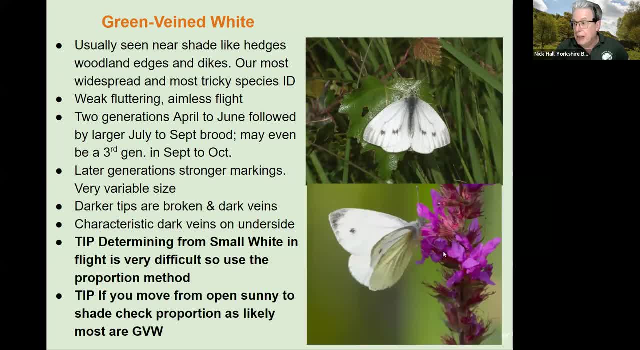 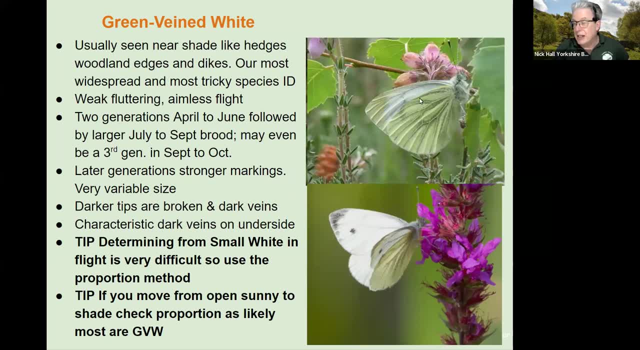 Unless, of course, it's landed. and then you see the dark veins. Now, the dark veins, The undersized veins, The undersized veins: The undersized is actually yellow, And these dark veins, if you look very closely, they're not green at all. 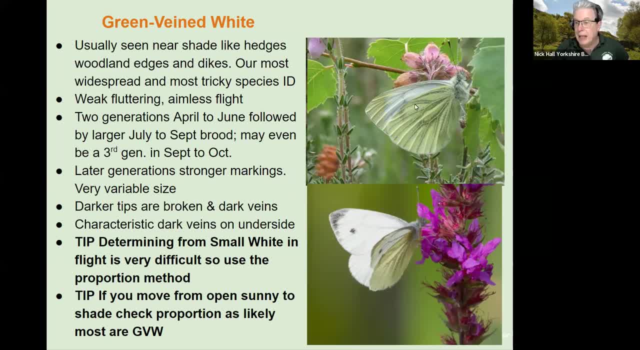 It's actually made up of a mixture of yellow and black, So if you get a chance to see the underside, you've cracked it. But that doesn't happen that very often. You're quite often relying on seeing it more in this kind of pose. 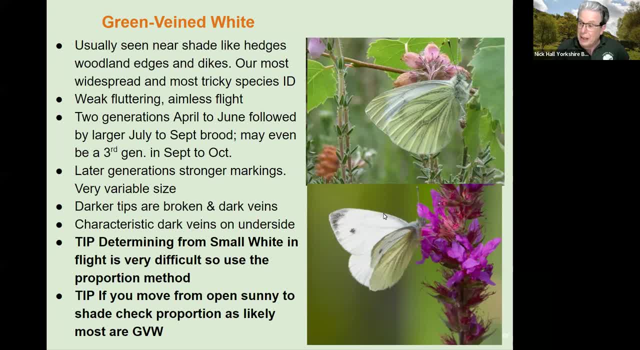 If you're lucky and it stays still long enough, And so we use the proportion. I try and practice the proportion method Now. it's very easy because as you're walking you are getting to see a number of them in a landed position. 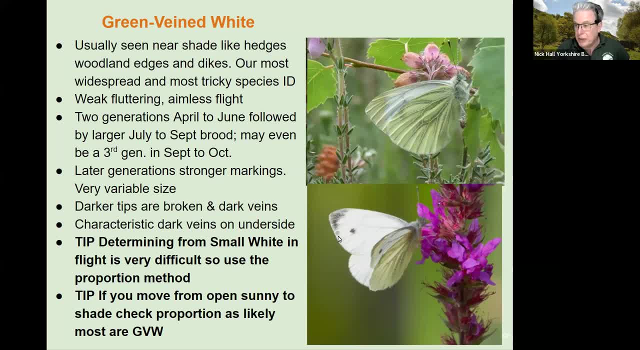 And then you can actually Do the ID that we've just described. While you're doing that, just make a note in your mind what the proportion of each is. So it might be 50- 50.. It might be 25- 75.. 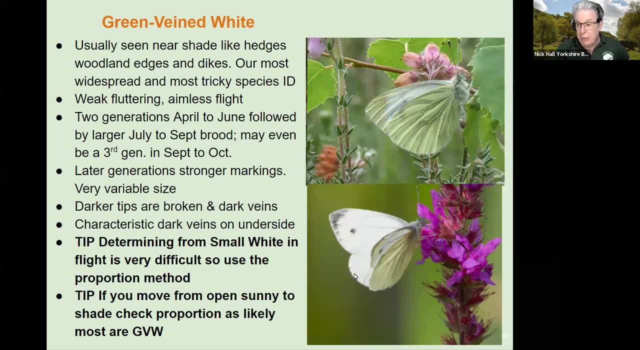 It might even be a hundred percent. An example would be when you move from open sunny into shade you need to check your proportions because likely as you go into shade most of them are going to be green, vein whites. So the proportion method works great until the conditions change. 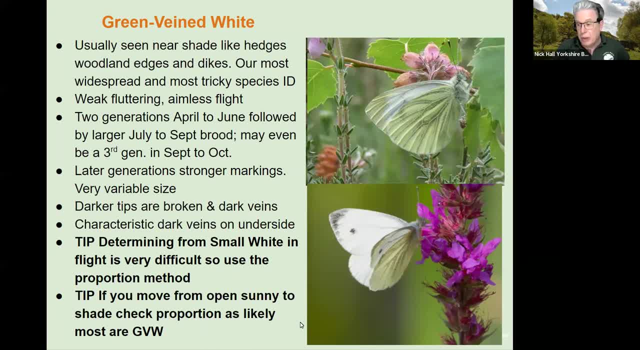 Okay, you need to check that every time you walk and you need to check it as you're going through your sections, just to make sure that those proportions are not changing. So the next white that flies past you, you can tell what it's. you separate out the large whites. 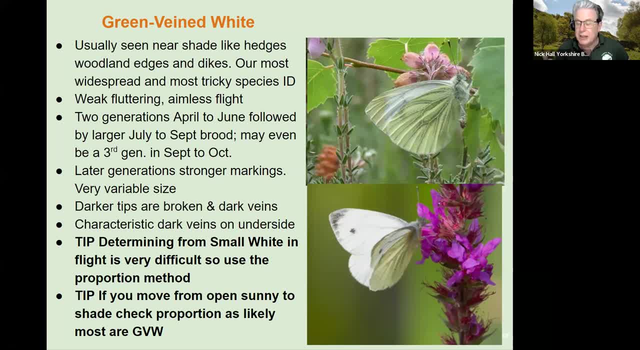 And the brimstones you lend left with the small whites and the green vein whites, And then you do: if it's 50, 50, you do one small white, one green white, one small white, one green vein white. is impossible to do any other method. 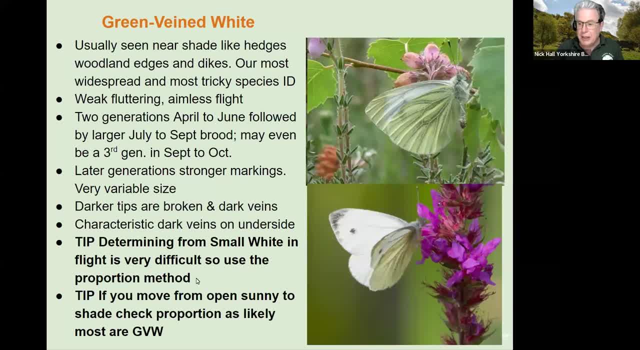 And that is the most accurate way that you can do it, to calibrate your head, as it were, Because that's the business we're in. We're in the business of recording everything. It's important that we, We record, edit everything, but we're making that best guess. 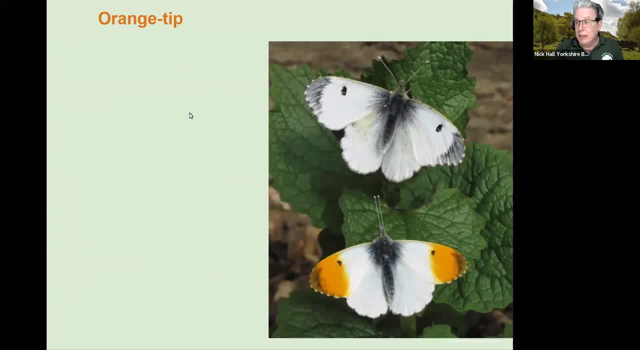 Just to make life a little bit more complicated than you have. the orange tip, which of course the female Is a male, Is characteristic tips, But of course it has its habits and it's very much prefers damp areas where it's food plant garlic mustard grows. 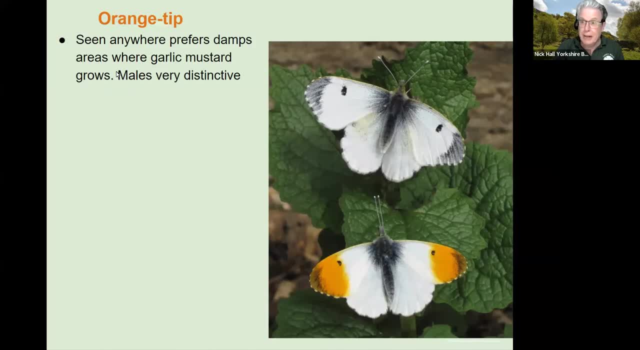 And you see the more In a woodland Areas than you will in open areas. Males are very distinctive. They wander a great deal Trying to find females, But the distinguishing mark which I'll point out now is the male has a very small black spot just on the edge of the orange. 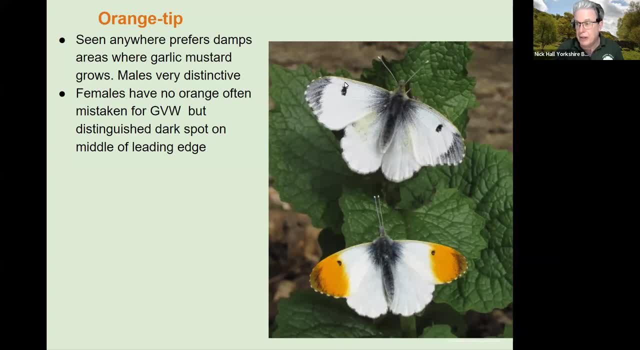 The female has a pretty large and it's always dark, It's always black And it's near that top edge, in roughly in the middle. You also notice that the wings are different shape from the whites that we've just been looking at. the wingtips are round. 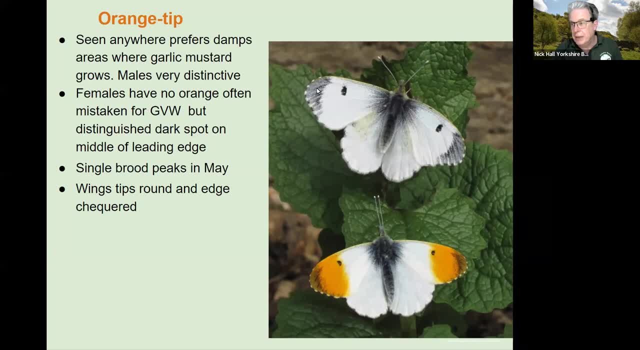 And they're also checkered, But they are quite a deep shade of Black, And that differentiates it from the mandarin will, And that differentiates it from the mandarin will, And that differentiates it from the mandarin will. 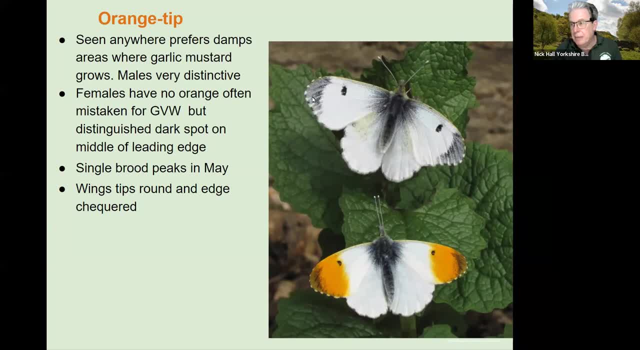 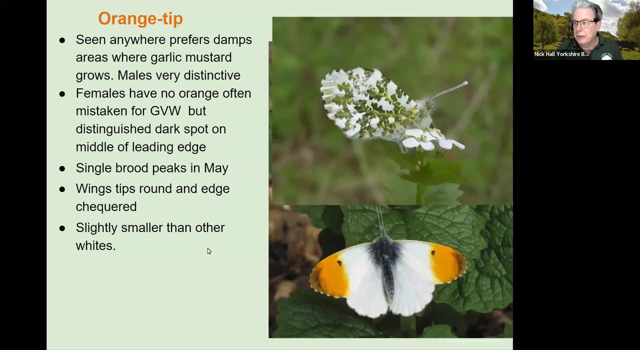 from the green vein white, where that would be much more diffuse. it would be broken, broken up and you have that characteristic black spot and the checkerboard. it's also slightly smaller than all the other whites, so it's the smallest of our whites and, of course, what we all enjoy seeing is that wonderful patterning on the back. 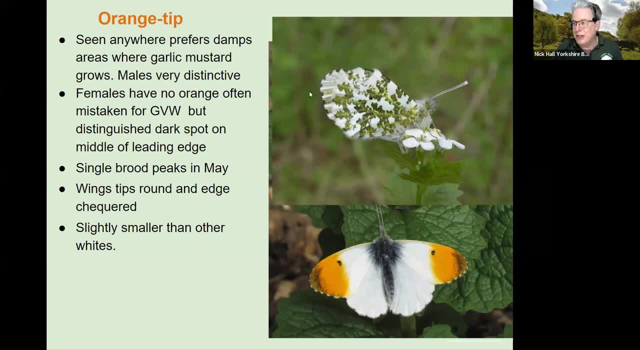 isn't it just absolutely gorgeous when you just stop for a second and just admire that intricacy and when you see it sat on a cow parsley, you begin to realize that that is an exact mimic of a cow, partially flower. it's a cracking mimic. and if you also look really closely because it's a lady- 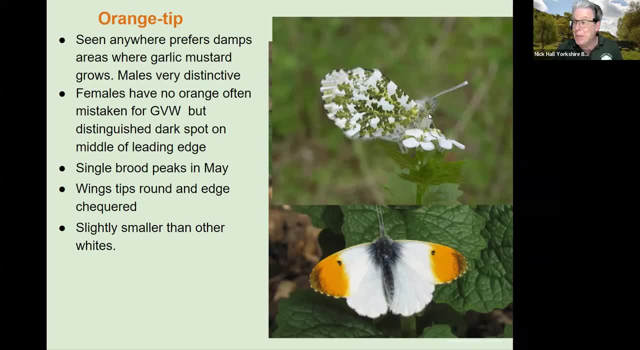 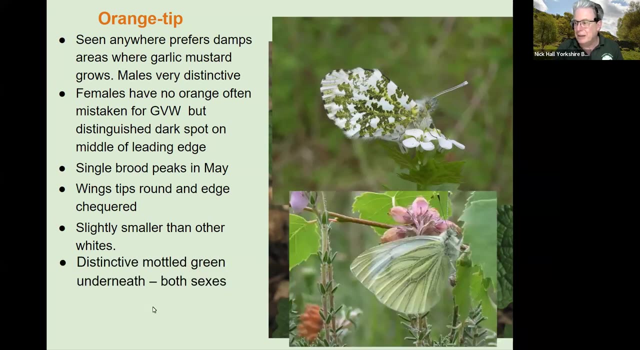 she has yellow eyeliner. you need a really good close-up shot, but it's absolutely gorgeous. again, this color is not green, it's actually yellow and black. that's the same for both sexes. and look at the difference between the green vein white and the. it's not difficult to get those two separated. i think. quite different patterning. 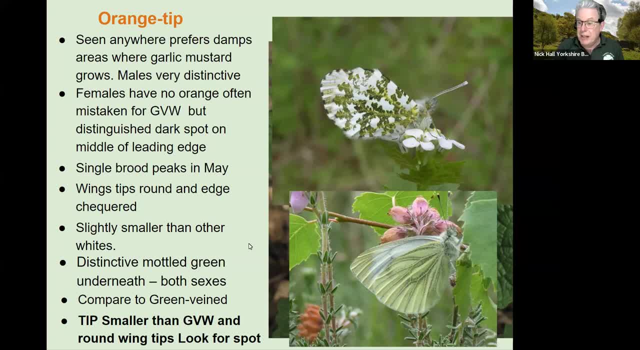 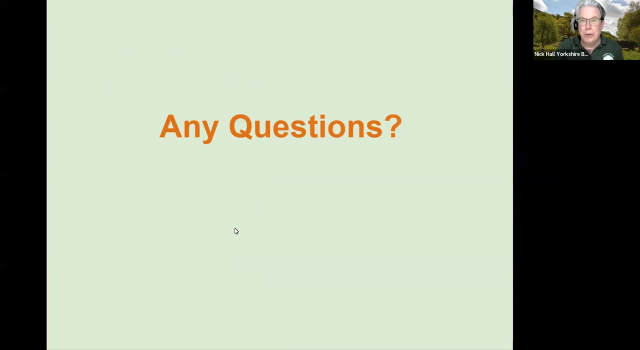 so the tip is. it's smaller than the green vein, white round wing tips- and look for that spot, that characteristic spot in the middle of the female's um uh forewing. that is absolutely diagnostic. so we're just going to pause now and if you have any questions, please, 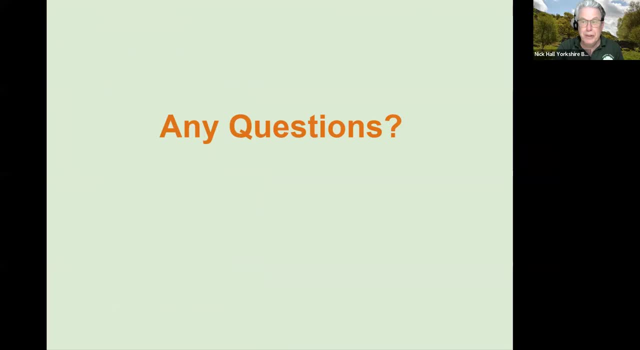 unmute and i will take questions, otherwise we'll move straight on. so nothing in the um the chat box at the moment, nick, okay, good, don't, don't um, don't be afraid to ask and stop me. that was a pretty um deep dive into into whites, but 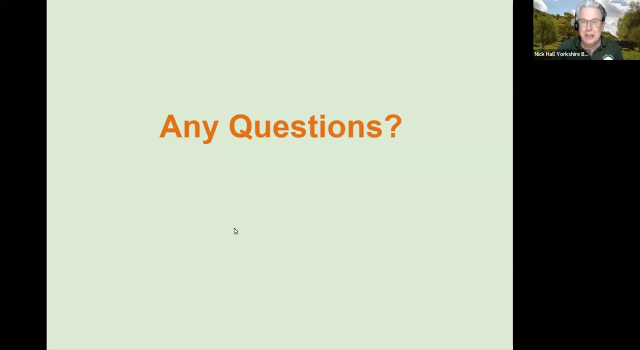 from our last meeting. that was the one that people really wanted to get their heads around is how. the way you do whites. i hope i've managed to answer some of the questions. okay, we're going to move on. if there's no questions, i? i have a question actually. okay, stella, that's. 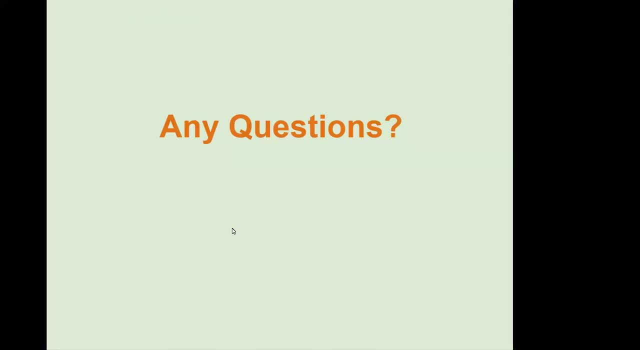 stella. um, you're talking about the proportion method. yes, did i understand correctly that if you see something that you think could be a small white or a green veined white, yeah you just that's a small white, and then the next one's the green bay. so you just so. if you say 10, you say five. 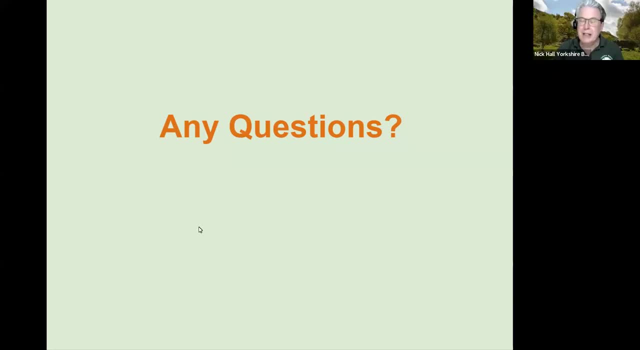 was one and five was the other. roughly- um, it's all, all matter of of. roughly i do uh. 0, 25, 50, 75 is my kind of uh proportions and i base that number basically on what i'm seeing, so the ones that are actually settled, that i can actually determine what they are by the methods we've described. 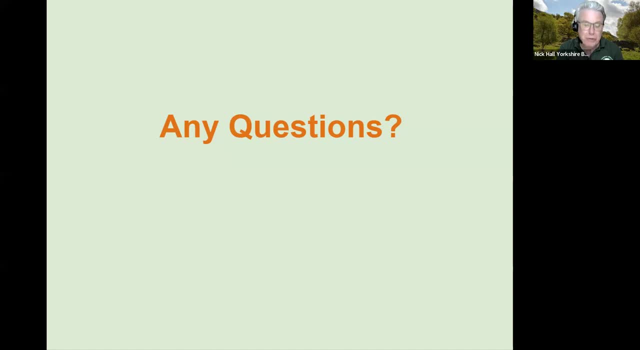 after i've seen four or five, i know roughly what the proportion is in that section. so if i get in 25 percent, that'll be and, uh, in favor of, um, green vein whites, which would be typical of a shady area. um then it would be. three of them will be green vein white. the next one would be a small white. 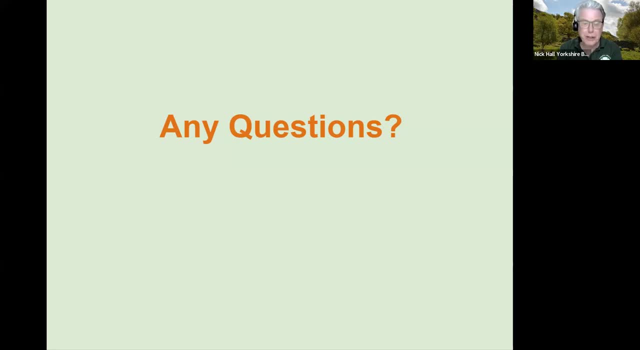 small, small white, and i would keep that proportion, unless, of course, i'm only using it as the way i'm going to use it for the ones that i can't identify. so the ones that i cannot firmly identify, not using it for every single insect, only for the ones that i can't identify, they're just going too fast. 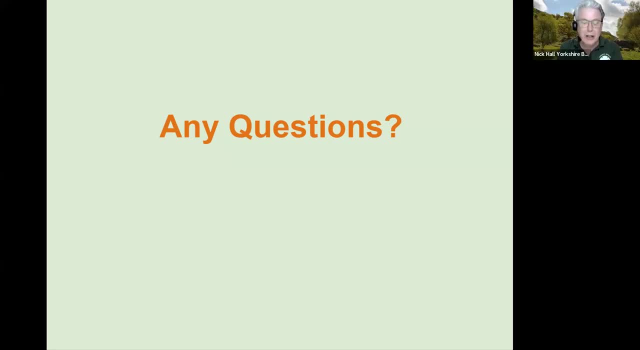 don't settle, etc. so i only apply the proportions to the ones that i can't definitely identify. i'm sorry. no, i think i missed. i should have made that clearer, stella, so you're right to pull me up. uh, very clearly. thank you for bringing it up. no, thanks for explaining, because i'm very new to this. 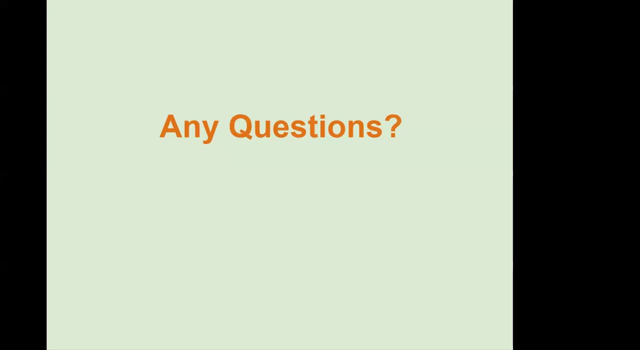 so i just needed to check that i had got the understanding right. okay, it's quite a quite a concept to get your head around. to begin with, i think um- and it's the first time i've talked about it on any of these- um, for a lot, of, a lot of people it's kind of automatic. well, i didn't. 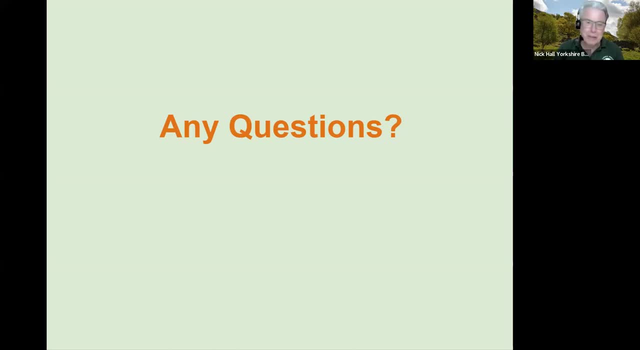 identify. i'm seeing 50, 50. it must be in a small white, must be. people kind of do it automatically in their head and it should be. it should be your almost automatic in your head, without thinking about it. okay, i'm sure what i would do, and what a lot of people do, is actually at this time of the 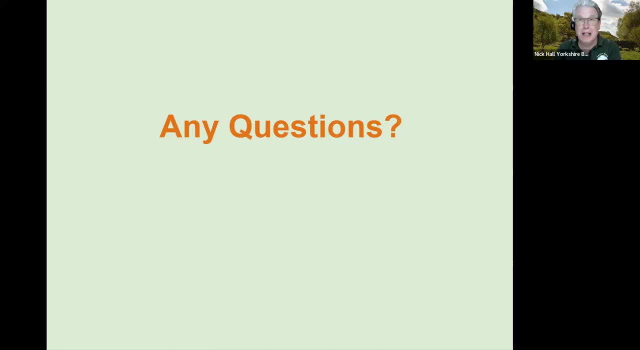 year as the first orange tips come out. you've got green vein whites and you've got orange tips. can you spot the difference between the orange tip- female- and the green vein whites? there'll be small whites along in a few more, another week or so, and then it'll be a good chance to get out. 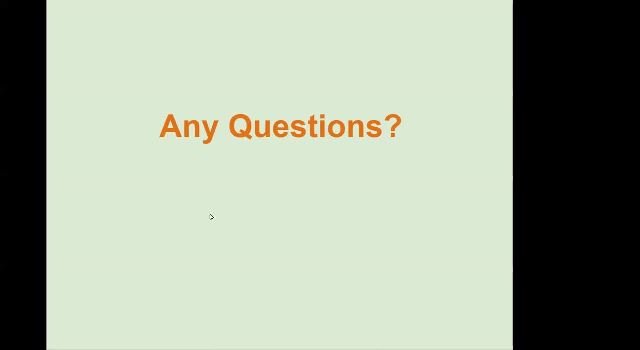 the garden actually practice those skills. so you make, you have a look at it and make your best guess and then you check, then you chase it down and actually do an id. so you think it might be 50, 50. you check two or three and just figure out. was i actually correct? do i need to correct, correct what i'm? 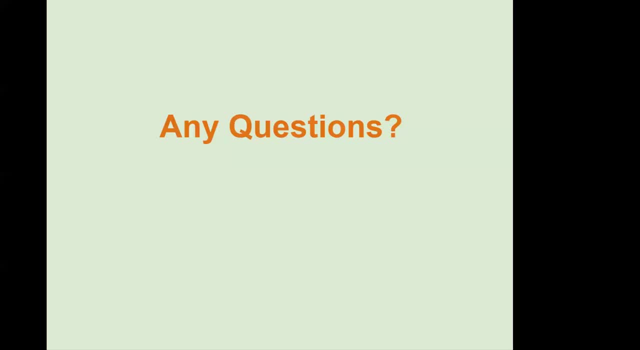 thinking: all right, yes, you can't be a bit of practice out in the garden? in my opinion, if, if you're new, these are kind of. it's the kind of skills you you learn in the first month, stella, and you do learn them, you do learn them really. 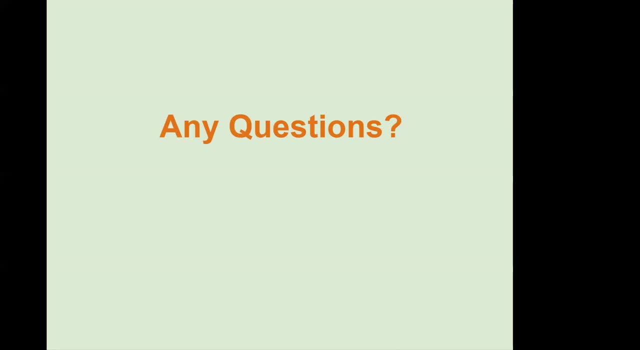 quickly. so, okay, don't worry, it will become automatic, right? thank you very much. okay, i'll move on. yeah, i'd add there that you, you tend to you start the season where everything's gone up your head because you've had, you've had four months off, and then you get your eye in and 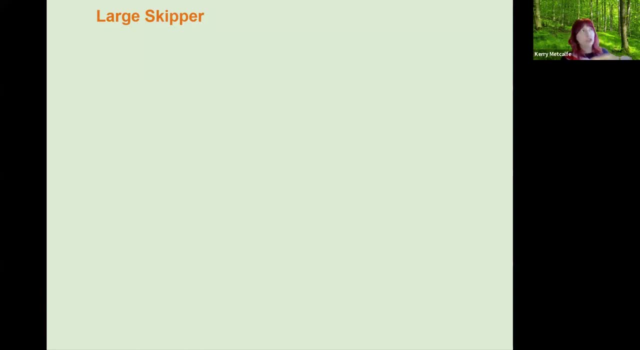 everything gets just a little bit easier. and then you will find also that on your own transit you get to know the um, the places where you're going to see these things, and what you're likely to see in specific areas as well, just as you keep doing it, but particularly as the season goes on and and 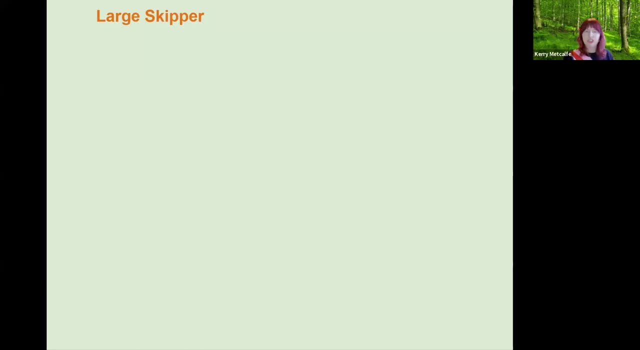 you start to see them and then they build. and yeah, it does just come with experience, i think sometimes- and we're always learning- you can have as much experience as you like, but we're still always learning. i learned a lot just just preparing this uh presentation. i have to be honest. 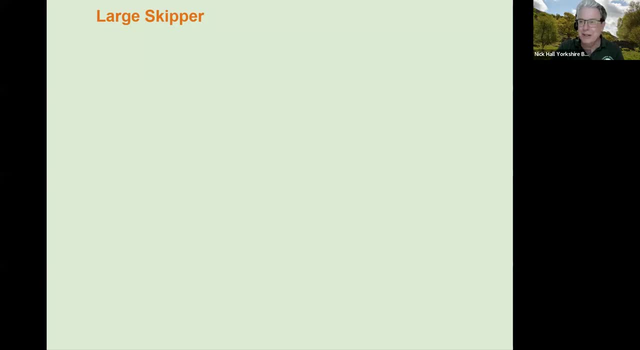 i'm gonna hand over to you now, carrie, to do, uh, do the, the dreaded skippers, because those were the other family which people had the most difficulty with over to you. yeah, i've taken these on because they were my nemesis for quite a bit. i should add in here as: 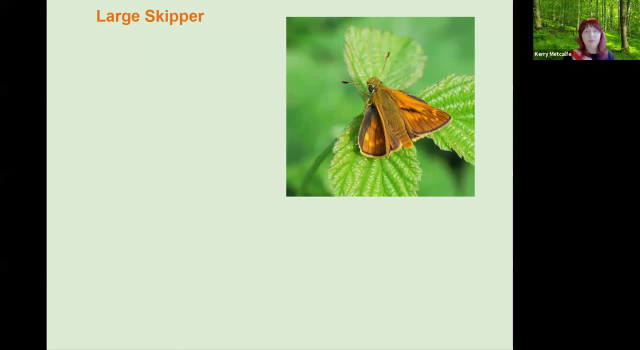 well that nairi says in the chat. their binoculars are really handy, um, and they, they absolutely are, as well as a camera, if you can have one. so large skippers, um, so like small skippers, they um tend to tend to be in discrete colonies that are fairly small, so you'll find that they'll have. 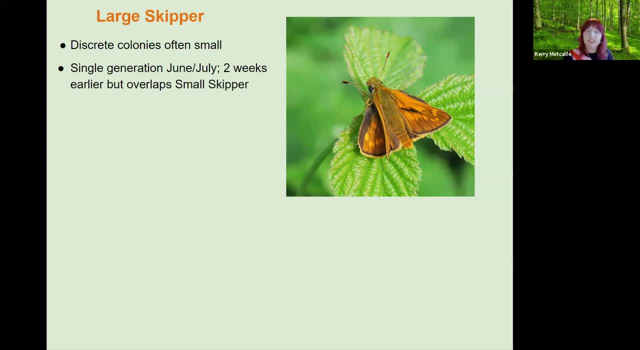 references for particular areas on your transect. so for instance in mine um they tend to favor down at the bottom of the bank um in the longer um damper grasses and on my transect large skippers i will generally see in the brumbly areas um where they're nectar on the flowers and small. 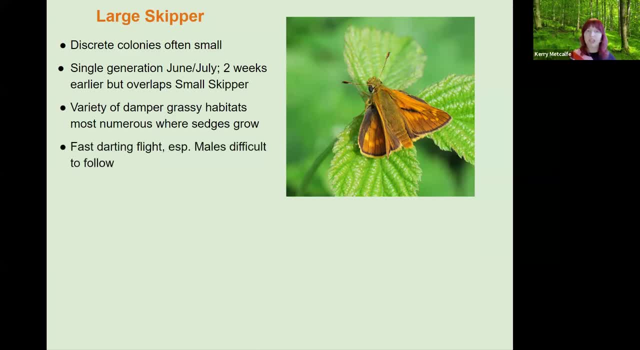 skippers i'll see in other places, so you can start to build up an idea, as i was saying, of where you might see these species within your transect. um, large skippers: i generally see them when they're leaping off some sort of vegetation just as you're walking by. but 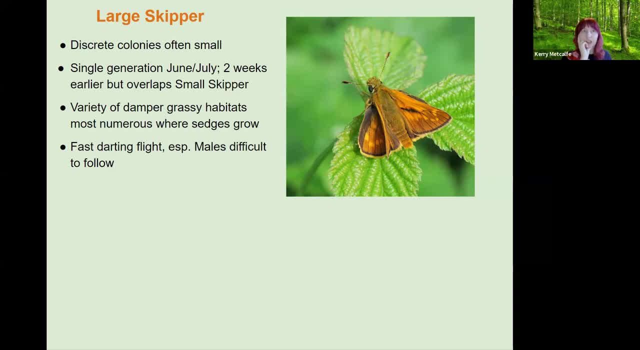 they're extremely fast, um, really hard to keep track of. so the leap off and you'll spend quite a bit of time looking around thinking what was that and where did it go? um, and usually the answer is no idea. um, but they, they tend to be easy to differentiate from. um, the smaller skippers. 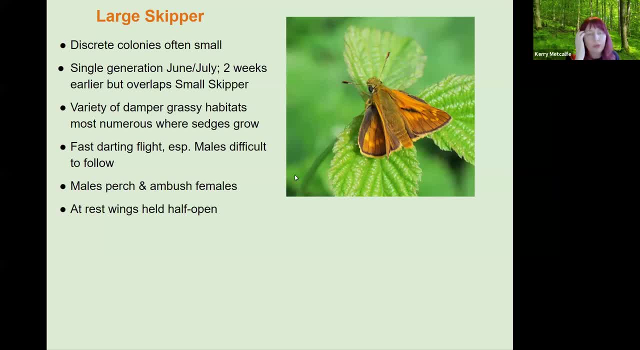 because they have this nick. could you just hover over the um, the wings? they have this checkered marking on the wings, um, and that's generally what i'm using to try and differentiate as well as the way that they fly um. so that's great. thank you, nick um. 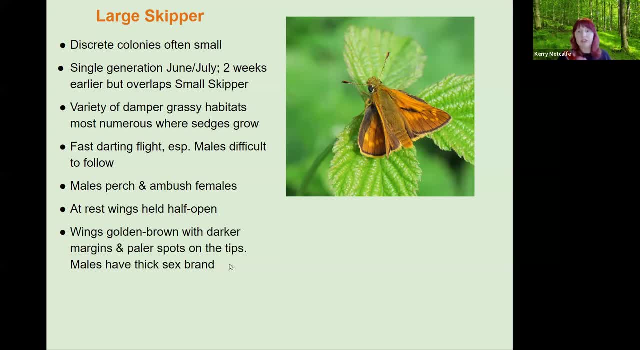 so large skippers will emerge earlier in the year, so you're expecting them in june, so you have a bit of time. you've got about two weeks before the small skippers then turn up, so it's a great opportunity to see them in the spring and then you can see them in the fall. 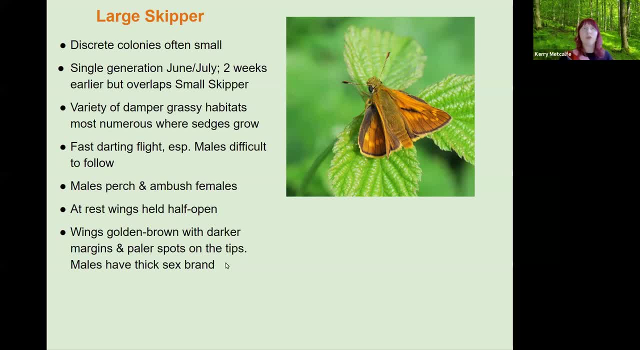 so it's a great opportunity for you to spend a bit of time familiarizing yourself with with their, their jizz, their the way that they behave and the way that they fly, because it is slightly different from from the small skippers which i i find still dart about, but it's just. i would 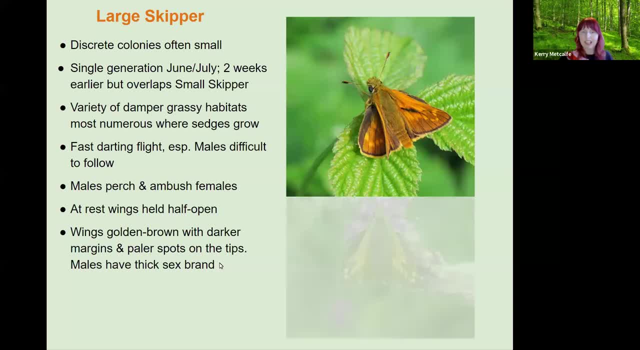 describe it as more gentle. um, i think, yeah, just a gentler. so they'll leap about and dart from from vegetation to vegetation, but it tends to be more localized. um, so you can keep track of them a lot easier. um, yeah, there's a great example at the bottom of the checkered pattern that you see on. 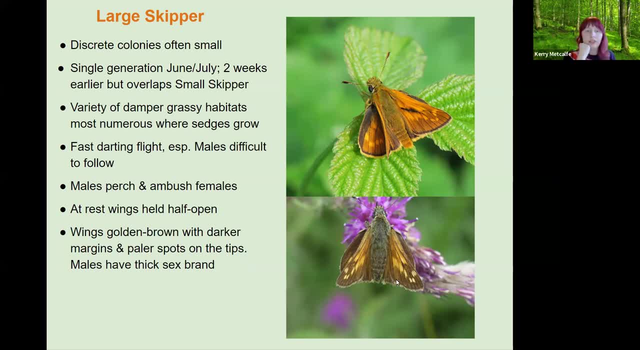 the top of the wing and in in the- uh, small and essex skippers. it's just a plain wing and i think that's the easiest way to tell them apart. if if you can do that in conjunction with the flight, i would really recommend, if you can, um taking a camera out. this is the easiest way i've figured. 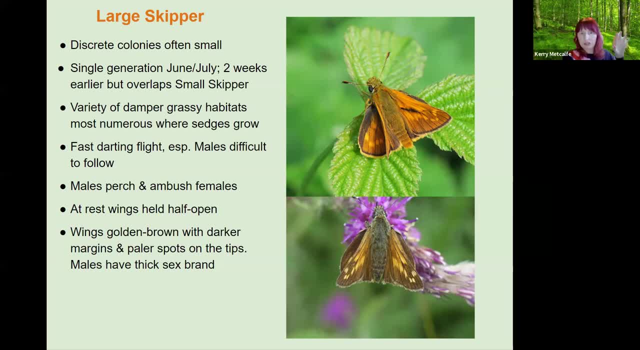 out to to really learn the difference between large and small skippers, and i think that's a and how to just really nail um that identification. you can also do it by antennae, um, so in the large skipper they're pointed where, in the small skipper they're, they're rounded um, but you're. 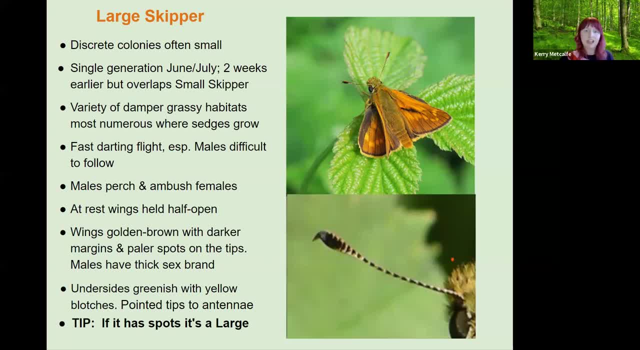 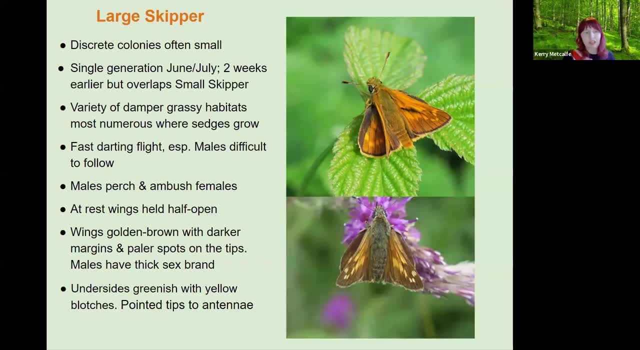 needing to get you. you're either going to have to get very close- and it's fairly impossible to do that- or, um, yeah, you're going to have to take a load of pictures. um, that's, that's generally the method i've used, and let me just check the chat. 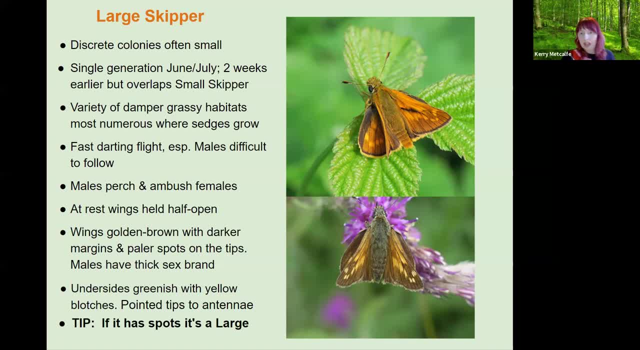 um, yeah, definitely take a field guide, the uh nhbs. one's really good. um, it's got three, three or four pages that's filled out. um, i have mine with me all the time, really helpful for if you spot something but you're not quite sure. um, and loads of pictures. thank you, that's helpful. you're welcome. 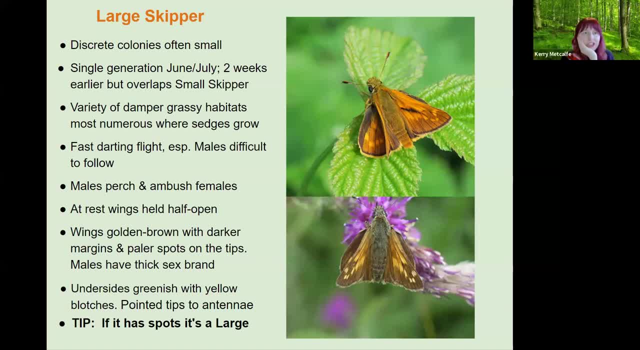 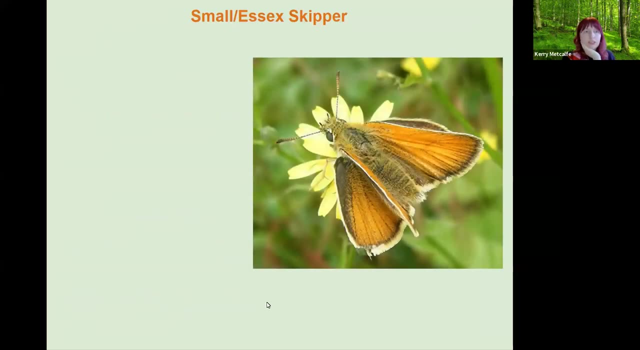 um, so i'm jumping about a bit, um, trying to just, uh, um, get get a handle on the differences between the two. so, nick, can we move on to small skipper please? so small and essex, um, we tend to group together. i don't have a six on my transect, so i'm, it's not. 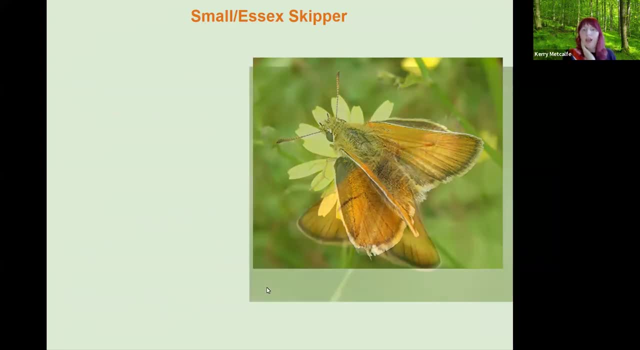 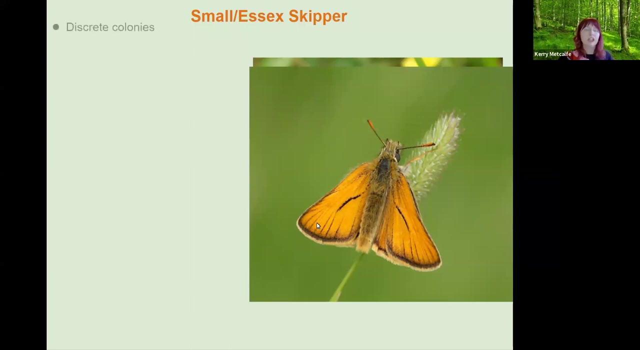 a species i'm particularly familiar with. um, so again, you'll see from this, uh, that that really blank in patterns, again very bright yellow and the size between the large and small and essex skippers is fairly negligible, even though they're called small and large. they like to keep us on our toes and confuse things, but it's really that color that you're. 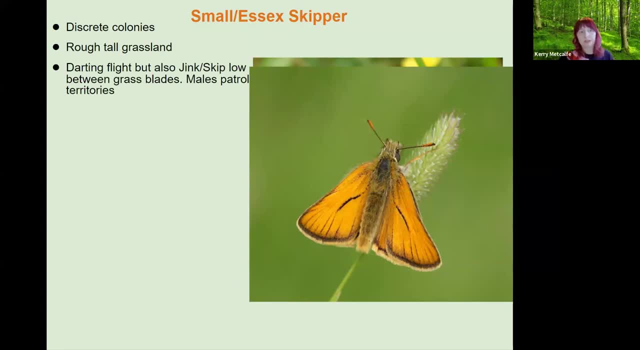 going to notice if you can get up close and the the flight pattern. so, as it says there they like the rough tall grassland as well and also exist in discrete colonies and again you'll find that the flight is darting and they skip about. but it's just, as i said, slightly gentler, so a little. 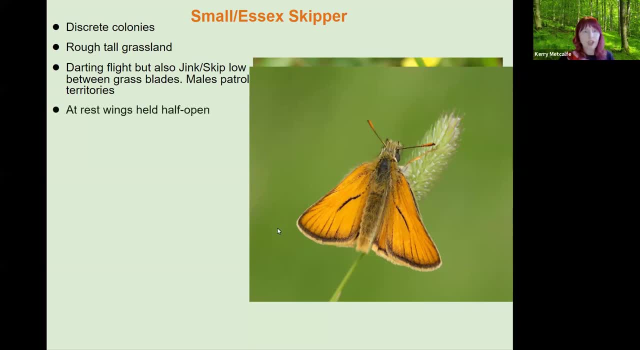 bit easier to track and, like the large skipper, they also keep their wings half open at rest. and can we just skip on a bit, nick? yeah, so, so the so you'll. you'll see the large skipper, first in june and then two weeks after. 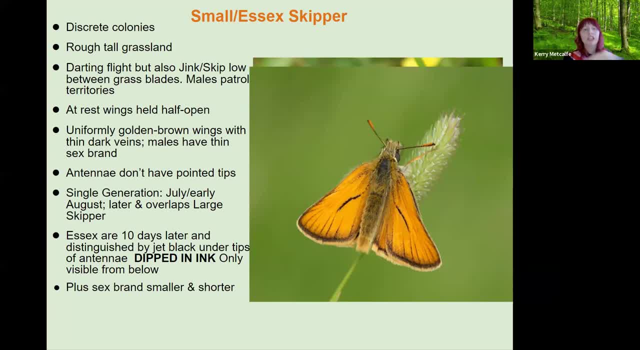 that you'll start to see the small skippers and then 10 days after that, roughly, if you have a essex skippers, you'll start to see the small skippers and then 10 days after that you'll see them. then, um, i think the only real way to tell between the essex and the small skipper is using 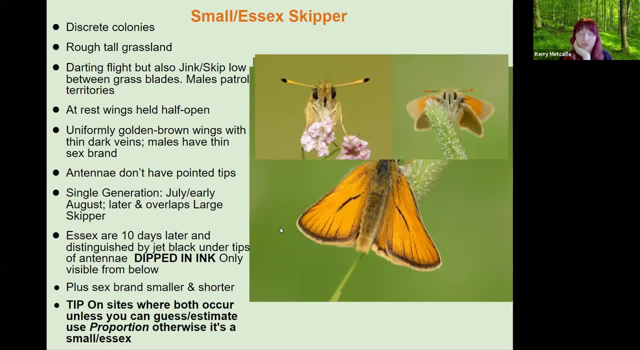 the antennae. so in and you, you're absolutely going to need a camera or binoculars for that and, um, yeah, really cooperative butterflies, um, so you're looking for in in the essex skipper, you'll see, nick's just got his um cursor on it there. their antennae look like they've been dipped in. 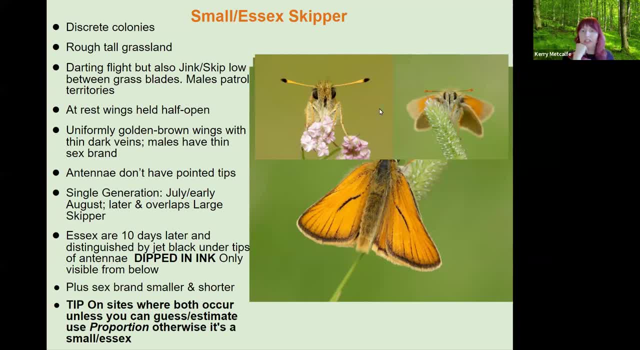 paint or ink, and so it's a very black tip, and then you'll see the small skipper and then the orange tip, whereas in the um small skipper it's orange tipped. so those two pictures are quite, quite good at telling, giving you that distinction. they also do have these sex or scent brands in the 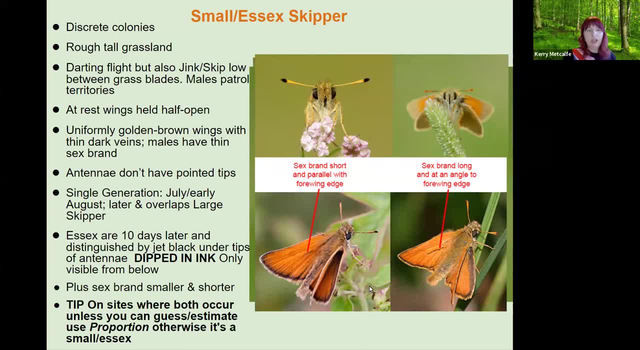 large skipper they're quite um quite large and chunky, and in the small skipper they're fairly slim and quite short, and in essex they're slim again but angled and quite long. so, as nick's put here on site, i'm going to show you a picture of a small skipper and i'm going to show you a picture of 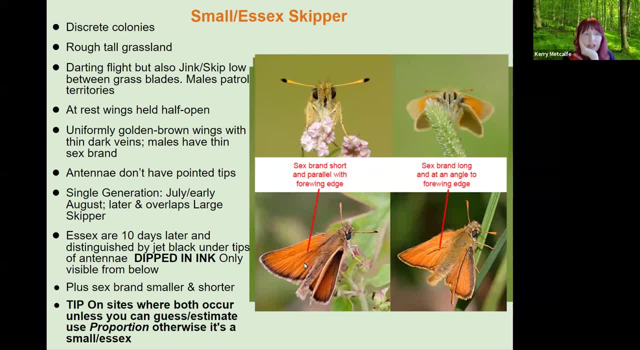 a large skipper. it's where you have large, small and essex. uh, the easiest way to tell them apart is: if is, is that a large skipper will have the, the checkered and upper wing, whereas small and essex won't? and if you're really not sure, use nick's um suggestion for for proportions. 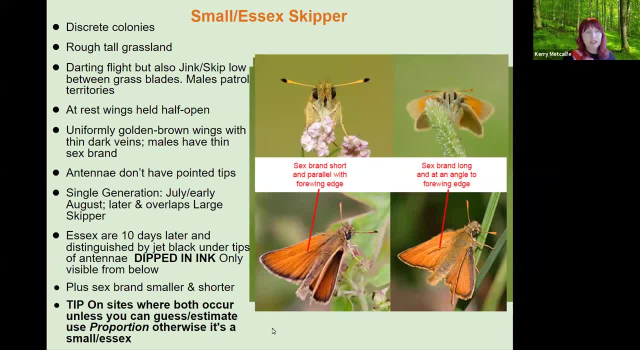 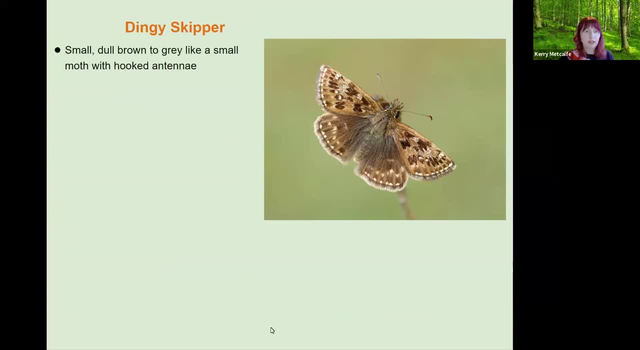 yeah, so that was a quick run through that. any questions on the small and large skippers? i think these are ones that that you really get your eye- and it took me three years to to try and figure them out of- of just taking photographs and getting frustrated and sending nick emails saying 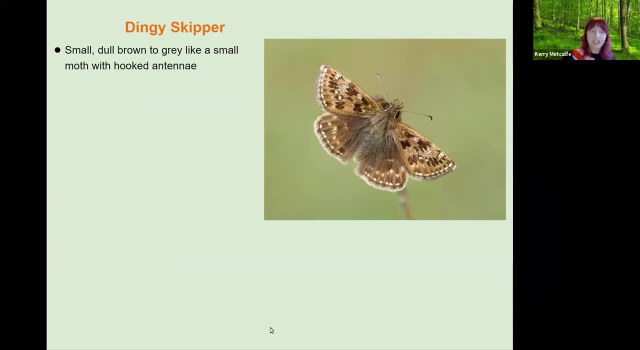 what's this um, but you do just start to get a feel for the way that they behave, um in particular. so it's a really good if you have them to, to try and and just get a handle on how the large skippers behave right at the start of the season. 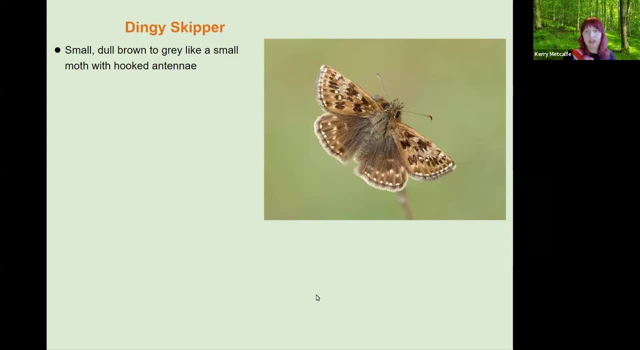 right, so we'll have a look at dingy skipper. um, dingy skippers are a bit of a speciality of of the, the transect that i manage at fordon. um, so i really like them. i think a lot of people think they're a bit dull and brown and boring, but i think they're really pretty, um, and and i really 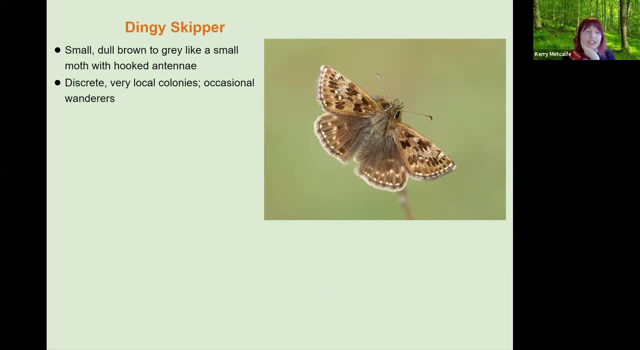 like to champion them. so yeah, as nick's put here, small, dull, brown to gray, um and a bit moth like. so they also live in in discrete colonies. so they're really pretty and they're really pretty. so again, in your transect you might find that they like to appear in particular areas i've got. 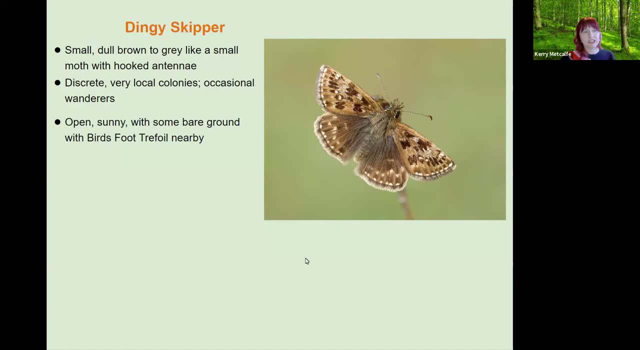 particular areas in mind that where i'm fairly guaranteed to see them. so they're. they're um very much in favor of open sunny areas with a bit of bare ground and where they can bask in the sunshine. they nectar on birdsfoot treffles, so you'll find them around anywhere that has that. 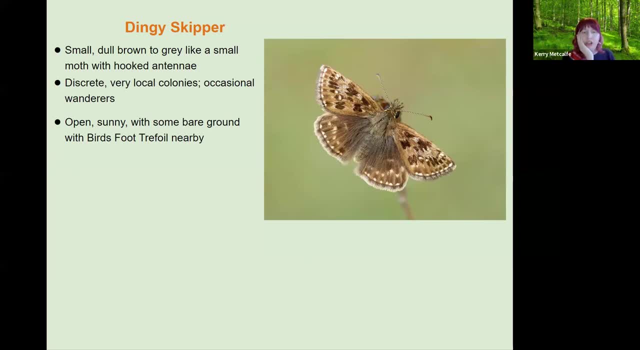 as well in any of the other treffles and and i think they're particularly like yellow plants, so i often see them lecturing on dandelions and and celandines and things like that. uh, in terms of flight they're they're small and quite fluttery, but they're quite quick, so you can. 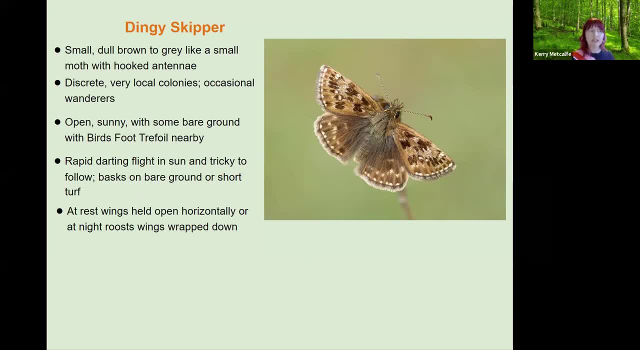 lose them quite easily. um, i always find that they're quite um cooperative in that they'll they'll often flutter around and then they'll settle. so it's sometimes quite easy to get right up to them and and have a look for an id, particularly again if you've got a camera or a pair of binoculars. 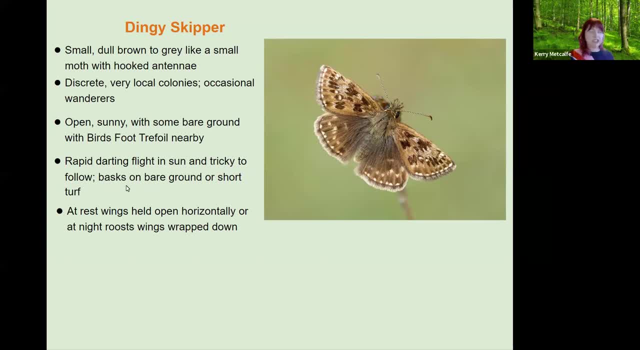 and i've never seen it. but so in the daytime they'll rest with the wings out, but on the night time they'll sit on a blade of grass, like like this picture at the top, and wrap their wings around the top and it's like quite an impressive little feat. so just to sing single generation. so 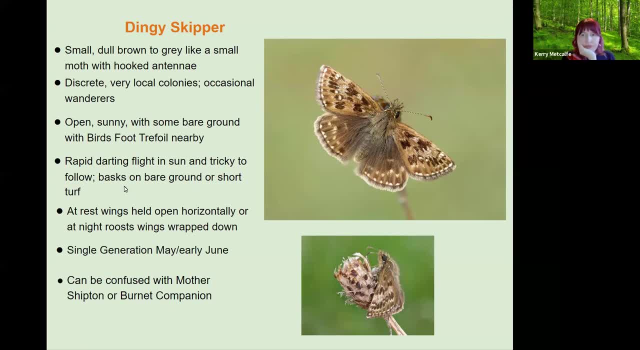 you'll start to see them in may time and early june and then, in terms of what they can be confused with, there's mothershipton and burnut companion. so mothershipton is a legwings species and they're mostly um, they're often mushrooms and they're mostly matte, and they're also some occasionally. 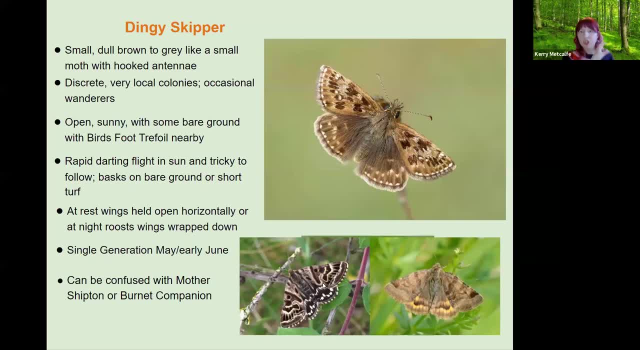 shipton, you can distinguish, because they have that very distinct, quite contrasting wing pattern that looks a bit like a witch's face and i find mother shipton tend to say no, thanks very much, fly off and sit and flutter in grass that you, you just can't get to and they're quite hard to to. 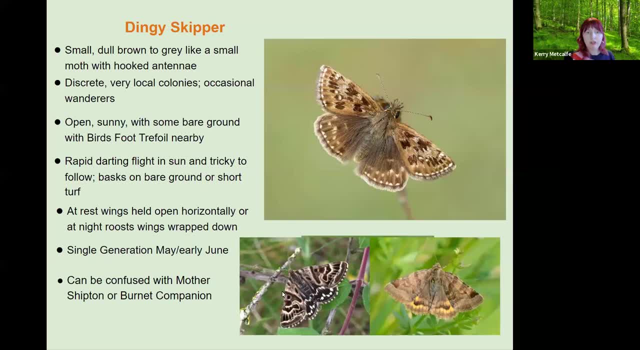 to really, um, compare really. and then the burnet companion has that yellow part of the underwing. so again, you should be able to differentiate. and and they have a similar upper wing pattern, but they're just a bit more drab than the dingy skipper. 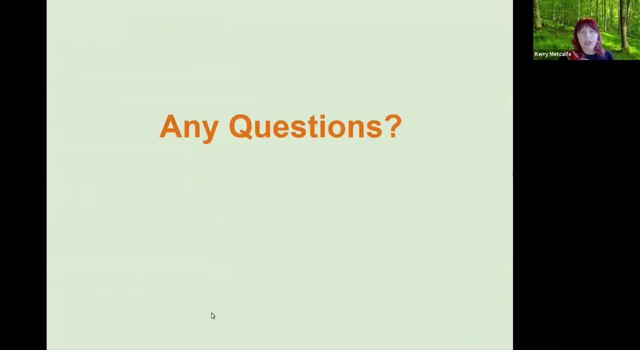 i should also say that in in dingies they can, as they age they can become quite drab and dull and and really fade out, so they look quite worn um, but they should still be distinguishable as as a dingy skipper, and i'll also say that i found that i have quite a few brown argus on my, my site, and 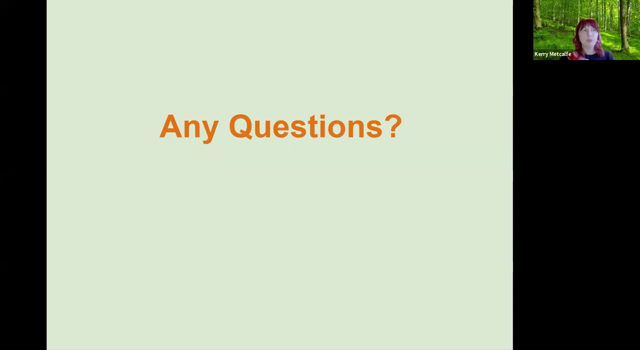 i found that as they jump in the air and flutter off, if you disturb them, sometimes you might be a bit uncertain which is which? but brown argus generally tend to to have a silver flash as they're flying, which? and dingies are a definite brown, so that's an easy way to tell them. um, yeah, i think that's. 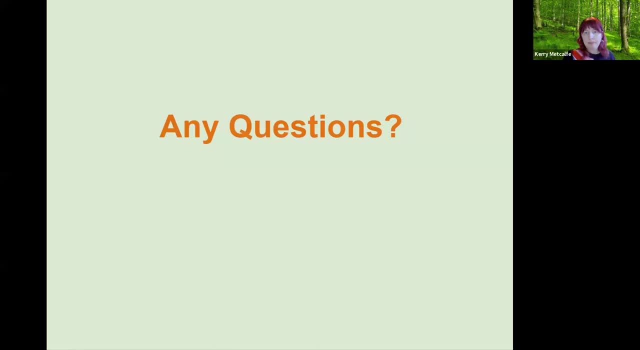 for dingy skippers any questions on them? i have a question, and i believe they fly quite low, is that right, dingy skippers? yeah, they tend to stay low to the ground, um, so i i think it's fairly easy to keep track of them. they are quite, quite quick and they can go quite far, um, but yeah, they'll tend to stay fairly fairly. 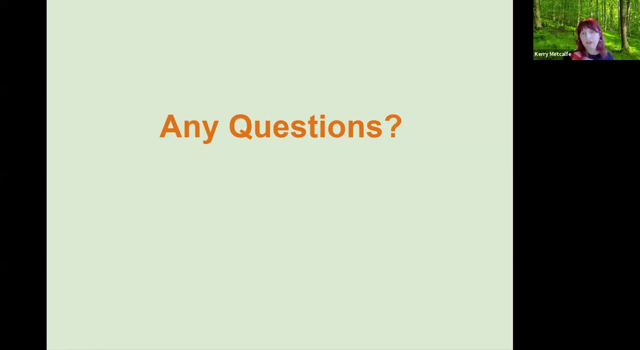 close to the ground, sort of a foot or so off off the ground, and i i find often that i'll just disturb them as i'm walking along. um, so you, so you'll walk along and it's they're quite hard to, in contrast to something like, um, the, the small coppers, but but they'll just leap up as you, as. 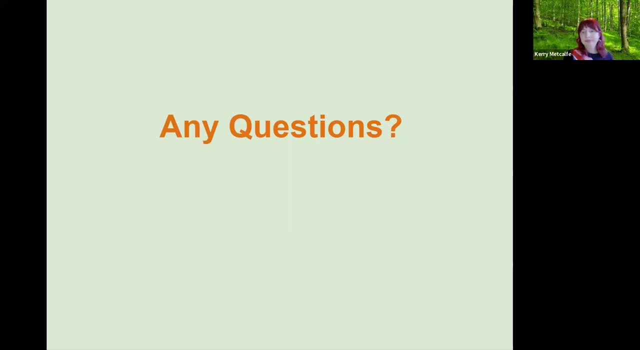 you wander along and it makes it quite helpful really, thank you. um, yeah, i think a phone. it depends how close you can get. i think with something like the- the large and small skippers- it's quite hard to get close to them. so unless you've got quite a high powered phone, you're 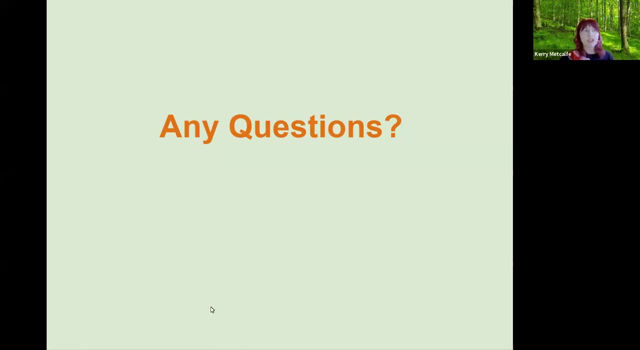 probably going to need more of a dedicated camera, but with a dingy skipper i think they're quite confiding and quite cooperative sometimes, so you can generally get close enough, i think, to use a phone camera. it's all trial and error, so, yeah, go out and try. 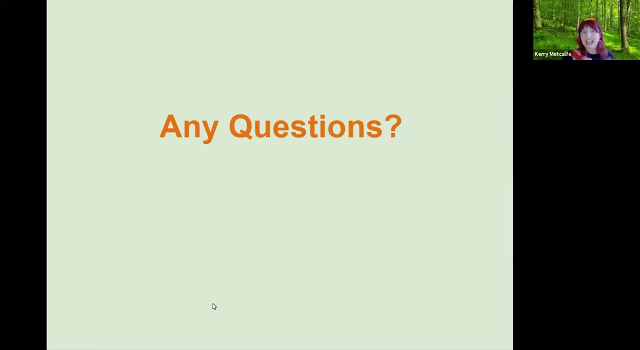 it and see how you do. it's part of the fun of doing this and it has it's fun. we want you to have fun. it's meant to be fun. could i just uh add, uh, carrie, if you go for it, um, i would say of. 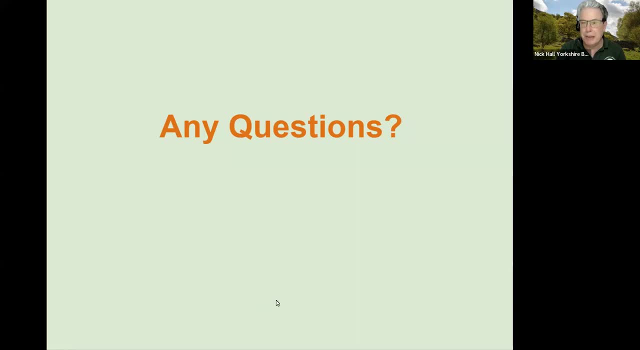 all the species, skippers tend to be under recorded because people miss them because of their speed. uh, particularly the large skipper, which is probably the fastest, smallest um, seemingly fueled on jet fuel. um, they are so quick and people just just miss them and i would say they're the most commonly under recorded. it's. 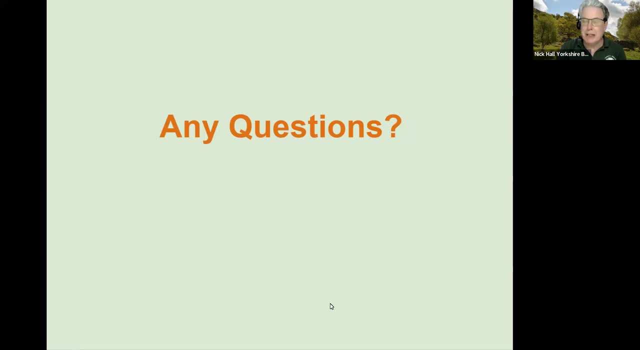 well worth, uh, developing your skills of just picking up that that little movement and trying. i know it's difficult to sometimes determine that movement from, say, a fly and um, but butterflies do have that certain jizz, that certain thing which is different from from from the fly, and uh, yeah, large skippers are tricky, um, small skippers, i think they also have this like: 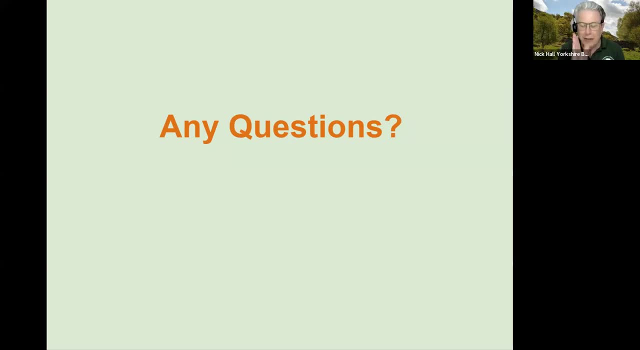 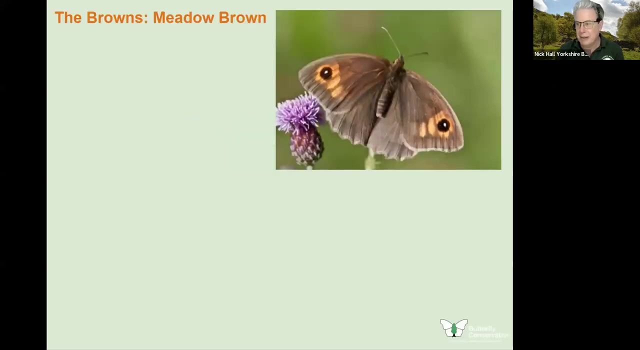 the females in particular like to uh fly between grass blades and they jink along, going um in and out between grass blades as they're looking for a place to to lay eggs, which makes it a little bit easier, while the males tend to be sit somewhere and then ambush things that go past anyway. shall we continue onto the browns? 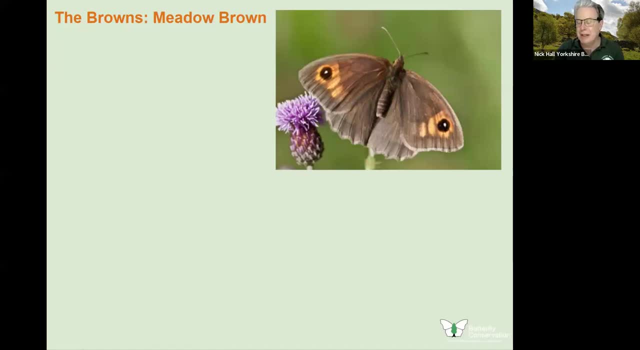 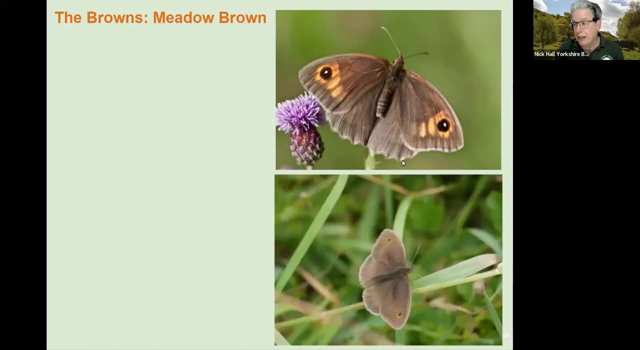 and i guess we've probably count more of more of these than any other- the meta brown, uh, and it's also very commonly um, misrecorded um, and the simple reason is this chap: so above is you've got a female meta brown and below you've got a very typical early in the season when they're very 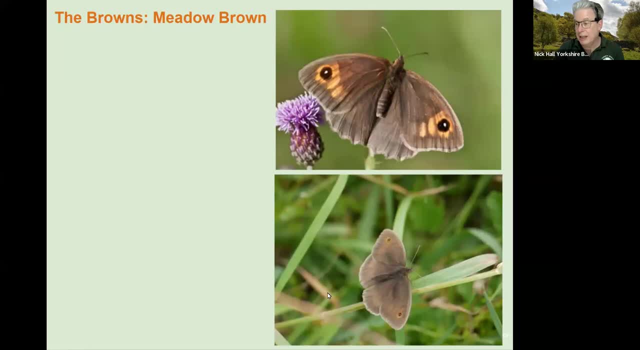 fresh and still got that lovely white edge on them. they look exactly like ringlets, apart from that little bit of brown. but there is this eye spot, which is the giveaway, which you don't see very clearly on the top side of a ring that you do not see clearly: the eye spots. 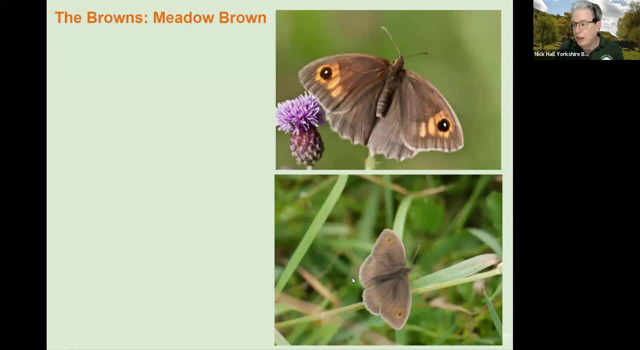 so and also the males occur earlier than the females, so easily mistaken with a faded ringlet. as you can see, the males are saying they appear first and resemble ringlets because they're very dark and the the brown around the eyes is very variable, bit more consistent in the female. 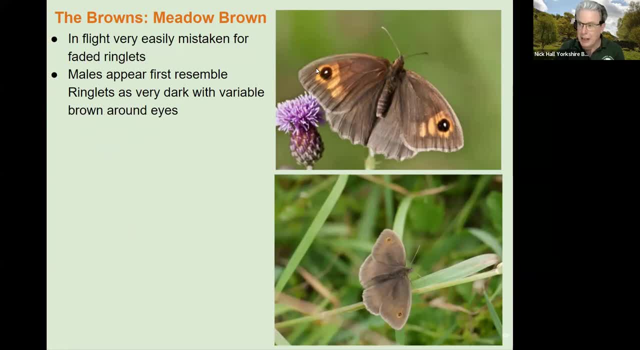 which is a paler color and has generally darker, a larger, more orangey uh marking around the eye spot. so a single black eyes pot. we're into the spots now and we're looking at the pupil, that white bit in the beginning. so the idea of of eye spot is different. 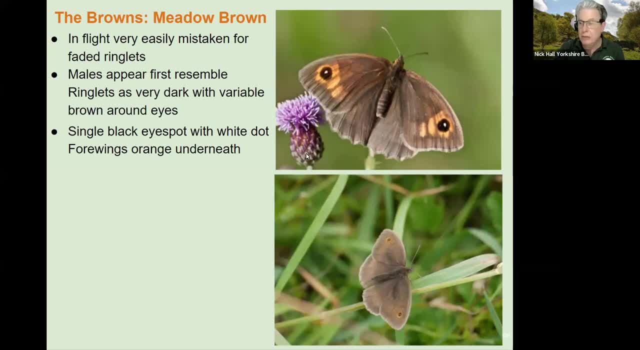 spots is: if you're attacking bird, which bit do you bite off first? if you're a bird, you bite off the head which has the eye on, so it's trying to kill it quickly by biting off an eye. so and really a butterfly can still fly quite happily with a bit missing and you quite often within a 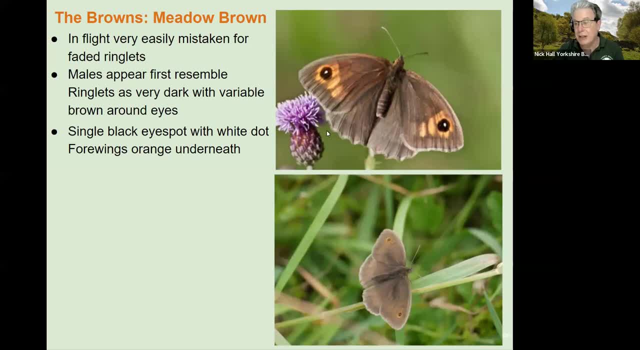 few days of butterflies emerging, you'll see tears and wear from bird strikes. quite often you see the shape of the beak where it struck a butterfly. so spots are a good protection. feelers- larger, paler and more variable orange marks, which we just said, a fairly long flight. 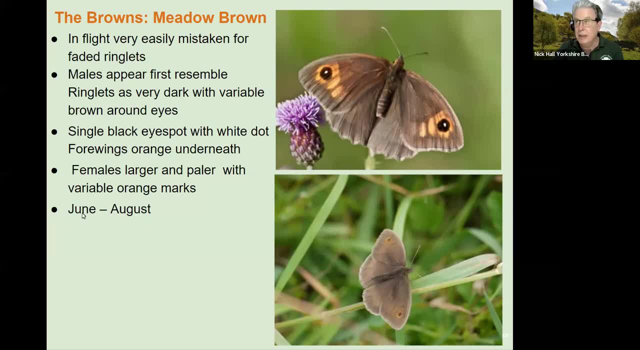 season, so they start in june, usually first half of june, and will carry on into august. now you, the caterpillars, develop at different speeds, and if it's extremely hot, like it was this last june, then a proportion of the caterpillars in the extreme heat will actually 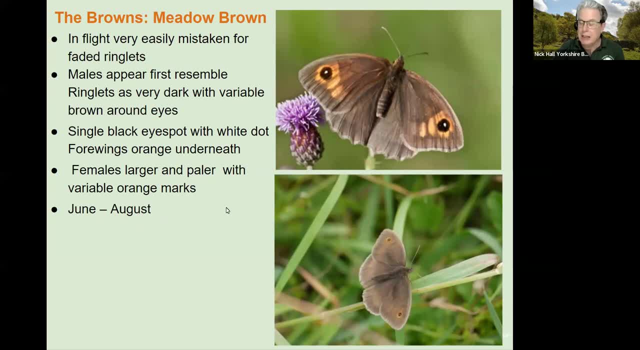 hibernate, wait till it gets a little bit cooler and then come back out again. so you get quite a spread of emergence and it more affects the females, which they're larger and they are tend to be later. so, uh, in certain, as you go south of the country, you find more. 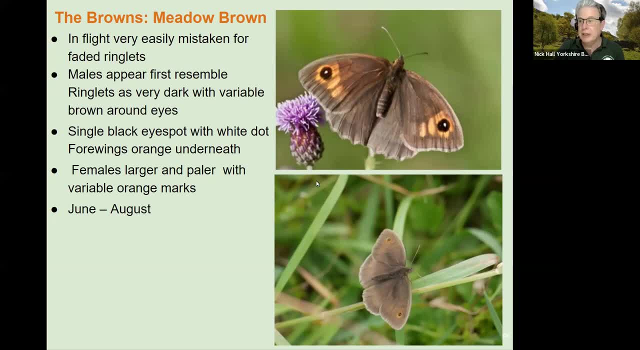 meadow browns appear in august than they do in yorkshire and that's because of this different- uh this diaposing of the caterpillars in the heat, so it's found in places with long grass. it's always in full sun, which is somewhat unlike the ringlet. these are sun loving butterflies. 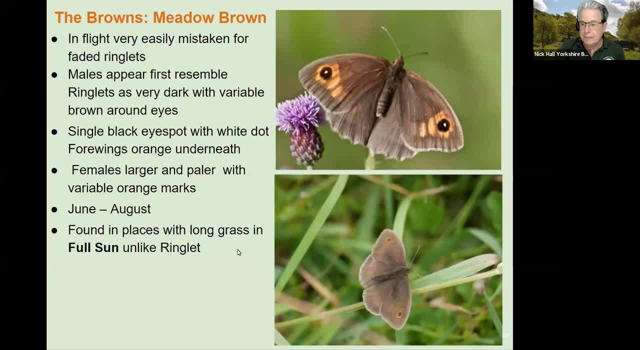 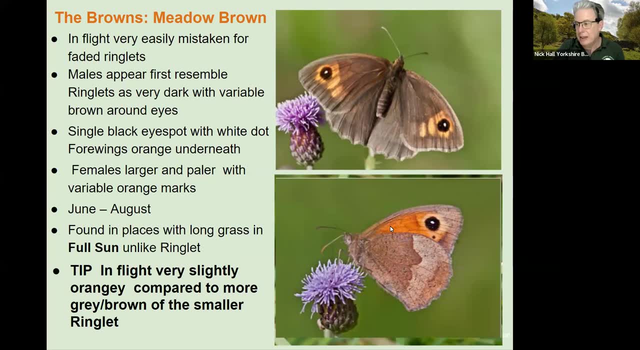 they rarely go near the shade and the big distinguishing mark really which counts, apart from the ringlet, is the forewing. underside is very deep orange, so when it's in flight compared with it, with the ringlet, it is orangey compared with the more gray brain and also smaller ringlet. 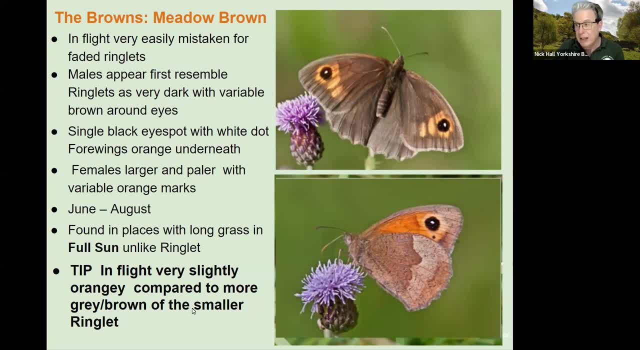 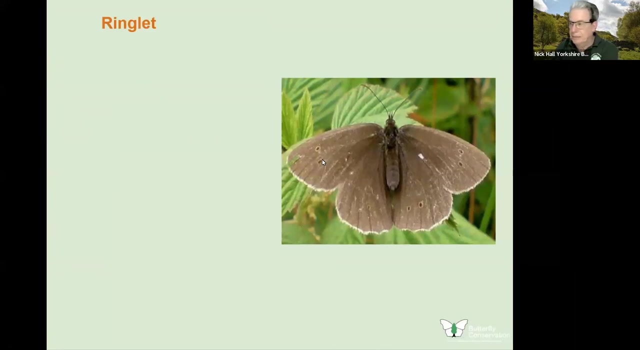 so that's the big tip with these two species. in other words, if you see any shade of orangey brown at all when it's flying, it's a meadow brown and it's because of this underside. so the ringlet is smaller, it's darker, although it goes a little bit darker than the ringlet. 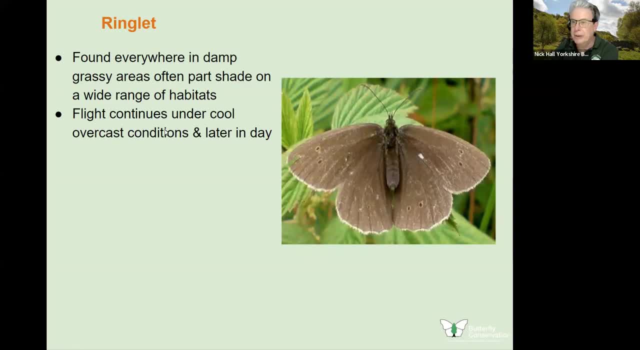 it's paler as it gets older. eye spots are not very visible. it usually frequents damp grassy areas, sometimes in part shade, and you can get them in a wide range of habitats. it's a relatively recent addition to the yorkshire list. um, you don't have to. you. have they really began to move in? 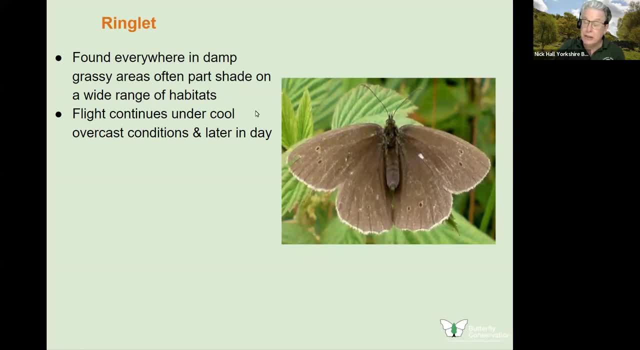 in the 1990s, so it's only been on our a lot of our transects for less than 30 years. it also is capable of flying under cool and overcast conditions, sometimes even flying in drizzle and rain- light rain- and it will fly much later into the day. 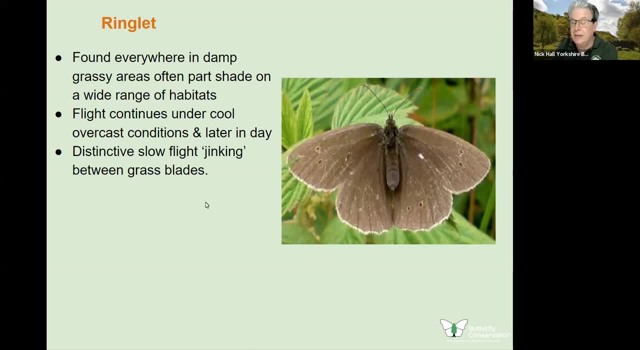 distinctive slow flight, the kind of jinking where, where it's going between, uh, grass blades so it closes its wings to get between the grass blades and then fly away. flaps, jink, flap, jink, flap, jink, like. so if you see that movement, this generally will be a ringlet. 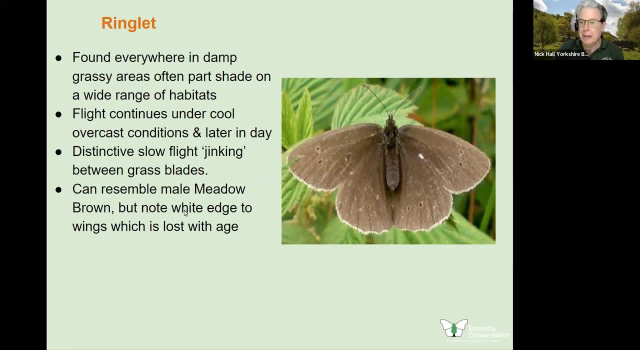 it can resemble a, a male meadow brown, but note that the edge of the wing when it's fresh is white. but it is that white edge is lost as they get older. single generation. but it has a short flight period compared with the jink flap, jink, flap, jink, flap, jink like. so if you see that movement, this 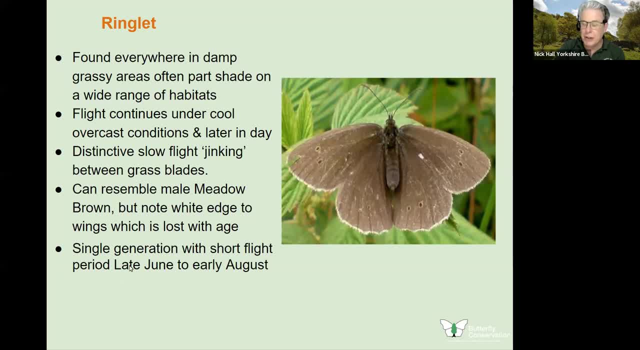 tends to be a wing mold, even though it's just not in the olden days. ウэ хау, depthment, length, length. jink flap jink, flap jink, flap jink like this. and the all长玩, jink flap jink, flap jink, flap jink like that. 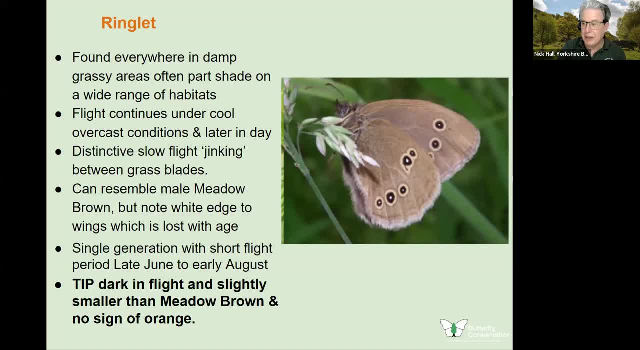 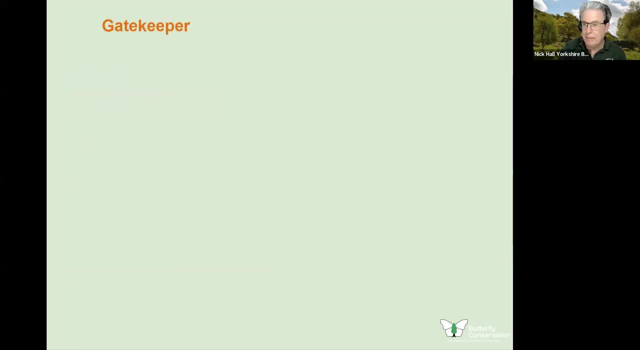 it'll, it won't? the jink, flap jink, flap jink. If you're not quite sure, wait for it to land. have a look at the underside and you've got the characteristic rings of the ringlet, Now the gatekeeper, otherwise known as the hedge brown. 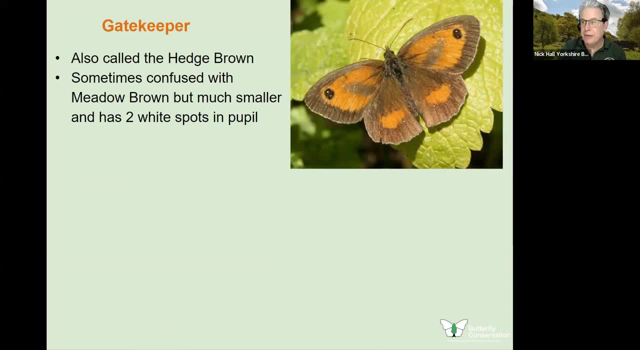 You can use either First of all the thing to say it's much smaller and the eye spot has two pupils. And the most important thing which I use to determine them because they're in flight- is it is very much more reddish orange than the meadow brown. 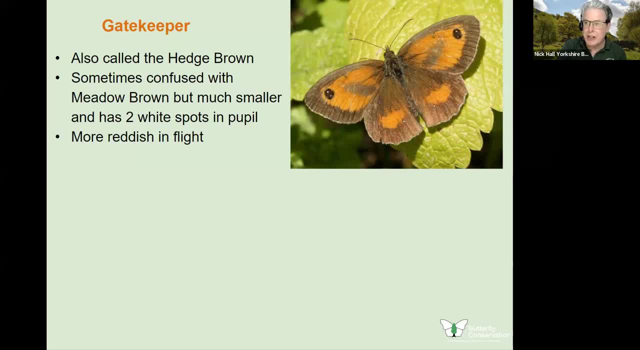 Some people call them the little fox because of its reddishness, And it is quite a red brown. It loves shade, It loves certain flowers, It loves brambles, in particular marjoram, And the reason is it only has a very, very short proboscis. 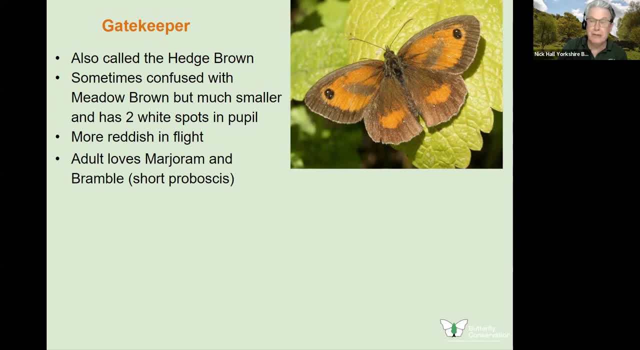 It can't reach nectar on most flowers. It's quite restricted what it can take nectar from. It goes to the tall grasses And surprisingly it always seems to be near gateways, hedges, woodland rides etc. And of course it does. 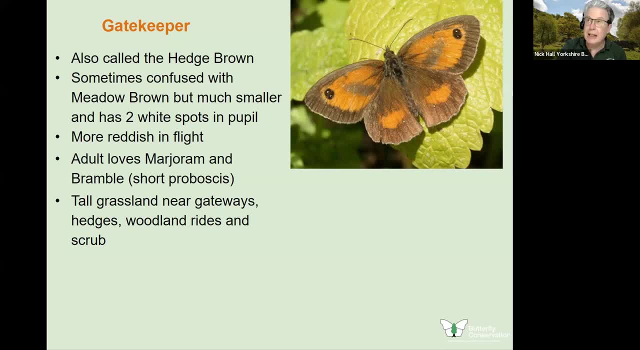 It doesn't inhabit the whole of Yorkshire. The line is, It doesn't quite reach you Kerry, does it? Or only a very few. I've had one, ever, One, ever, Yeah, But if you go to 20 miles south they are abundant. 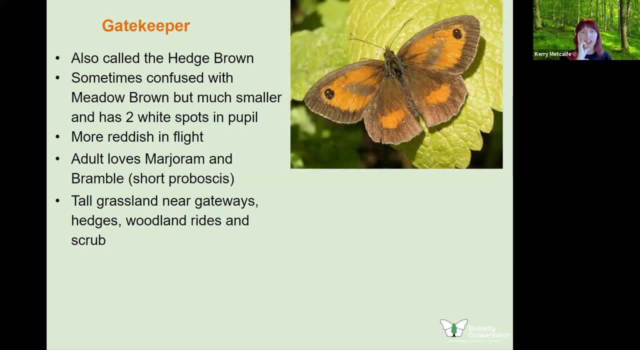 It's kind of what that is. Where is it? If you go to Top Hill Low Nature Reserve, they've got a lot there And that's yeah, that's not that far away. Or even Warren Percy, which is also on the waltz in the same kind of habitat as you. 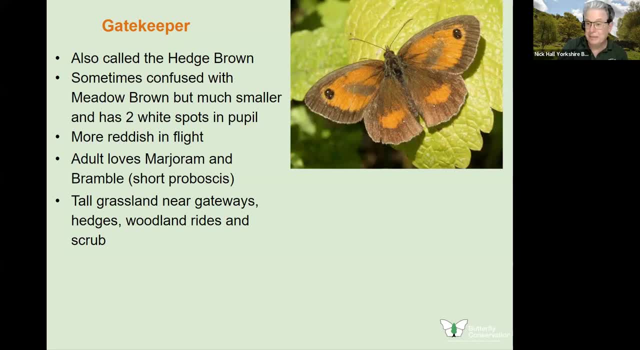 They have good numbers. Yeah, I'm hoping for some. So one generation. So tip is: if it's small and there's a hint of reddish brown, it only can be one thing: It's a gatekeeper. Underside is very attractive. 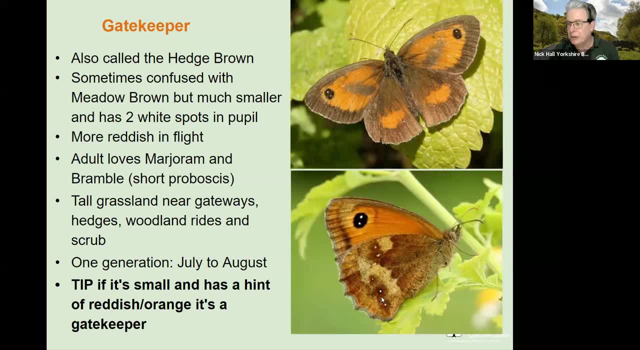 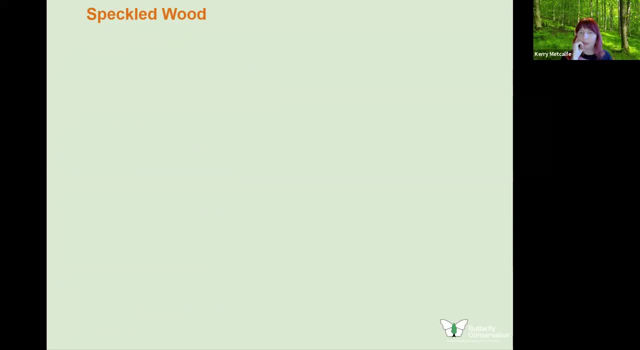 You see the double pupil And some more white spots. So, Nick, we've got a couple of comments coming. So Nairi says that they have them in Lower Wharfdale but not in Upper Wharfdale. 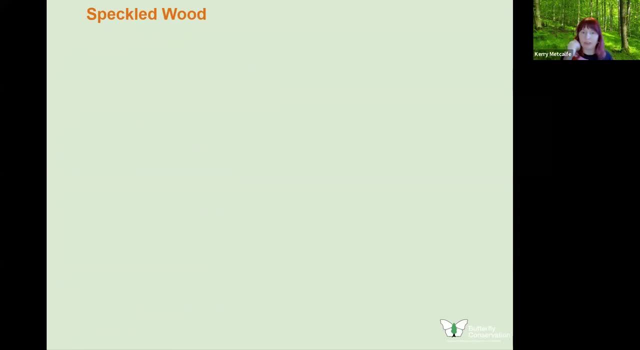 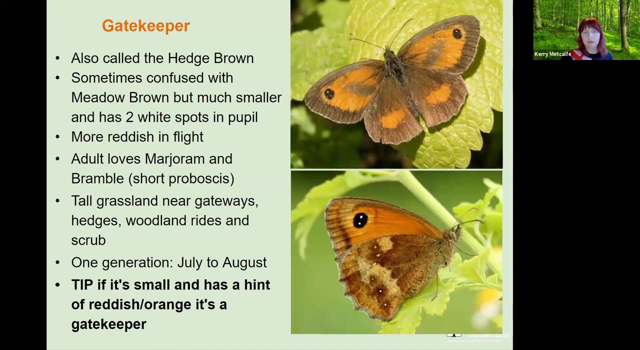 My geography is absolutely hopeless, so I'm not entirely sure where Wharfdale is. And Tamsin asks: could you explain exactly where the line is? Oh heck. So I would say Up to the Howardian Hills and then draw a line. 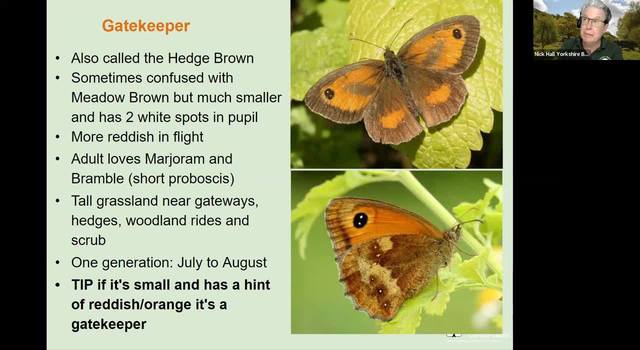 It's kind of a diagonal line from maybe south of Bridlington up the Howardian Hills and Rippon is present, And then it goes up. Rippon is present, And then it goes up the valleys, as Nairi was saying. 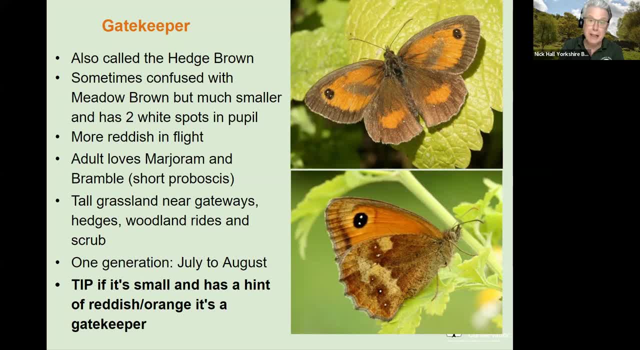 It does go up the valleys but not always all the way up the Big River Valleys of Yorkshire. So the Wharf, the Nid, etc. But it's very much more widespread in the southern part, southern half of the county. 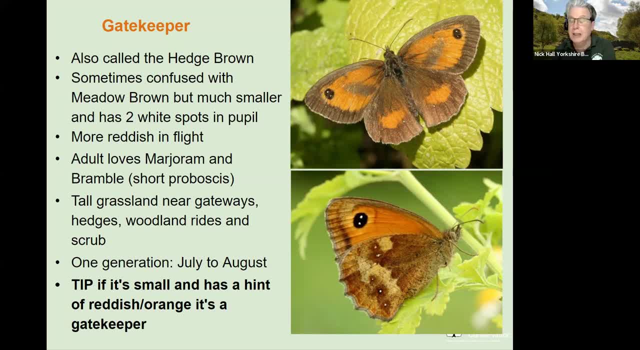 It's almost universal across the Vale of York. Does that answer the question? I hope I've just pasted a link to the Butterfly Conservation website, But if you scroll down on that page it shows you a bit of a distribution which gives you a bit of an idea of what Nick's talking about. 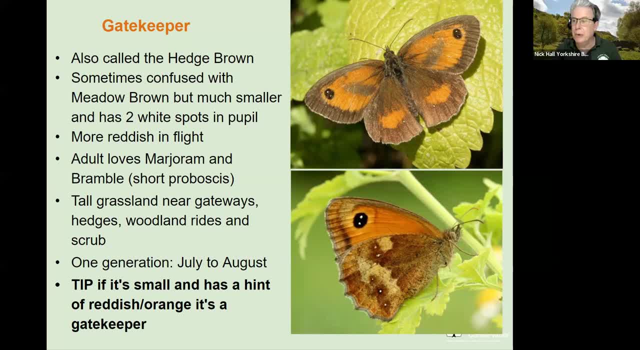 Yeah, That line hasn't changed. surprising with global warming It hasn't changed dramatically, Although you get wanderers even up onto the North York Moors. In terms of abundance, that is about the line. Below that line they're quite abundant. 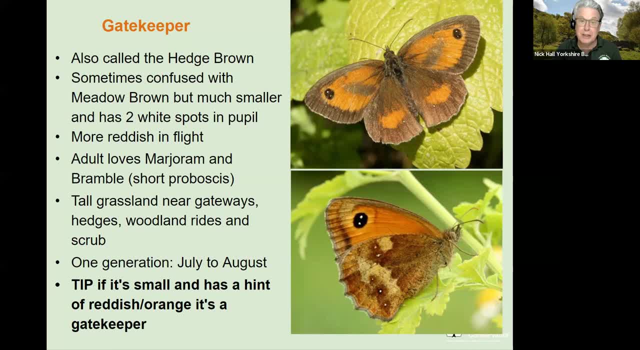 If not very abundant, above that line they're almost non-existent. You get wanderers as Kerry gets on her transect, So you could probably get wanderers almost anywhere, So it's something to watch out for wherever you are. Tamsin asks as well: would it be likely to occur around the settle area? 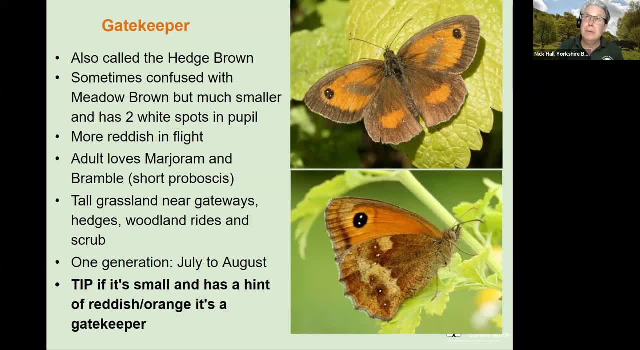 The lower parts, Probably. Probably, If it's really down in the lowlands, yes, But I think we're dead on the line at settle. That's a bit way up the turns. on altitude, I would say anything less than 100 metres might have a chance. 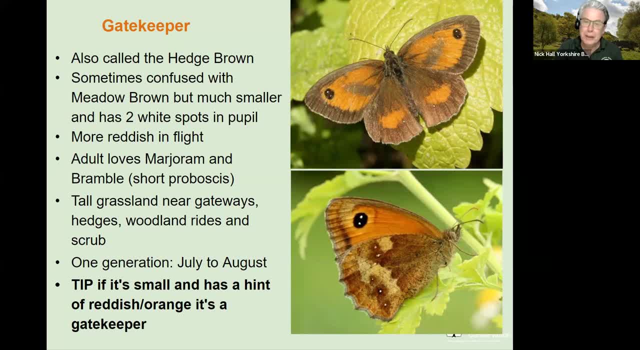 Anything more than 100 metres. no chance at all. By the way, 100 metres is about one degree centigrade, And I think that's what we're talking about here. It's a small difference in temperature. I'll move on to the speck of wood, if I may. 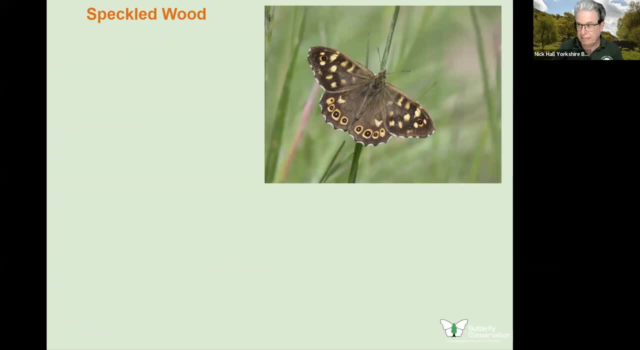 This is a really interesting species: Dark, chocolate, brown flecked with yellow creamy spots. That colour changes a little bit through the seasons. Males defend sunspots and sunspots are our big friend, Because sunspots enable us to find this little blighter in woodland. 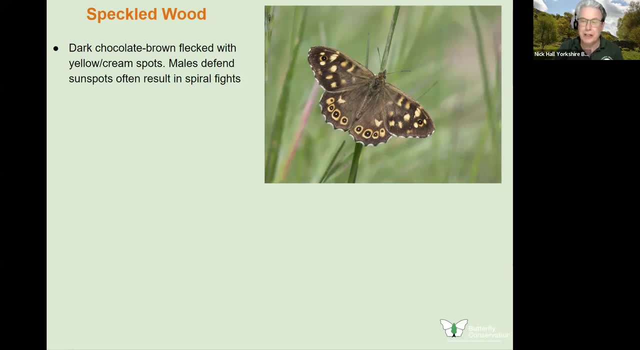 um. if you passed a shadow through that sunspot, it will always take off, and usually if it takes off, there'll be three or four of his mates will spot that one insect take off, in which case you then get a spiral fight to go on. so it just they spiral upwards um and gather more speckled woods. 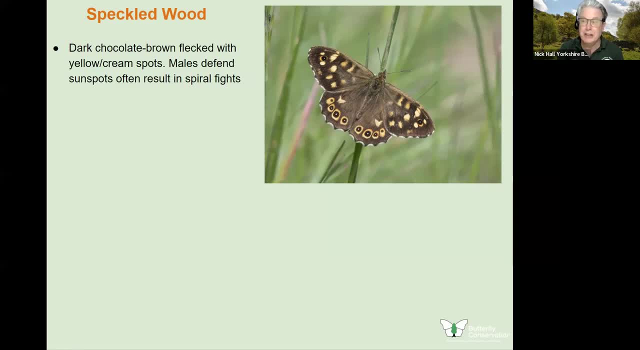 as they go. but it's also always the rest that sunspot resident speckled wood returns to his spot, the others just diffuse away and the resident returns to his spot to stand guard. its life history is quite complicated, so you have three overlapping generations all the way from. 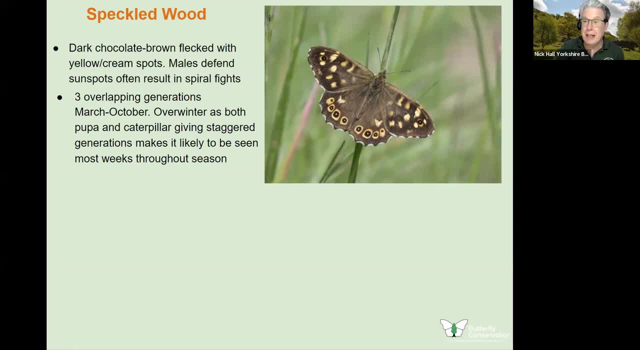 march to october, but the overwinter is both pupae and caterpillar, so you yet are somewhat staggered generations. So at the moment, and it's quite surprising at the moment, the reports coming in from our transects are quite startling. People are getting more than double the number. 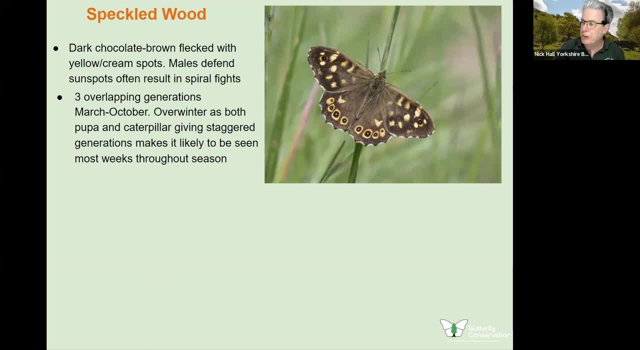 they normally get at this time of year. I had one report of 30 from a graveyard, which is nearly double the normal, what you see at this time of year. They've had a big hatch And the reason is they're hatching from pupae. 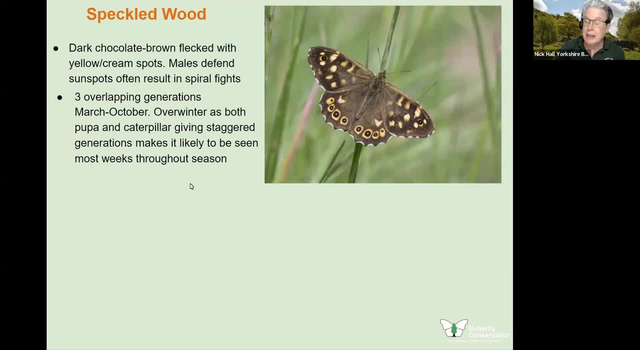 And because of the warm weather, they've all hatched together. They'll live for about a week And then they'll be replaced with butterflies which are hatching from caterpillars which overwintered. So you get this kind of double peak in each generation. 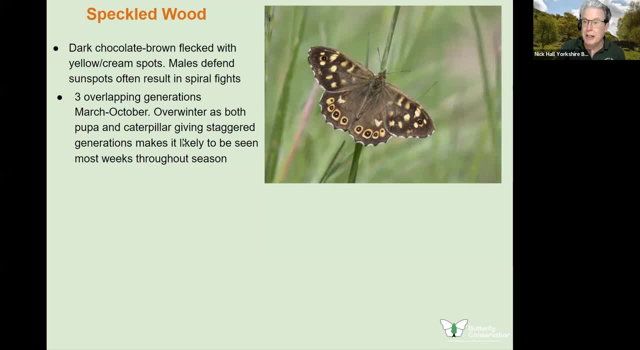 It gets more and more blurred as you go through the year And the result is you can see speckled wood. now I would say every week throughout our season. There'll be dips, but you can see them throughout the season. It loves grassy vegetations, woodlands, but it also likes 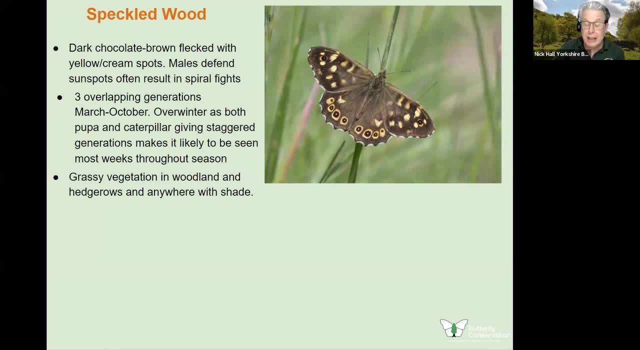 and this is a big change really in its behaviour, which happened around about again about 30 years ago. It switched from being a woodlander, a woodland species, to being a species of hedgerows and shady areas. So around where I live it's extremely common on field edges. 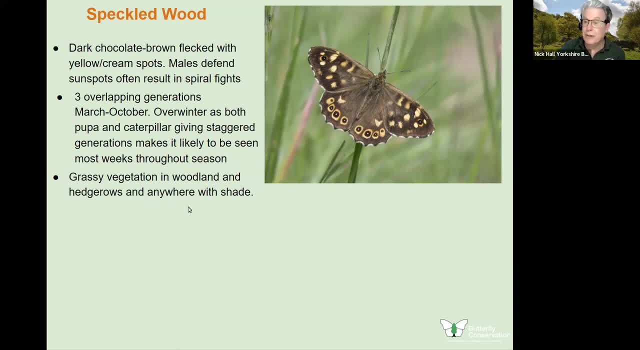 If there's a little bit of shade, that's all it needs for a few hours during the day. it gets a bit of shade from the surrounding trees. It's enough for it to breed on, And the numbers of speckled woods we're seeing these days compared with 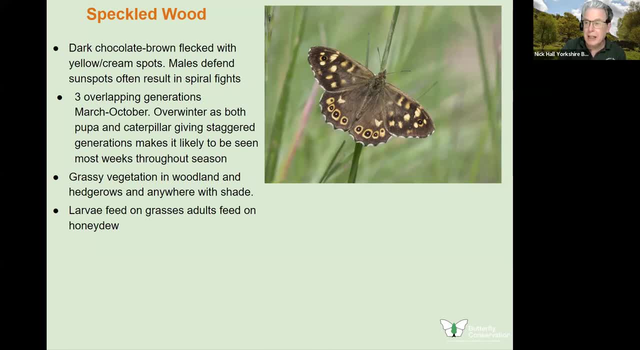 20 years ago. it's much, much bigger. It's probably going to rival meadow brown before long as our most abundant species. The larvae feed on grasses and the adults feed on honeydew, So this is the sticky sugar that comes from the rear end of an aphid. 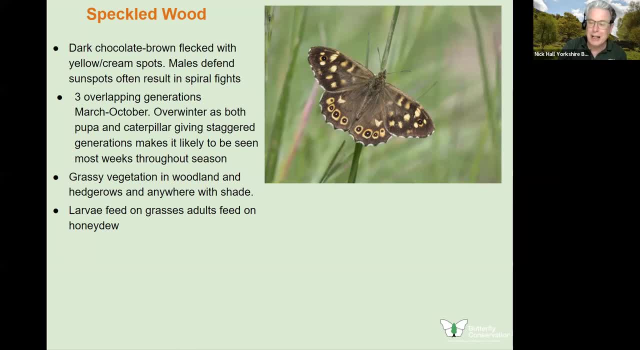 So if you've got sycamore trees which are prone to getting stung, you can get a lot of honeydew. So if you've got sycamore trees which are prone to getting stung and the leaves underneath get sticky, 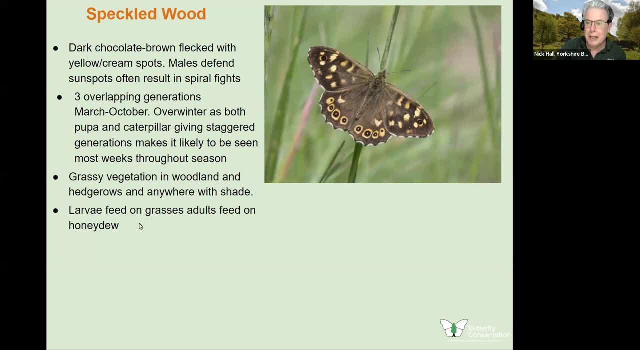 they are basically feeding on the honeydew from feeding aphid, which of course, is very common. There's a tip I can give you on the flight. It's quite characteristic the flight of a speckled wood is. it will beat and then it will glide. 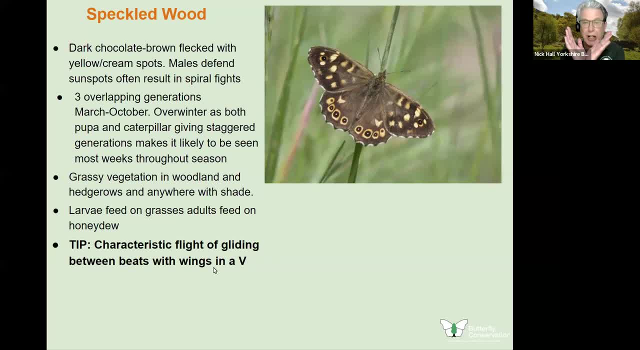 And when it glides, it glides with the wings in a V shape, And when it glides, it glides with the wings in a V shape. So if you're following one, you'll see a beat, glide, beat, glide. 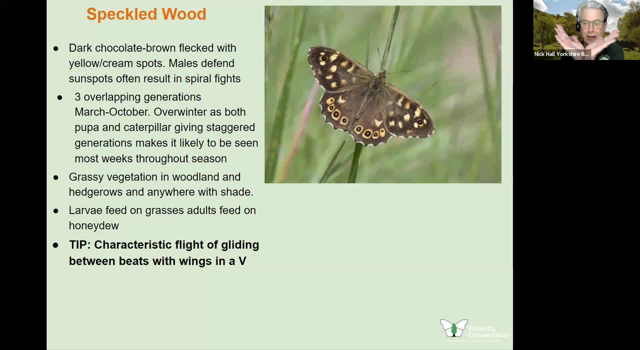 So if you're following one, you'll see a beat glide, beat glide And you see that V shape And it's very characteristic: speckled wood. I mean the color is fairly obvious, but just to double check, 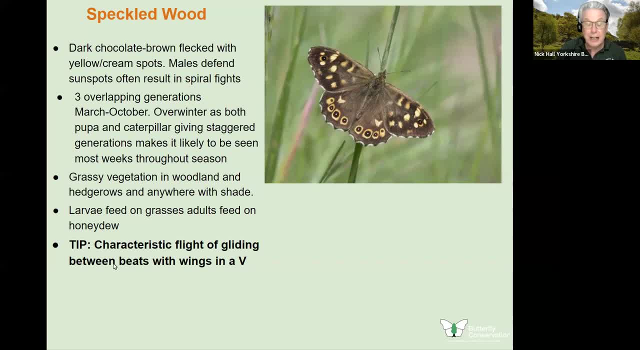 if you see that characteristic flight, you've cracked it And I always check. when I'm walking, I always check my sunspots And I would give this as number one tip: check your sunspots for sitters. I call a sitter as an insect that is perched. 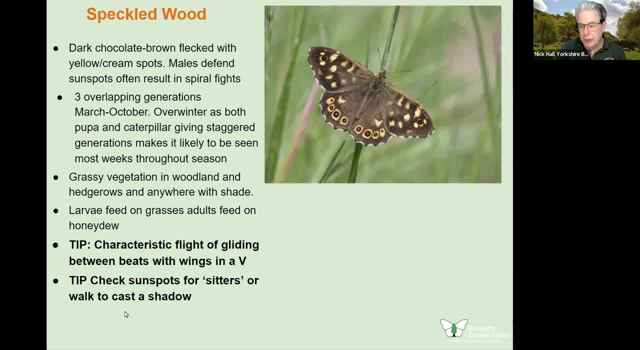 And as I'm walking, you must keep to your route, But I always allow my shadow to go across any sunspots if I can. If it's reasonable, I can just move to one side of my path and if it's a shadow, through a sunspot. 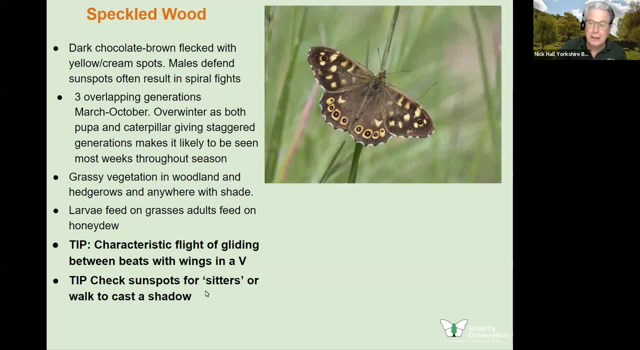 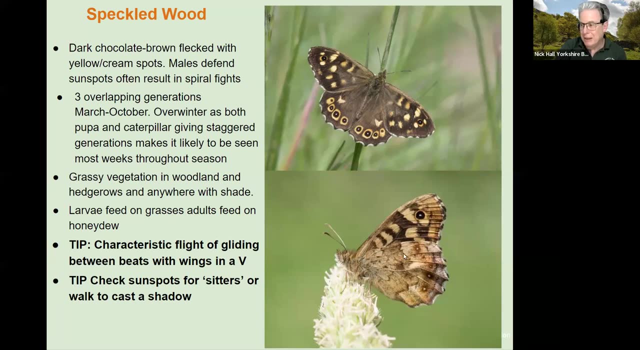 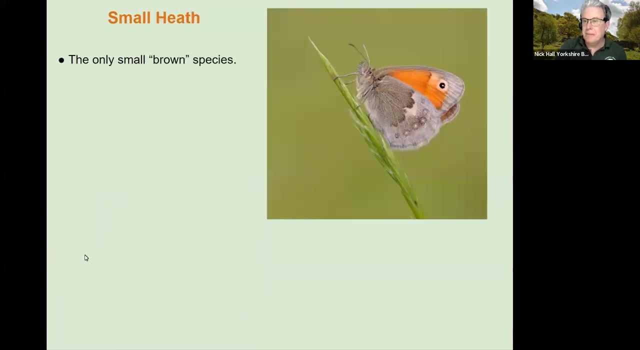 That's usually enough to bring up an insect, And it's surprising most sunspots on my transect are guarded by speckled woods. This is the underside, quite plain. You've got the eye spot. Now moving on to 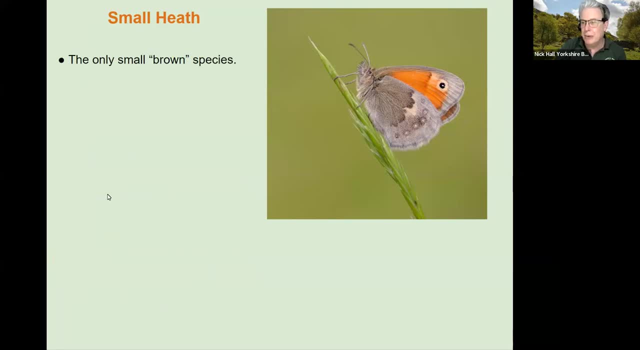 And this is our smallest brown species, The small heath. It's declining and it's now threatened in the UK But still, fortunately in Yorkshire it's still pretty common- Always sits motionless, with its wings closed. It aligns itself to the sun, so there's no shadow. 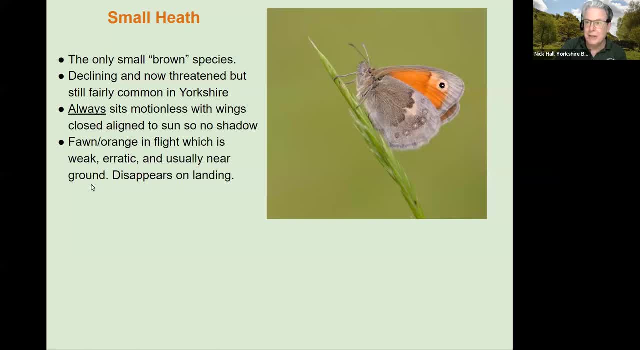 That's another little characteristic some of the brown species have of not getting eaten by birds is as soon as you land turn, so you have no shadow In flight. it's a fawny orange colour, Unlike the colour you see here on its wing. 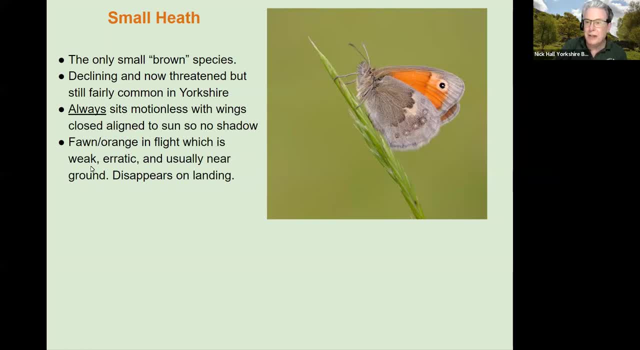 and I'll show you why in a minute. the flight is very weak, fluttery, erratic and usually very close to the ground. As soon as it lands, it tends to disappear. for the reasons above, It has one pupilled eye spot. 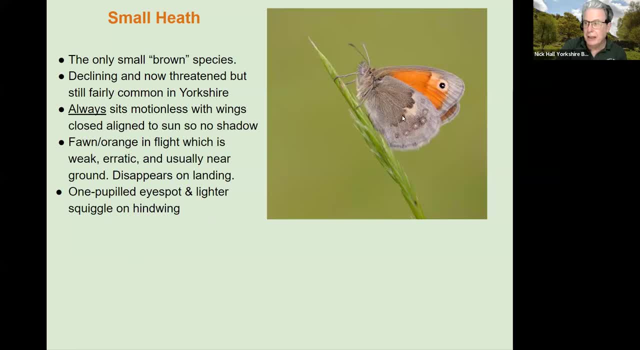 And you also see this little light squiggle here. It's quite distinctive and makes it different from other species. Colonnades tend to be small. They're found on rough, often Tuskegee, grassland of commons heaths. 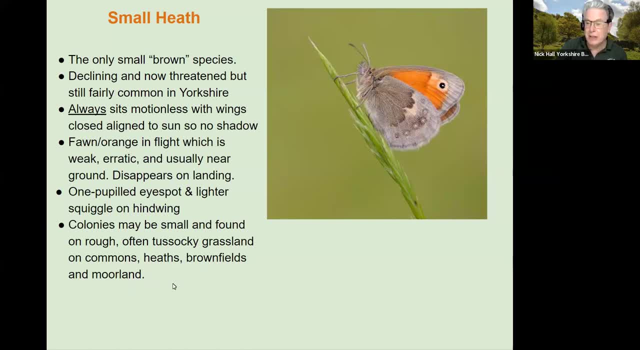 brownfields and moorlands, So quite a range of different grassland habitats. There are two overlapping generations in Yorkshire, one starting in May and the other towards the middle of July, But they tend to overlap. There's only a small gap between them. 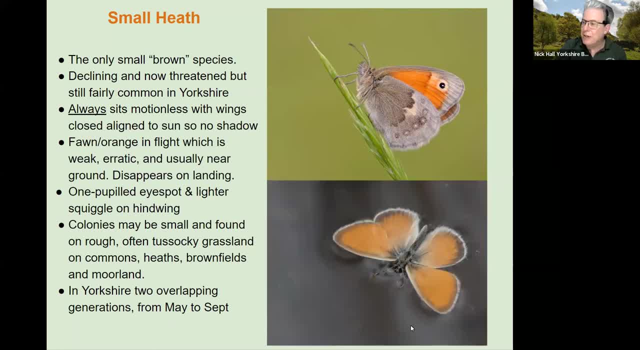 Just so you know, if nobody's ever seen one, and very few people have ever taken a photograph of a small heath with its wings open, this poor chap fell into a puddle And the photographer managed to get a photo of it in its prostrate condition. 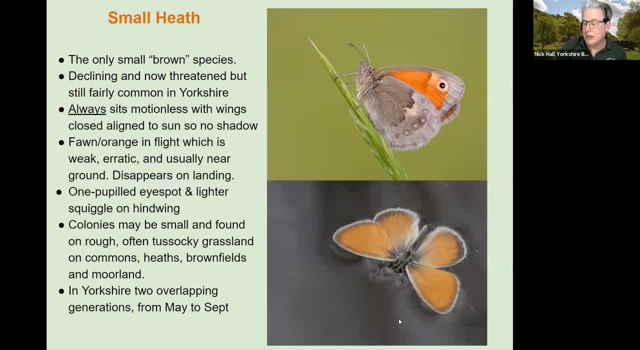 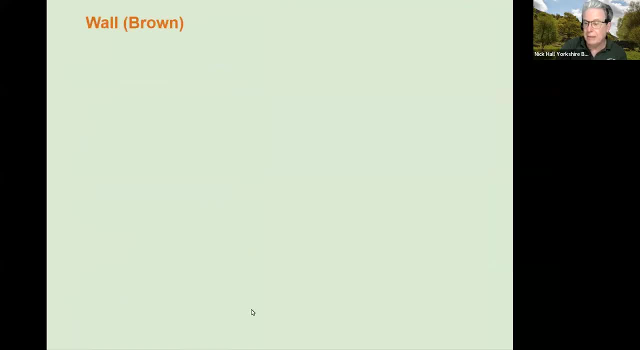 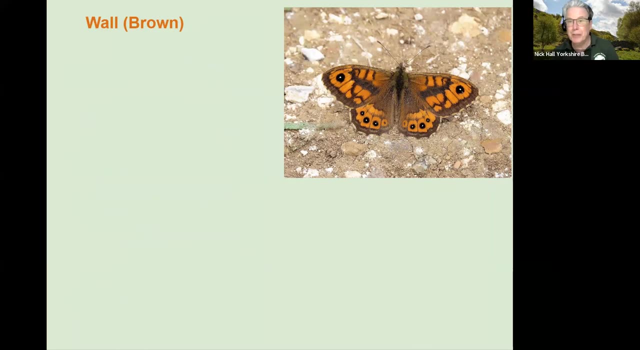 to show us exactly why it looks the colour it does, And that is the colour that you see when it's flying. It's that topside colour, It's just a fawny brown. I'm going to hand now to Kerry for her species, the wall brown. 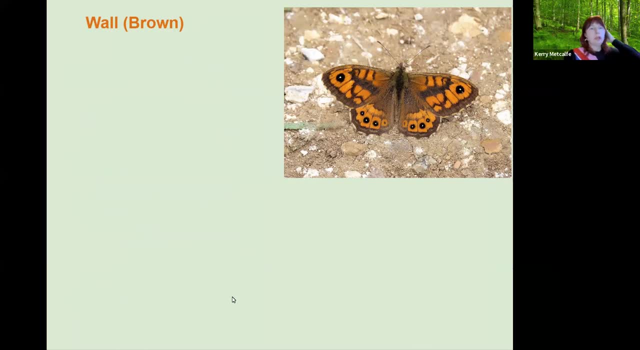 Excellent. Thank you, Nick. So wall brown, often abbreviated to wall, So sadly a bit scarce really, from Lonely New Yorkshire since 2010.. I'm just posting the corresponding page on the Butterfly Conservation site so that you can see the distribution again. 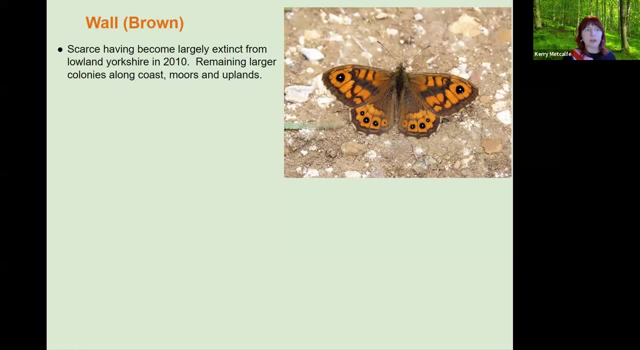 Because if you have a look at that, you'll see where the gaps are. So we can still see them in colonies along the coast and the moors and the uplands. So I have them on my transect on the edge of the moors. 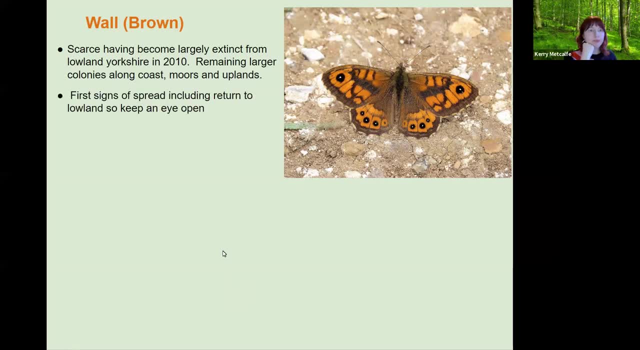 But, yes, sadly vacant from the lowlands in recent years. But good news is that they seem to be coming back. So worth keeping an eye out for them And quite hard to miss them. So wall are very strong flyers. Often you'll just see a flash. 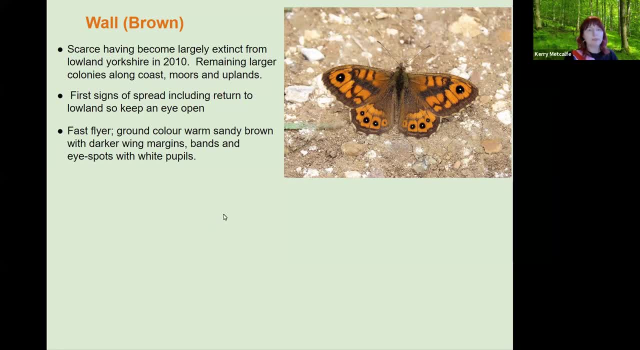 of this fantastic orangey-brown colour. They're quite distinctive with the eye and those markings. There's nothing really like them apart from the dark green fritillary. You will generally see them in rough grass And, again, like some of the species, 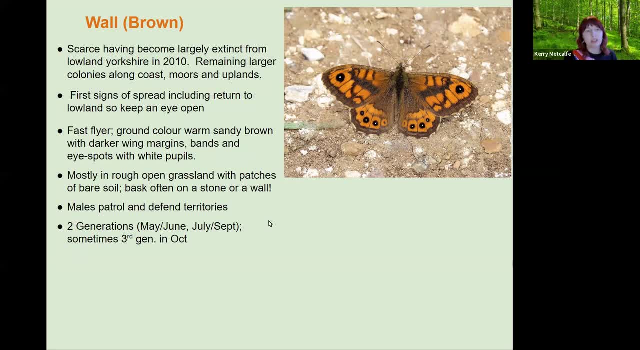 on patches of bare soil where they like to bask and sit and just absorb the sun. like many of us Males are, I would describe them as argumentative thugs. They like to patrol up and down and defend their territory, And they'll often chase females. 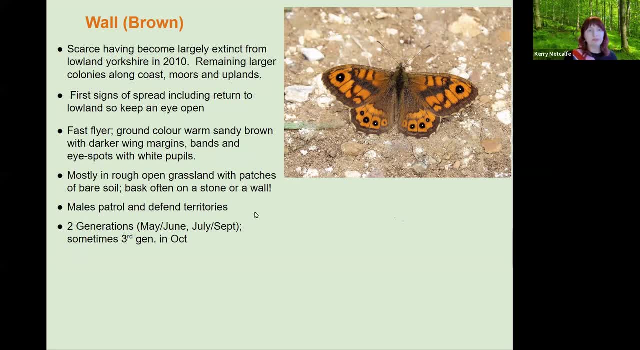 and fly about into the air, But, yes, really strong flyers. So two generations. So you'll first see them in May and June And then again in July and September, And then occasionally, when we're really lucky, we might get a third generation in October. 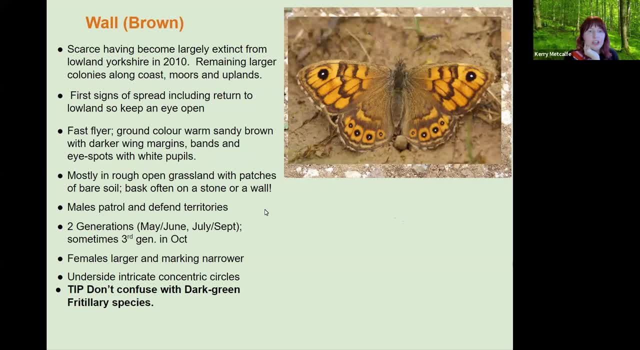 So females are larger and their markings are narrower. So that's quite a nice distinction. Could you just flash back and forth again between those? Nick, Yes, so the males are just a bit smaller and the markings are just slightly chunkier. 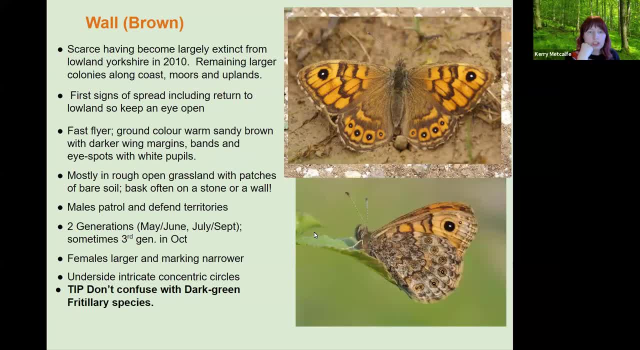 And they're undersized, As you can see here- has these fantastic concentric circles. I think that's a beautiful under marking, Not dissimilar to the way that the orange tip is marked, Different obviously, But just that almost speckled-y. 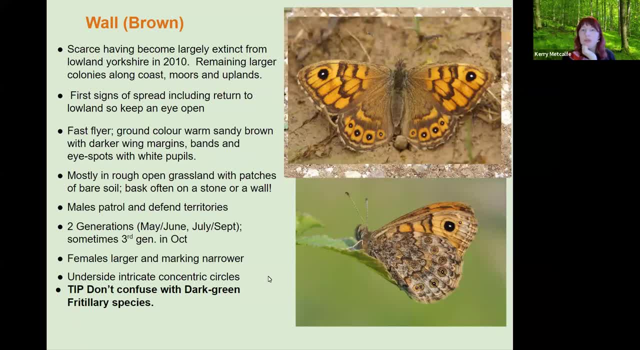 With wall. they're similar in size to the gatekeeper, but where the gatekeeper is just on the other side is just generally quite orangey. they have that really distinct patterning so you can generally tell and and obviously that really strong flight, you're more likely to confuse. 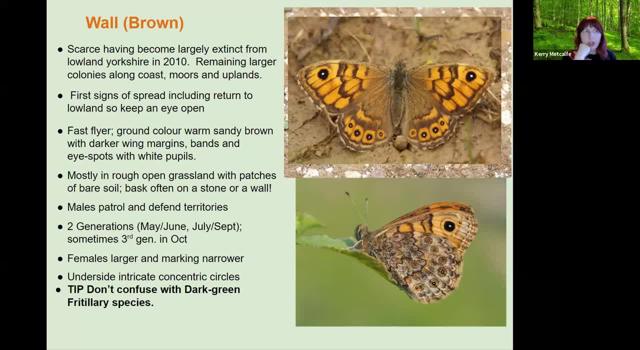 them with the dark green fritillary: um, also a species that's very strong flight and looks like it might beat you up if it bumped into you. um, but where, where wall of a fairly sort of medium size butterfly dark green fritillary are very large, um, and again, with your transit you'll get. 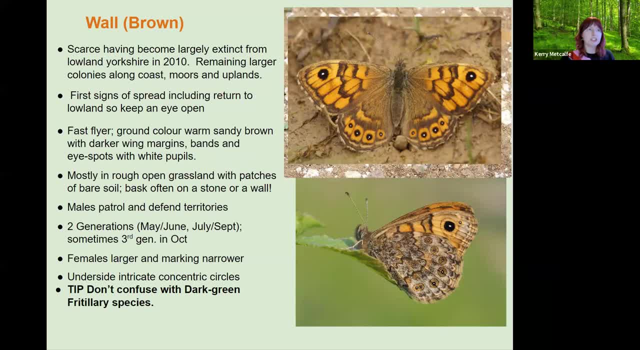 a feel for where you might see these species. so so, for instance, with mine, i know that i'll see dark green fritillary generally in sections eight and nine. um, so if i'm seeing something like this, that's flying by me very quickly and it's bright orange and i'm not entirely sure. 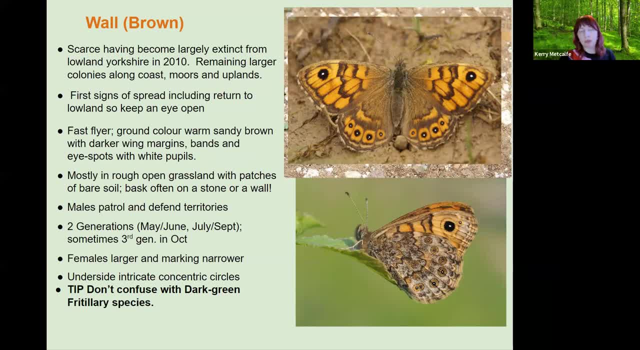 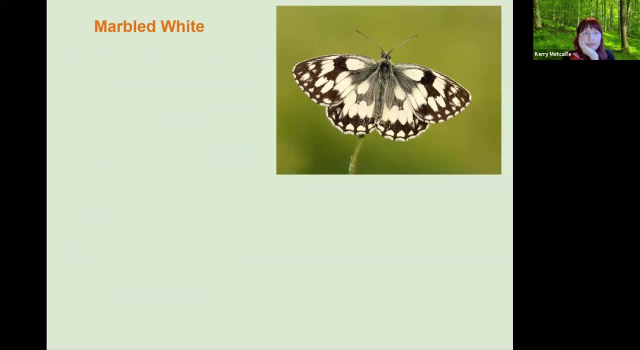 on balance of probability, it's probably a brown, a wall brown. if it isn't, um in in the area, i'm expecting to see dark green fritillary. so yeah, um, you're looking for the markings and the size to differentiate between the dark green fritillary. so i will now hand back to nick for the beautiful. 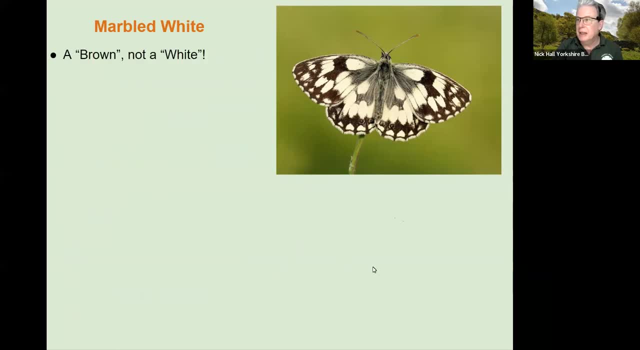 marbled white. thank you, yes, uh, no wonder it's the symbol of yorkshire butterfly conservation. it's a. it's a beautiful thing, but it's not white. it is actually a brown. uh, it's a brown with with white markings, so don't think of it as a white. 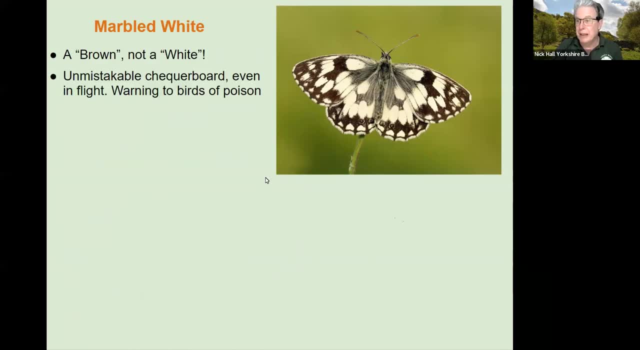 uh, so unmistakable checkerboard, um, and you can see the checkering in in in flight and the reason it's checkered is it's warning to birds that i am poisonous. um, it has some pretty potent um uh, alcohol, alkaloid, um poisons- they actually gets from a fungus. 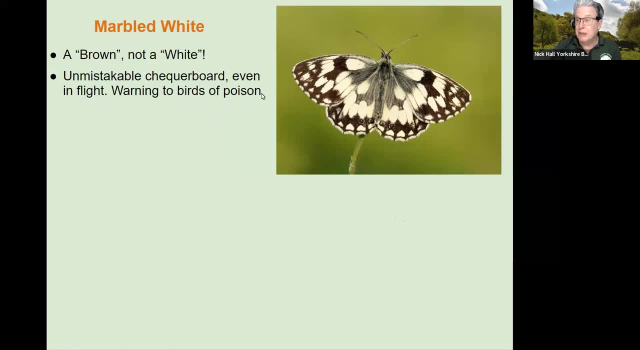 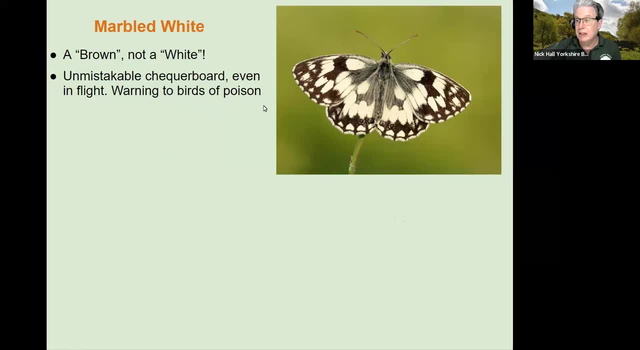 they will not lay eggs unless she smells the fungus, which is the ergot fungus um, which is famous because it has a black bodies, uh that stick out of the uh where, where, where the grass, the grass seed was going to be, you get a, a black uh body of an ergot um, and that's what the female 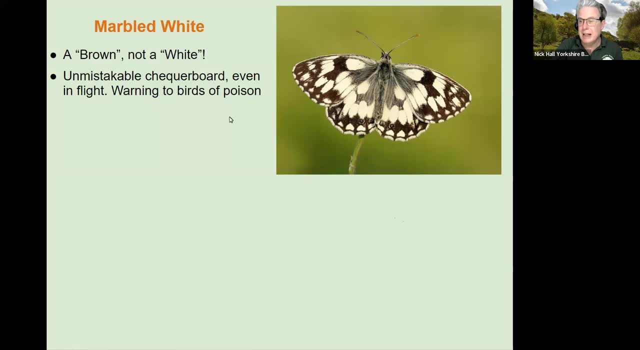 is trying to find, because that indicates that the, the fungus, is present and therefore my will be protected by the poison, and i'm going to tell the whole world that i'm poisonous by being this startling wonderful marbled color. uh, colonies tend to occur in in medium height. 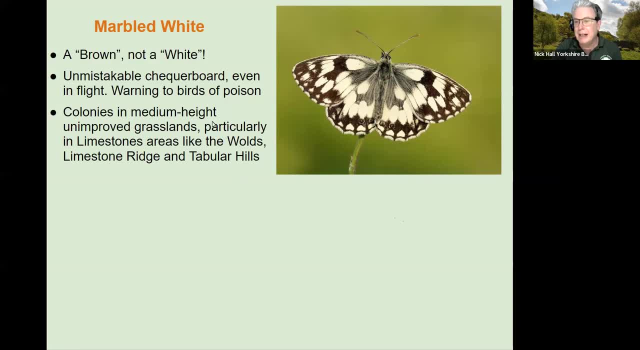 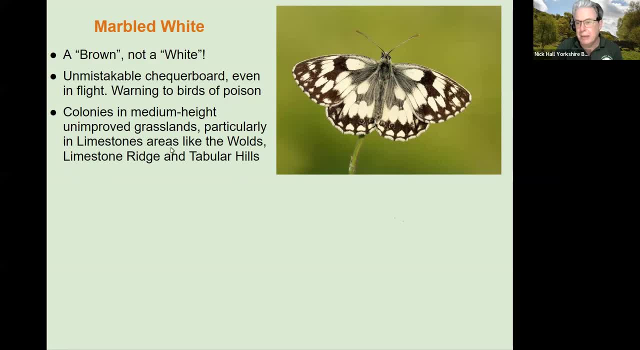 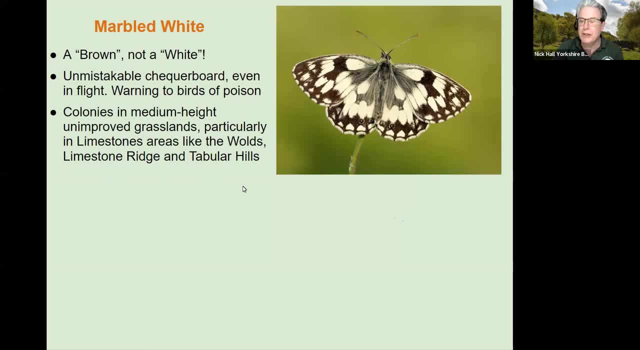 hills um on the south edge of the north york moors uh, which are chalk um. it's the only bits that are are chalk is where the rivers have cut through the and exposed the chalk um significant spread in recent years. it's beginning now to appear on. 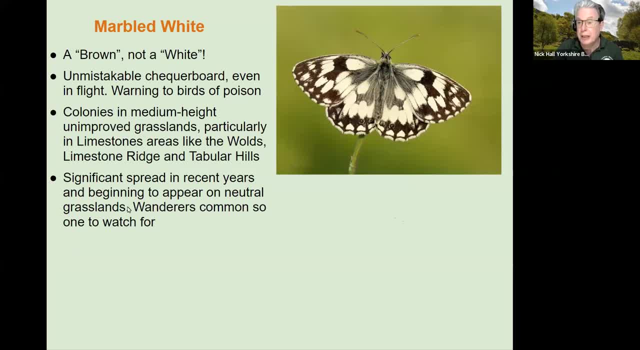 neutral grasslands, uh, around york. you don't think of york as being a place you would see marble white, but it's actually quite common, uh, only in very low numbers: ones, twos, threes or fours. railway embankments, road embankments, uh. fields and parks, uh, i've even had it in my garden, which. 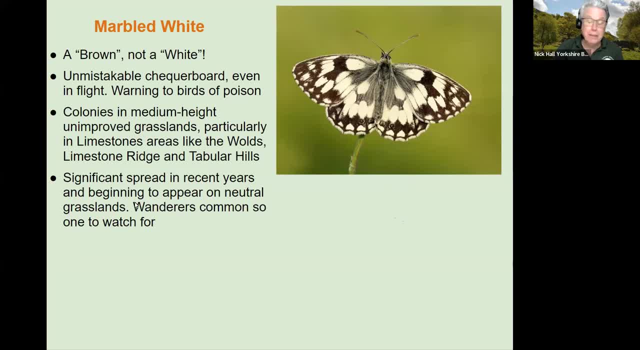 is in the middle of agricultural wilderness, in the middle of veil of york. so they are actively colonizing uh the veil of york and if they find a suitable grassland um they are colonizing. so wanderers are very common, so watch out for those. uh larvae feed at night um one generation. 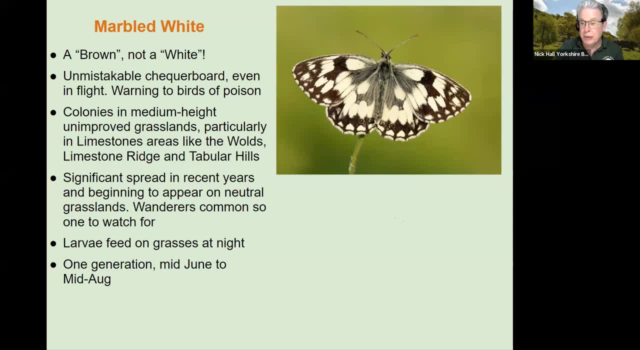 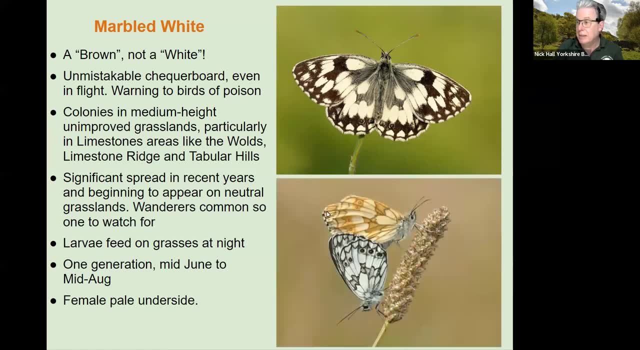 which lasts from mid-june to mid-august. um. the female is a very. how you tell them apart is um. the females are very light colored compared with the male, dark colored on the underneath and in the adult. this is a female. it's very slightly creamy. 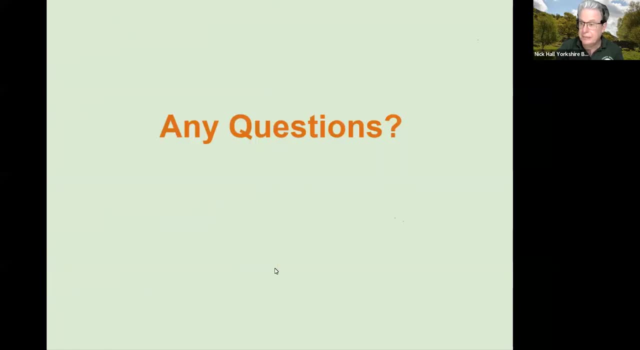 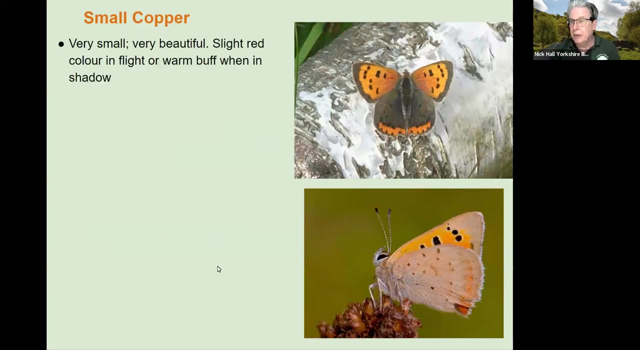 colored. that's how you tell the sex is apart and that's the end of the browns. so i'll ask questions at that point. okay, we'll carry on. let's carry on to the coppers, the blues and the hair streaks, the lysinids family first up. it's quite unique. it's a very small, very beautiful, uh, red in color, in. 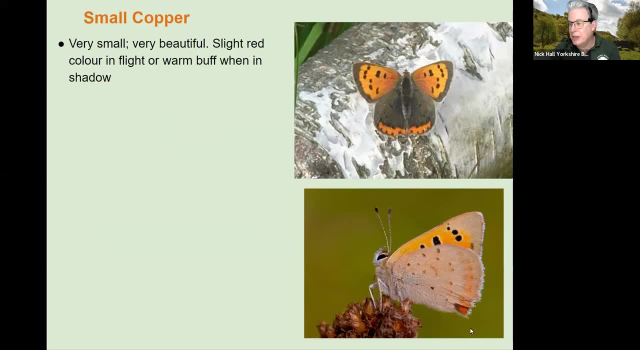 flight. uh, a more warm buff color which is the underside um when it's in shadow. but it's our only red butterfly which is really really red. uh, active, erratic, fast line, difficult to follow because of its typical hair streak. uh lysinid behavior. it's very fast and it changes direction quite quickly. um, quite often flies high. 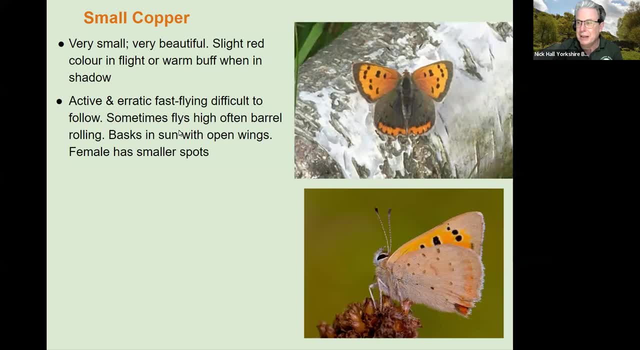 and you're quite often seeing it barrel, rolling down a down a woodland ride, and it is quite common in in in woodlands, baths in the sun with open wings. and the female. how you tell the sexes are far apart is this is a female, the spots are small and its body 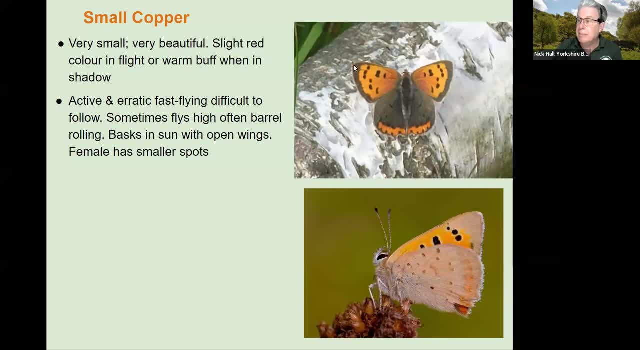 is a bit more chunky, uh well, and the band here is quite narrow, while the male this is wide, the spots are bigger. you'll also see, um, sometimes little blue spots here, just above the bottom here, which is a different form of the same species. you can write it down on your recording form as a note. 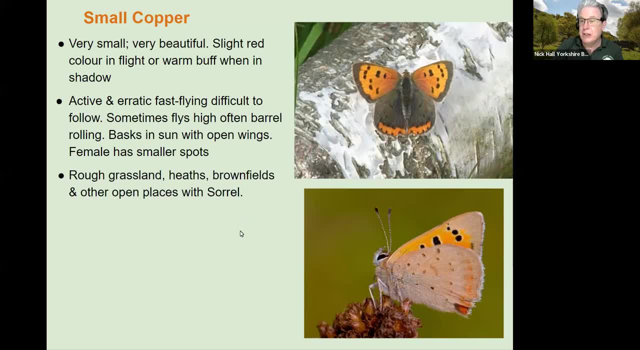 um and out of interest. so it's a species of rough grassland, heath, brownfields, other open places where there's sorrel, small, discrete colonies. it's not uncommon. it's a pretty mobile species. rarely occurs in any big numbers, i suppose. when i'm counting on transects, i suppose a count of 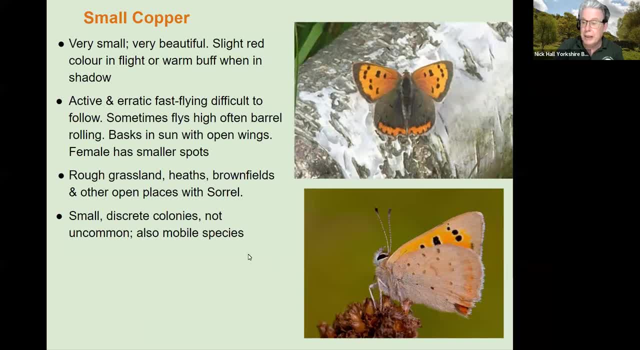 two or three would be, uh, quite common. there are some transects where they can get up to 40, 50. and that tends to be in the northern parts of the of of the county, up on the hills, upland upland areas, pretty places like um um, swaledale and cutterick. uh, you can get extraordinary numbers of of of. 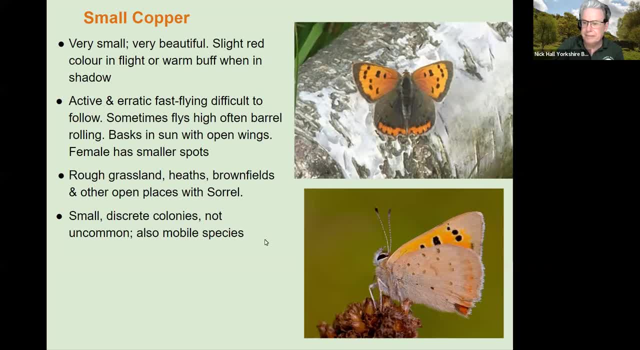 common blues. you know 50, 100 in one area. three generations um may, june, july, july and august, september, october, and the last one tends to be the biggest generation. and then the parasite set in, and it's an egg parasite um, and then the numbers crash um the following year. so our tip is- it's our only- 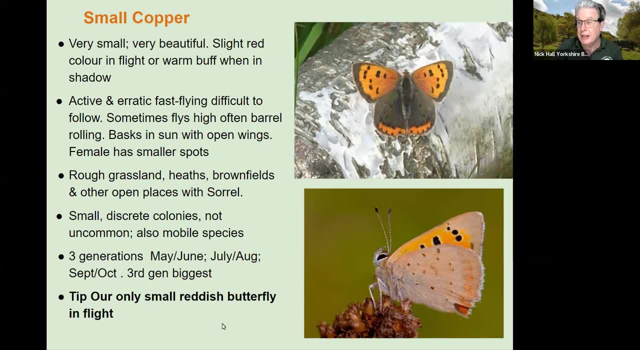 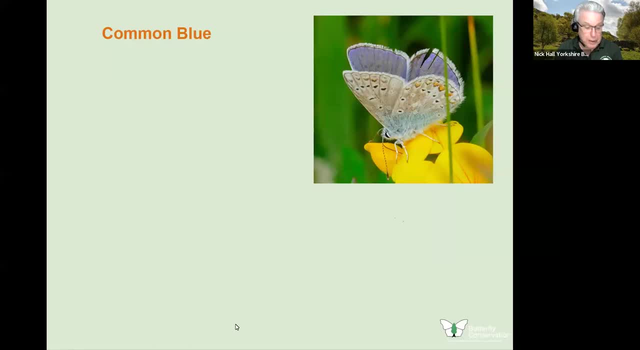 small red butterfly, um, and you see that color in flight. i'm going to hand back to kerry now for the the common blue. excellent, thank you very much, nick. um, another beautiful butterfly. um, so common blue. so males are very conspicuous compared to females, so they have this wonderful bright blue color, um, and you'll often see them flying around looking for a mate. 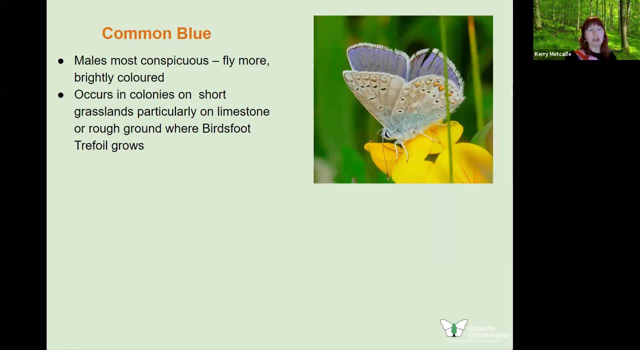 so they occur in colonies and they tend to to hang around on the short grassland, um, so particularly on limestone or rough ground, and again, they're like birds for trefoil. so you're looking for, yeah, short sword areas with with birds for trefoil, or and bare areas, uh, two generations. so the first generation flies in may to june, and then you're. 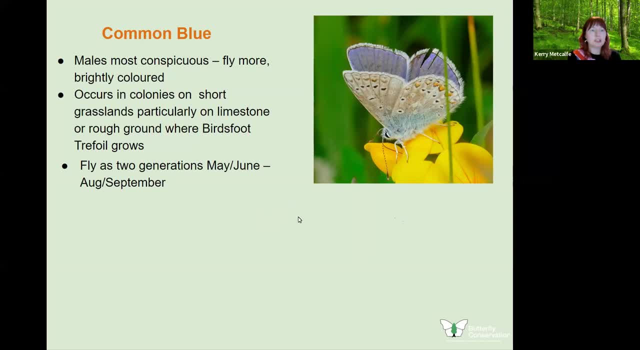 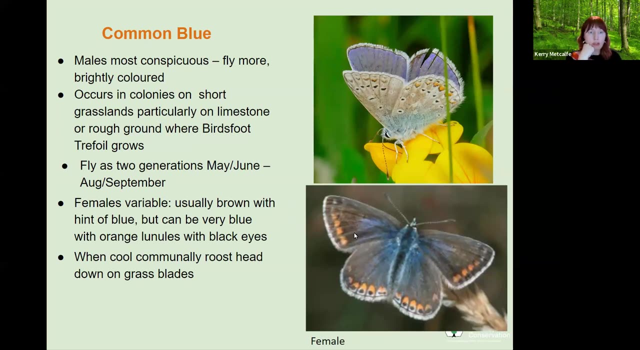 likely to see a fresh generation again in october, december to september time. females tend to be quite variable, so you can. they can be very brown, um, with just a little bit of blue, quite like um the brown argus um. or they can be quite distinctively blue and easy to to tell apart. 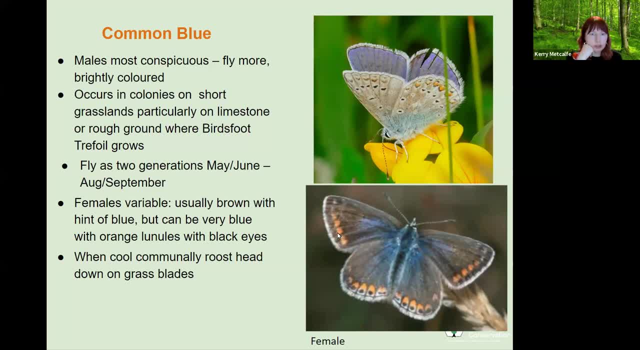 um, they have, like the, the brown argus, they have these orange lanyards. um, so, when you're trying to differentiate between the two, you're really looking for that, that just that hint of blue, um, that that you can, you can use to distinguish. uh, you can also do it by the underside, but it's quite tricky. um, and you're looking for for figures. 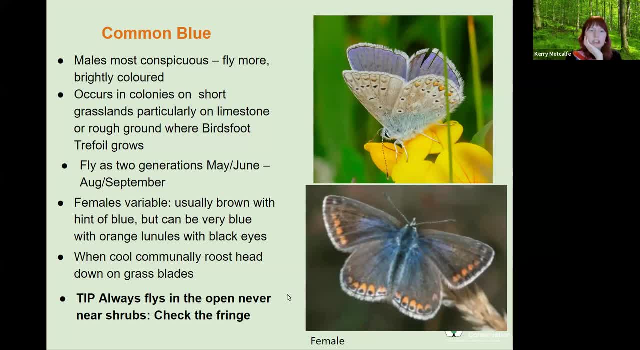 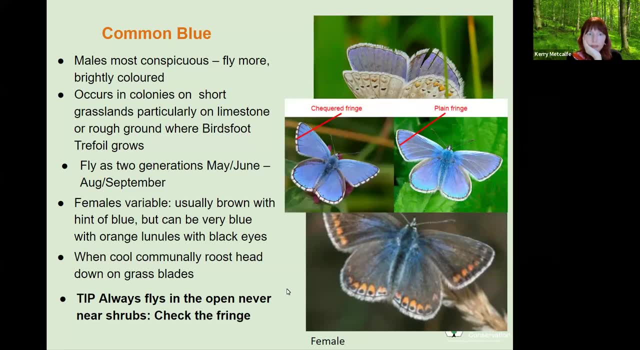 of eights and and spots that aren't there, and i think we'll get on to that in a second. so you might also mistake the common blue male for the holly blue. um, so the difference here is that a holly blue comes out, is it emerges earlier and it prefers to to fly around bushes, trees, shrubs um much higher. 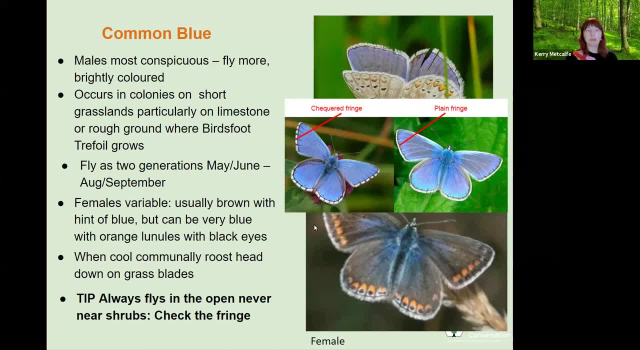 whereas common blue tend to stay lower to the ground and again prefer open grassland with with short sword. so and- and yeah, you can just see on that picture nick's pointing to a holly blue- will have this checkered fringe. so if you're lucky enough to be able to see the holly blue, you can. 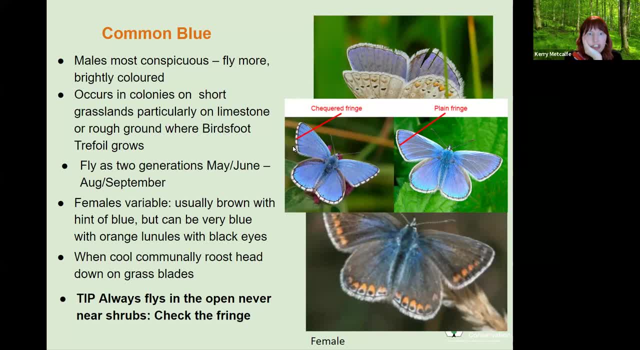 be able to get close enough. um, that's another way to differentiate, but, um, the top tip is: if it's flying around in open grassland, fairly low, it's a common blue. and if it's- if it's hanging around the shrubs and the trees and it's flying a little bit higher, it's likely to be a holly blue, brown. 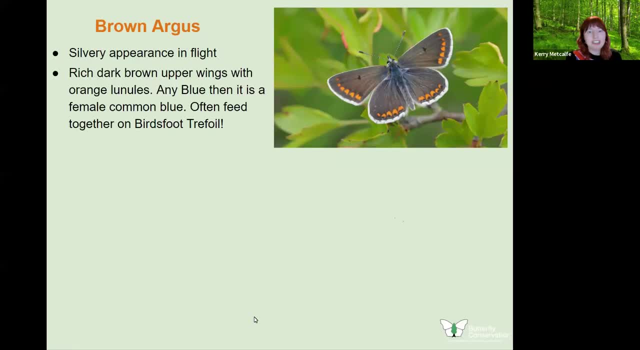 argus, another of my favorite butterflies. um, i think these little things are such beauties, um. so when they're flying about- i think i mentioned earlier in comparison to the digi skipper- they have this um glinty, silvery appearance it's. it's really quite distinctive and quite hard to miss. 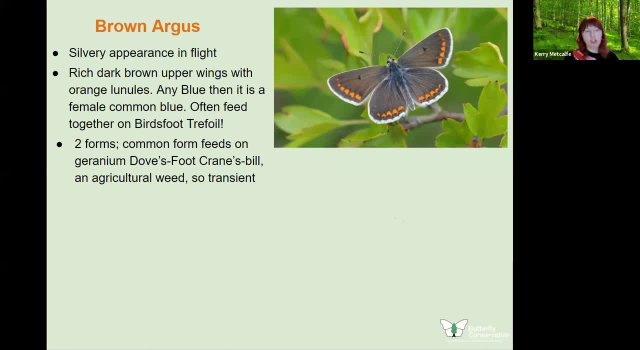 so you'll just see a flutter of of something that looks silvery and and know you've got a brown argus. they have this beautiful, rich, um brown color on the upper wings, and upper- sorry- and lower wings, and then these fantastic orangey lanyards, um, and again you can see there, that's, that's a, a brown. 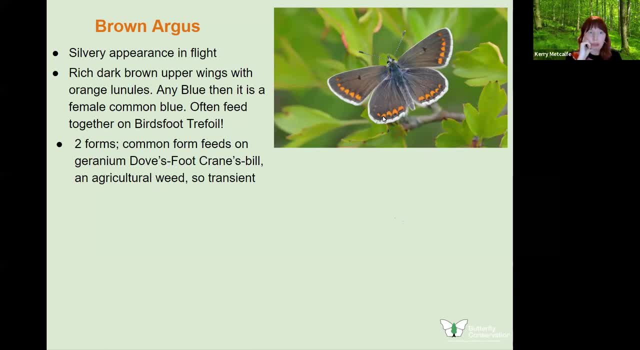 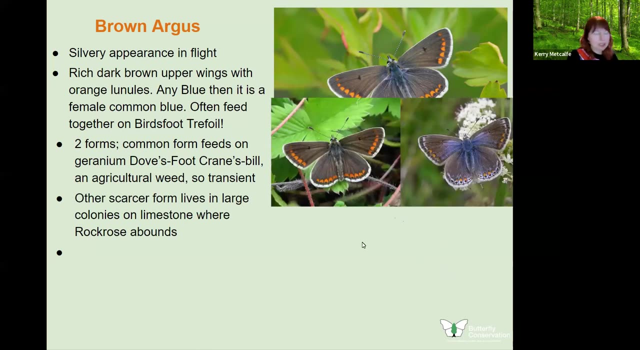 argus and in contrast to to the female common blue, um where, where you just see that hint of blue again- um, they like to hang around on birdsfoot trifles. so just to confuse things a bit, so there are two forms of brown argus, because one would just be far too simple for us to deal with. 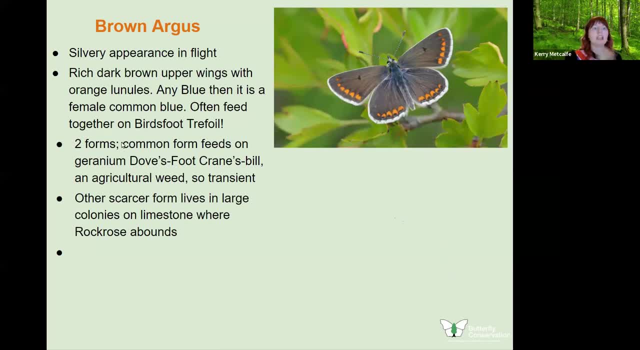 so the common form um, which i think i have on on my uh, transect feeds on geranium. so does foot um and it's transient. and there's a scarcer form that lives in large colonies on limestone where you're likely to find rock crows. 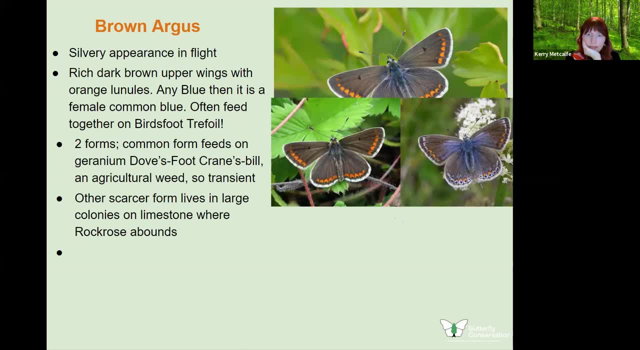 so i think, nick, at the point, because we have quite a rose there, yeah, yours, yours is a rock rose form, um, so i've got the rare form, then you've got the rare form, and most of us, most of us uh have to put up with the common ones. um, we didn't have these um uh, up till probably, uh, 20, 20 years ago. 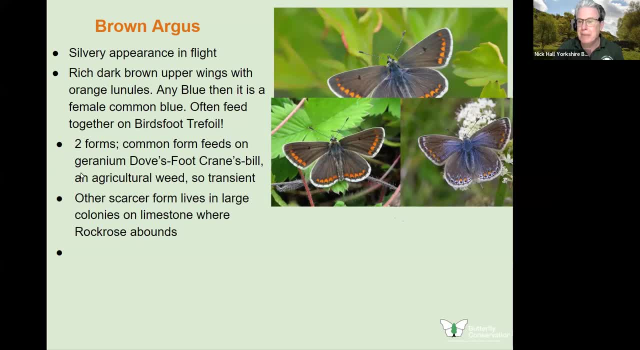 uh, there was only only the scarce form in yorkshire. um, and this, this form, the cranesbill form, has moved in and in some places, uh, you know, across and and and pushed out the, the scarce form. um, they're almost impossible to tell apart. apart from this, they're almost impossible to tell apart. 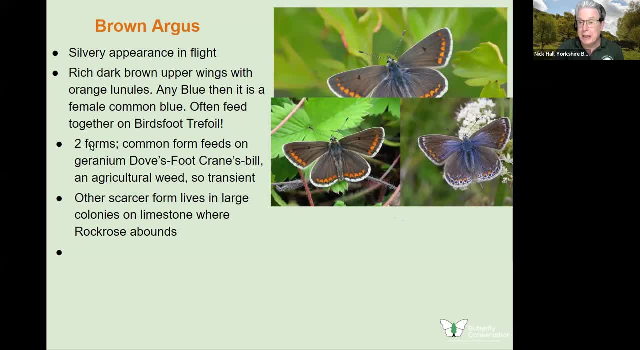 from the food plant and the reason they've become very common is Dovesfoot. Cranesbill is an agricultural weed and it grows in that little strip at the edge of fields which gets sprayed, but that is left bare soil is the perfect place for the Cranesbill to get a hold. 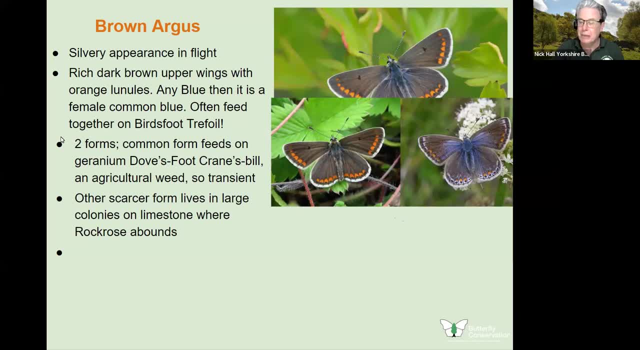 So for that reason, because they're so regularly sprayed with pesticide, the colonies are transient. so some people call it the migratory Brown Argus, while yours it's a Fodden Kerry is the scarcer more it will stick to that one place. yeah, but you also get much larger numbers. 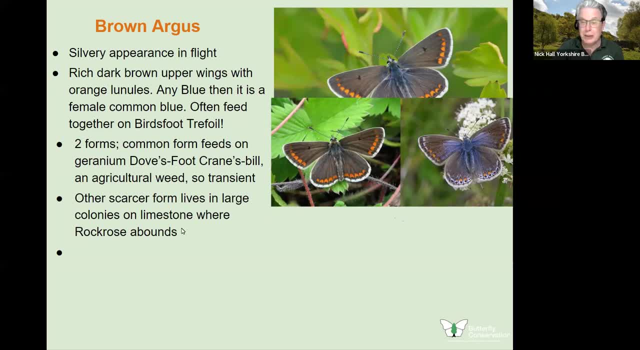 at your. you get hundreds, while we'll just- well, most of us will only see a handful, even if you're not a farmer- At best a handful, most because they spend so much time moving. but they are incredibly common because you see them everywhere, on down, on the, on the lowlands, they are literally everywhere and really 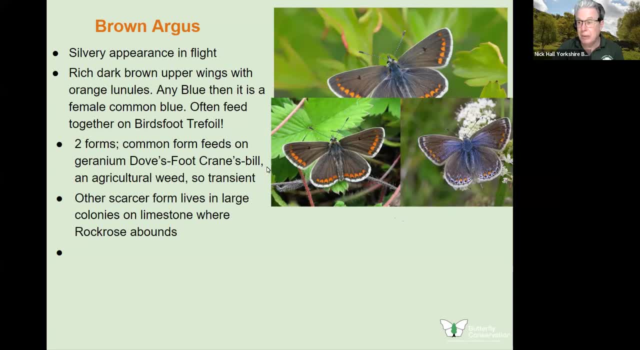 easily confused with, uh, with common blues, mostly because they sit together, they nectar together, they, um, they'll go and sit on birds for travel together, and when you get these two forms here side by side, you begin to see the reason, um, for that confusion. anyway, i've said enough. uh, Kerry, this is your. 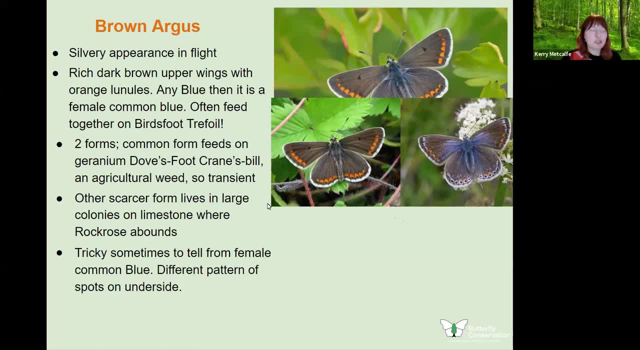 this is your baby i'm going to hand back. no, thank you, you're far, much better at this than me. i thought i'd just do the the lowland uh, um, uh viewpoint of it, which is quite different, probably your viewpoint. yeah, that's great. i should say that we, we aren't trying to. 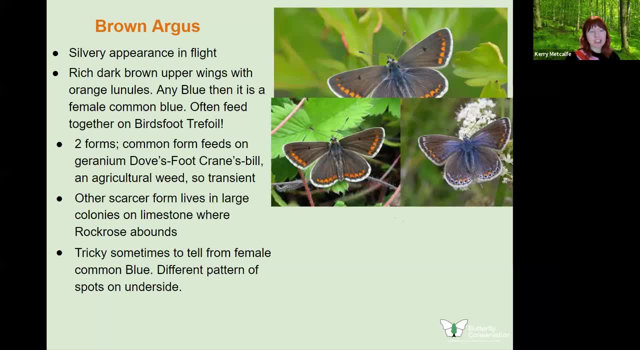 distinguish between the two different types. we're just happy to record Brown Argus, so don't don't worry about that at all. uh, where are we so? yeah, so, as Nick says, your fantastic comparison there, where the Brown Argus on the left definite blue of the female common blue on the right. 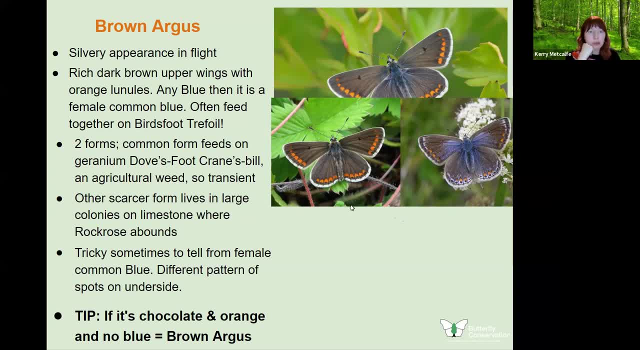 so, yeah, your top tip for for differentiating the Brown Argus from the common blue is: if it's, if it looks like the, the specimen on the left, if it's chocolate and orange- oh, chocolate, orange, um- and has no blue, it's a Brown Argus, and if it's got that hint of blue, it's a female common blue. 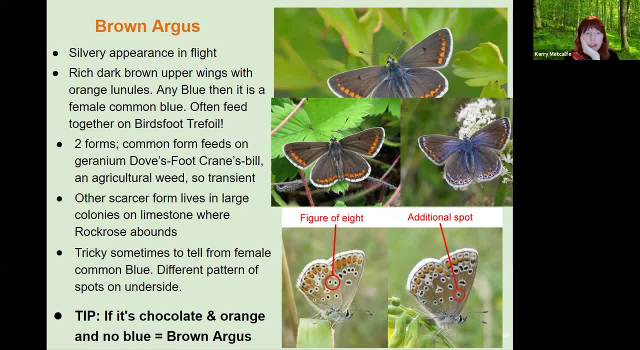 yeah, your other great tip: if you can get close, probably going to want um a camera, and, but if you can get close enough to see the underwing, um really nice way of telling so. on the left you can see circle, that figure of eight and something that Brown Argus have. but 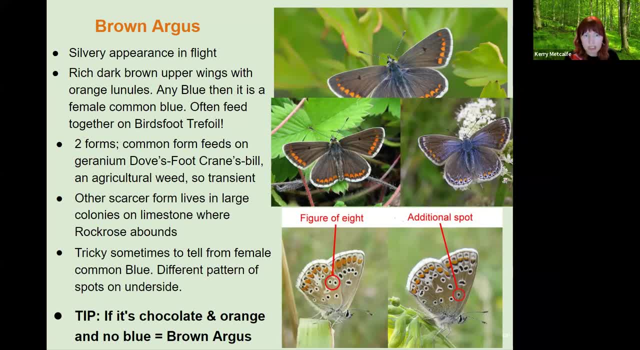 common blue? definitely don't. and then, in contrast, on the right, common, uh, common, yeah, common blue. have this additional uh spot on the base of the forewing sort of- if you like, the butterfly shoulder, um, and Brown Argus, don't have these. yes, you're definitely going to need to. 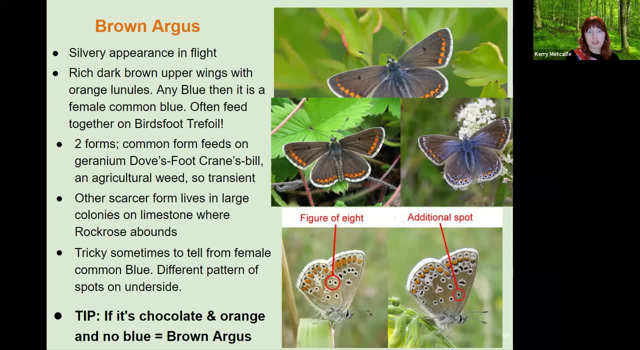 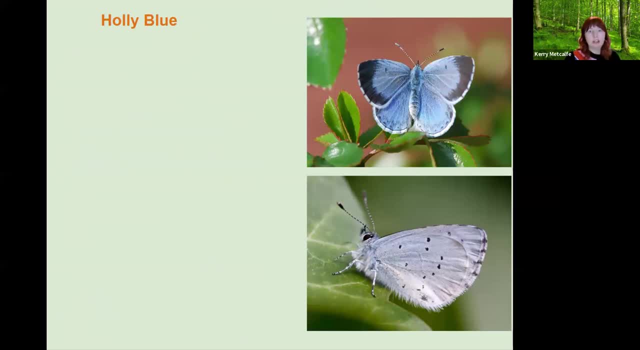 to be very up close and personal with them or taking a photograph and looking at that. and then on the right is Holly blue, another beautiful butterfly, um. so, like I said earlier, you usually see Holly blues fluttering around trees, shrubs and um bushes, so they tend to to be much higher. 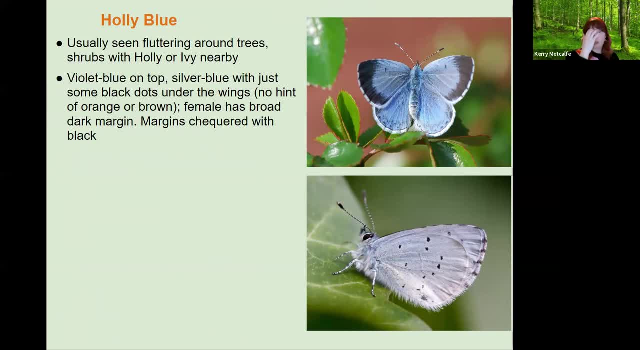 off the ground than their similar common blue, common, yeah, common blue species. so they have this fantastic violet blue um upper wing and on the underwing they've got this, this silvery blue with these small black dots. so quite different to to the common blue and, yeah, as Nick has written here, there's not a hint of orange or brown. so very different from. 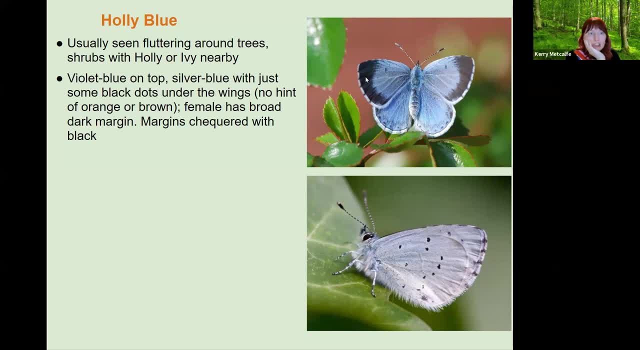 from the female common blue as well. uh, the female has a broad dark margin and, as you can just see, as Nick's pointing out, um, they've got these checkers as well. so really, again, quite distinctive. so they're not colonial, so they're wonder about. you can find them all over the place. 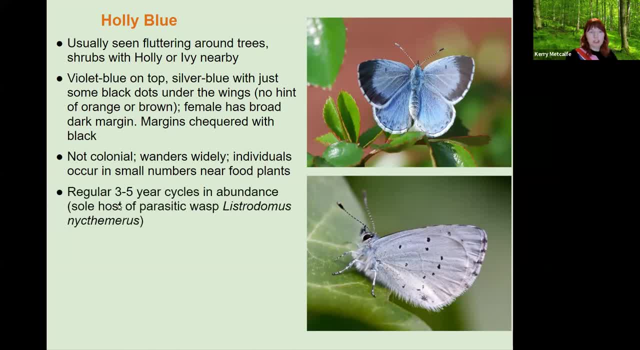 um, and they'll occur in small numbers near their food plants. so they have a regular three to five year cycle and, lucky them, they're the sole host of the parasitic wasp, wasp lystrodomus, nice, thermarus and- yeah, that's my attempt at that- uh, two generations of them. so you'll first see them in a 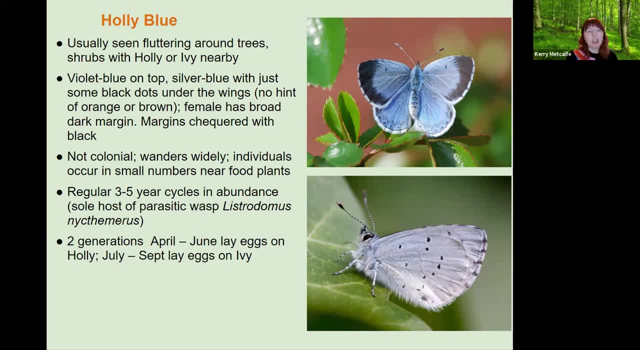 april to june, and then you'll see them in july and september. and so in april to june they'll lay their eggs on holly and, just for a bit of a change, in july to september they'll lay their eggs on ivy. 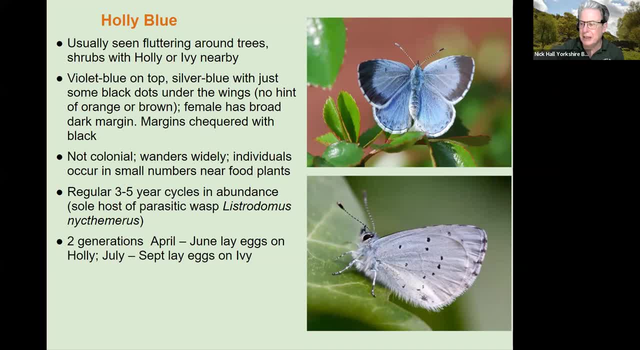 is there a reason for that nick? yeah, it's. it's, um, because the caterpillars bore their bore into the fruit. so they bore into the holly fruit to begin with, and then they bore into the uh, into the ivy fruit, fruit, fruits as they develop. so it's the developing. 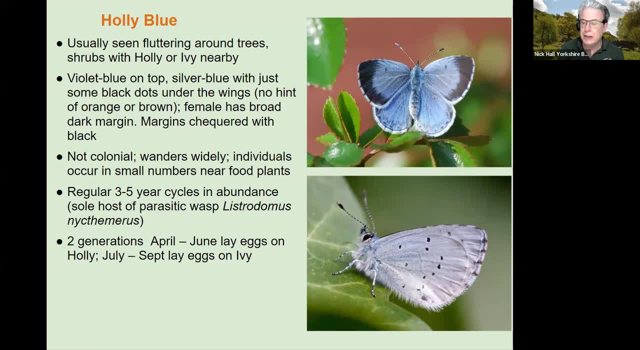 um fruits that they they're interested in. so they do generally lay the eggs just behind the, the bud of the flower or just at the base of the of a fruit. um, yeah, but they can't. they are, they are actually, they do actually. if they can't find the ivy, they just go straight for holly. 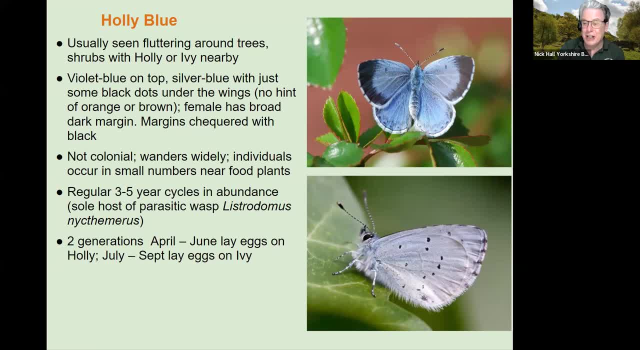 and carry on as normal. um, it's not a strict rule. yeah, it makes sense, doesn't it? really not putting your, your eggs in one basket, or your, um, your larva, um, so they are carried in gardens and parks right next to the center of cities. so this 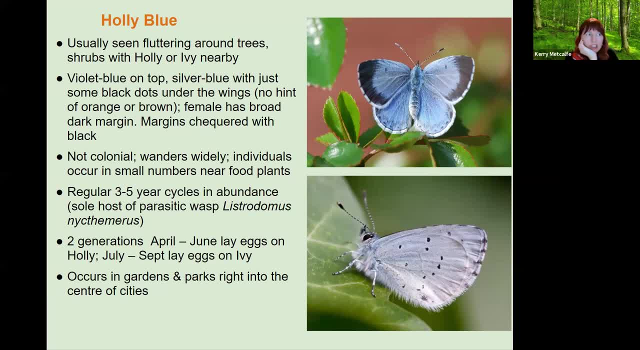 is one i see in in the garden quite a lot, um, which is quite nice, in contrast to to something like the common blue, which i definitely don't see in gardens. so your top tip for for identifying a holly blue is: if it's blue and it's hanging around trees, shrubs and hedges, um, and it's flying higher. 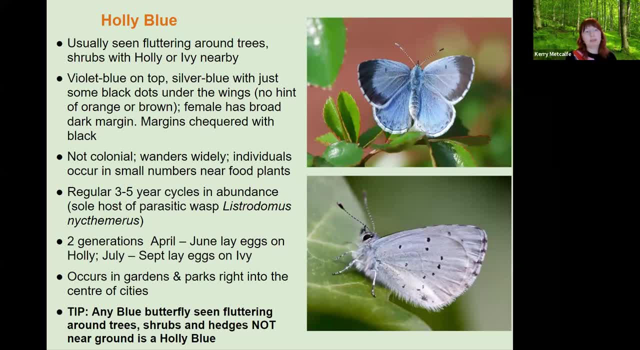 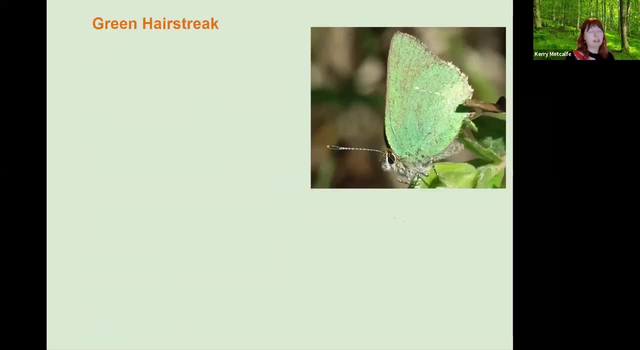 up, it's a holly blue. it's not a holly blue, nothing else. it's a holly blue, and if it's on the ground in open spaces, it's a common blue. right back to nick for another gorgeous butterfly. okay, we're going to go over to the hair streaks. 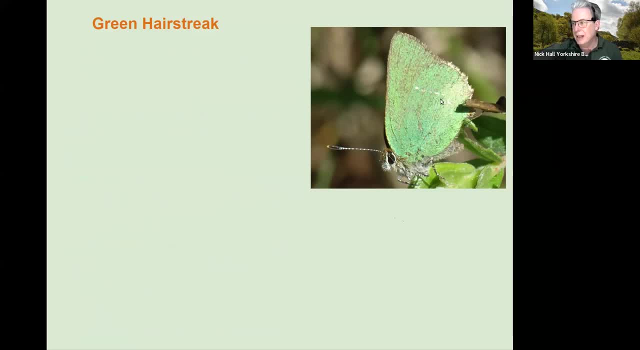 now, and the reason it's called a hair streak- this is the green hair streak- is it has these lines on and there's a lot of butterflies have these lines on their underside and they're usually associated with forest dwellers. but i'll explain a bit more about that later. so the green hair streak- 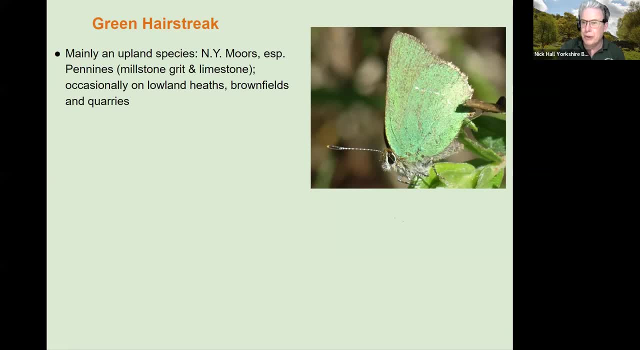 is generally an upland species- north york moors pennines- usually on millstone grits, sometimes on limestone, occasionally on lowland heath and brownfields and sometimes in quarries. it has a very big range of habitats and it feeds on different plants in different habitats. so it 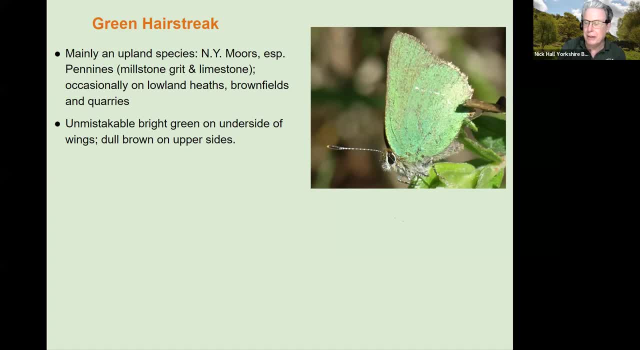 has this unmistakable bright green on the underside, dull brown on the upper side. when it's flying it's very hard to detect and i often, quite often, confuse it with large flies which are also brown. they always rest with their wings closed and show the green. if you can find the the green on the green plant, it's very 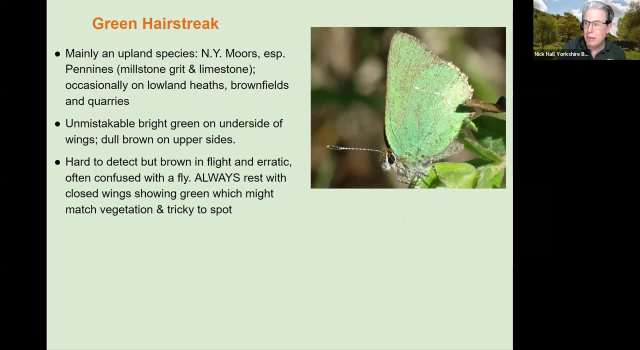 clever camouflage and almost exact match for the vegetarian vegetation. so if it lands it is a tricky one to spot. you have to rely on that brown when it's flying to see it. fortunately the males will come up because they're quite territorial, while females are searching for. 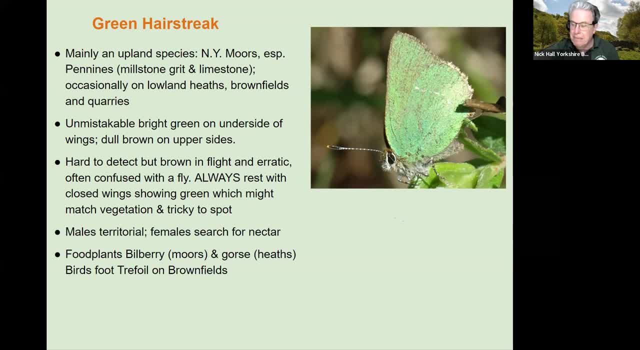 nectar. the food plants bilberry, which is probably its most common food on the moors gorses, sometimes heathers, and on the lowland it tends to be bridgefoot truffle and it's summery in the south west to the north east of the south east, and it's a big 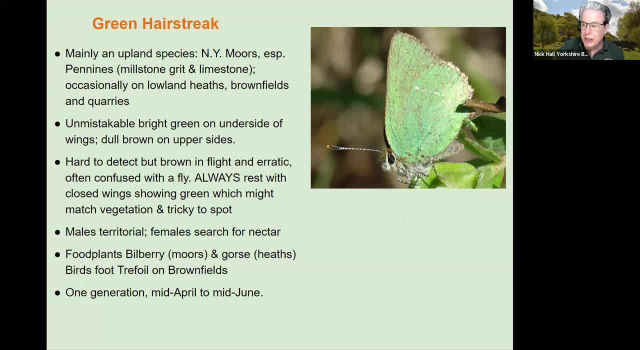 bred farm whose lowland um, um, um- and i'm going to go to the one generation- mid april, mid june first. one's already been seen outside leeds this year and i think the first ones were seen at opli chavin is the hotspot if you want to see one. you haven't seen one before: opli chavin- small brown erratic flyer and always near its food plant. so we move on now to the aboric food plant plant as a food plant product is a food plant. a food plant is a plant. you can grow fruits, wild foods and other vegetables on a family farm. or food product is a food plant. a food plant is a food plant, a free, endlessly and free fire food etc. which you can find. the food plant for food. you can grill your food. 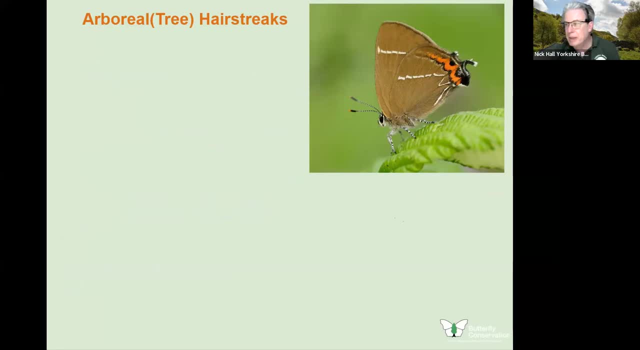 arboreal or the tree hair streaks. These are the most poorly recorded- no, not poorly recorded, just under-recorded- butterfly. They're surprisingly common but we don't often see them, And this particular one, the white letter hair streak. 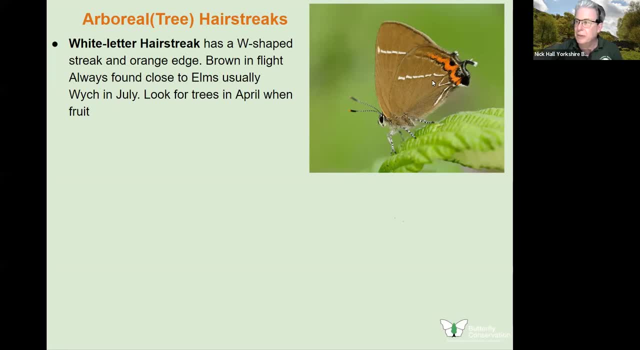 is regarded as scarce And it has this wonderful W shape right here which gives it its name of the white letter, And it has a streak of orange along the edge. here Browning flight is always found, always found close to elms. 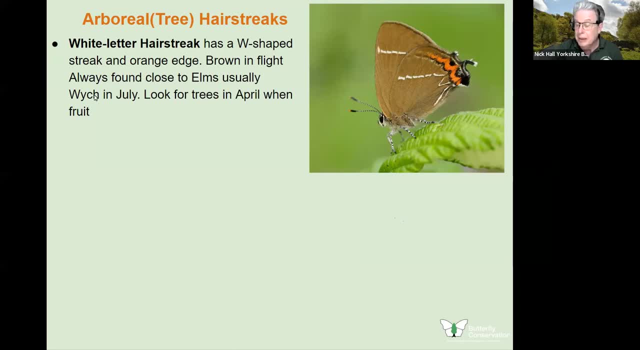 and it's usually witch elm which is still quite common in Yorkshire. Everybody thinks that the elm trees all disappeared with Dutch elm disease. It's not true. Elm trees, in my opinion, are indestructible If they die of Dutch elm. 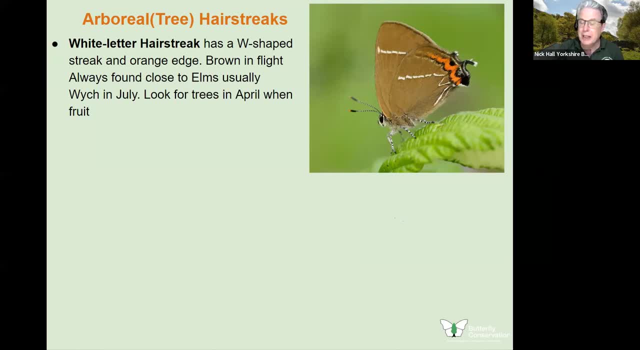 they send up a shoot from the bottom. A year or so later, a new tree grows. It'll grow to 20, 30 foot, which is big enough for it to produce fruit, at which point the hair streaks move in. 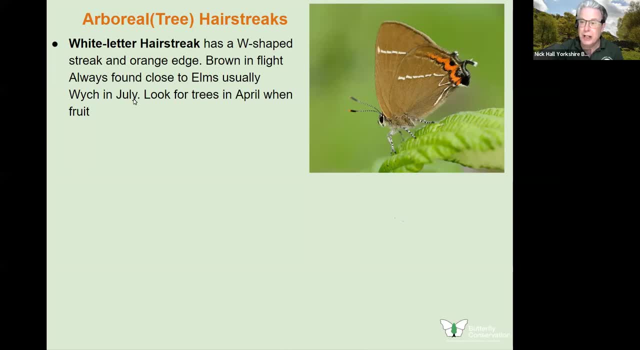 And then, a few years later, it will die off with the Dutch elm as soon as the beetle gets in. When's the best time to find them? Well, the best time to find them is right now. These next two weeks are the perfect time. 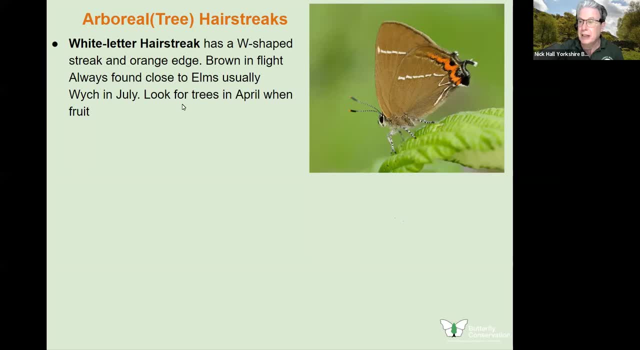 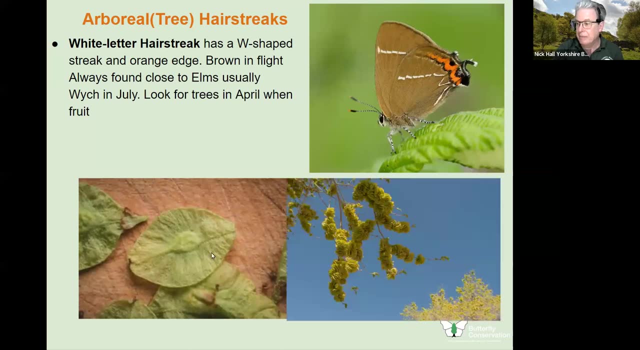 to find the elm trees, And the reason is it's fruiting And these are actually the fruit of the elm, And what's it look like? It's quite characteristic, the elm tree when it's in fruit, because it has no leaves. 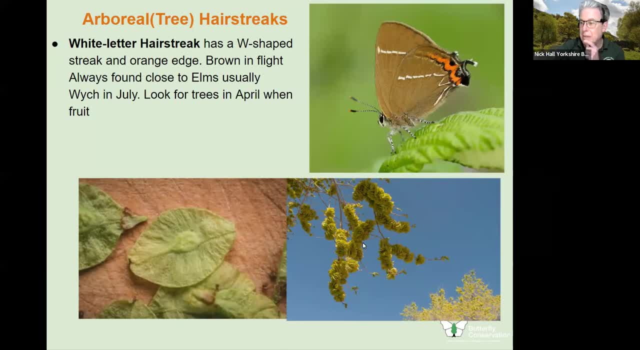 like most trees, at the moment They have no leaves, but it fruits before it has leaves And it's this kind of silvery green. It shines in the sun. So if you're walking in woodland, watch out, because you'll see with the wind. 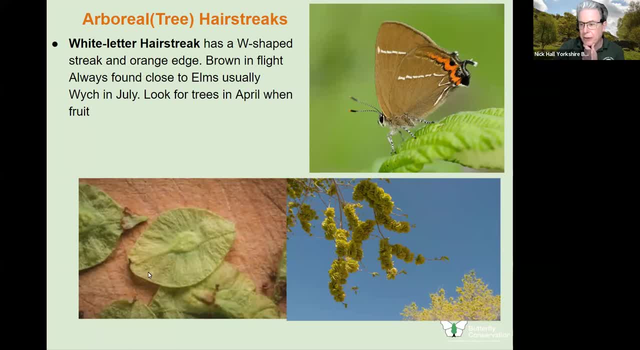 which we've had today. these will be lying on the floor of the woodland track And if you look up, you should be able to spot these chaps which are the semosis, the fruiting bodies of the elm, And they look. 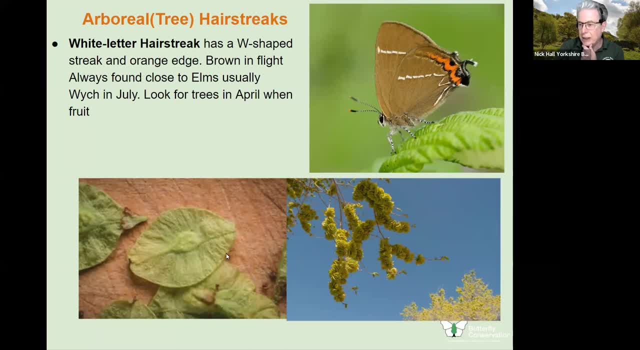 this is typical of a elm. They shine in the sun- This silvery, very pale green colour- And if you mark them in your head now when you're on your transect, then there's always that chance when you come back in July. 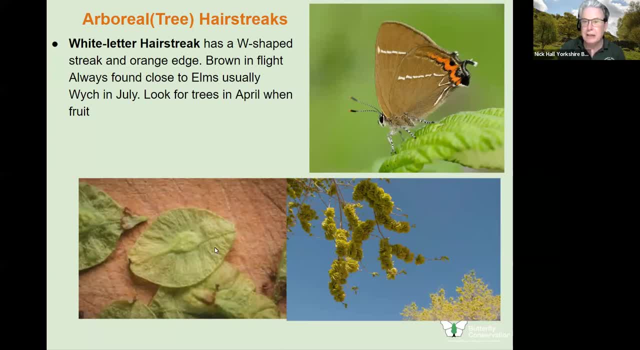 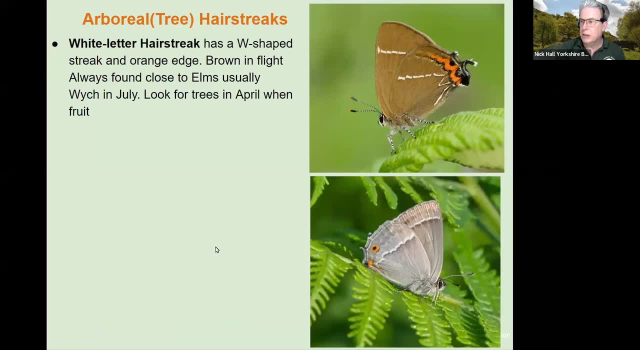 when it flies, of seeing the insect. So the other hair streak is the purple. That is the purple hair streak, Also very common, can be very numerous, And the way you tell it is it has this silver underside also with that white streak. 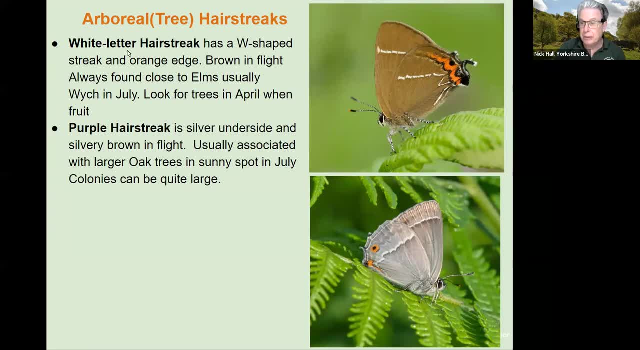 Now almost universally amongst our arboreal tree butterflies have this streak And we'll see a few more If you go through this presentation. there's a few more of them They have and the reason they do it is like wartime, when you're doing some camouflage on ships, et cetera. 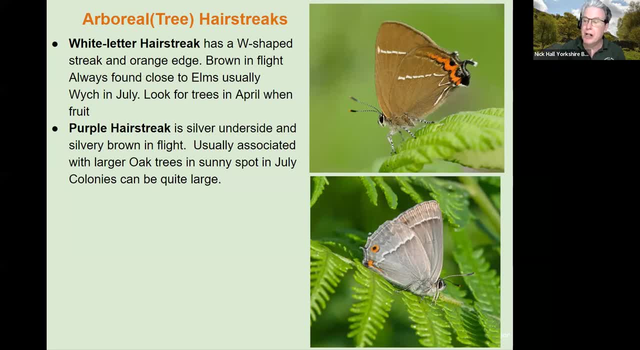 you want to break up your shape When you're in partial shadow. if you have a big stripe across you, you are breaking up your outline So it confuses the enemy. Like ship camouflage, you disrupt how an insect sees you by breaking it up. 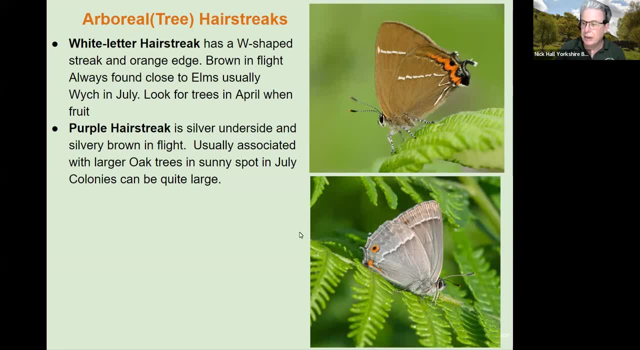 by having hard lines across Almost every large oak tree. if it's in a sunny spot and you're in July, you will find them if you go at the right time of day. Both species are tricky to spot because they tend to be quite erratic in their flight. 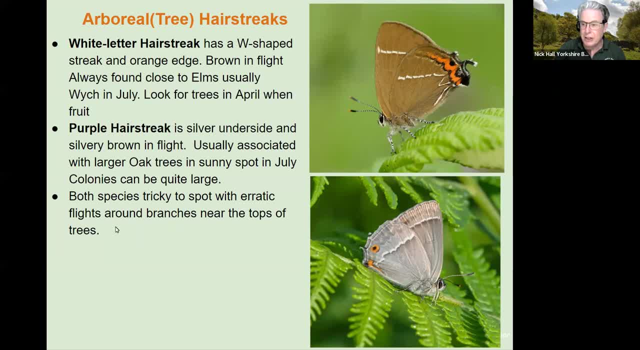 And it's generally very short flights around the tops of the branches, near the tops of trees. They also tend to peak in their activity in the evening, ie when we're finished our transects they come out to play. Both species feed on honeydew. 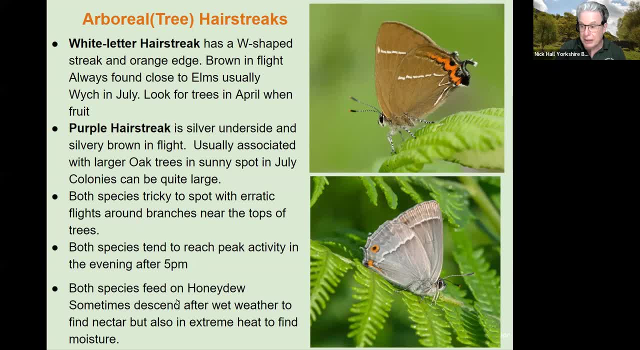 And the main time you'll see them- which is surprising- is after wet weather, when all the nectar, when they come down to nectar because the rain has washed all the honeydew off the leaves So they're forced to come down to find food. 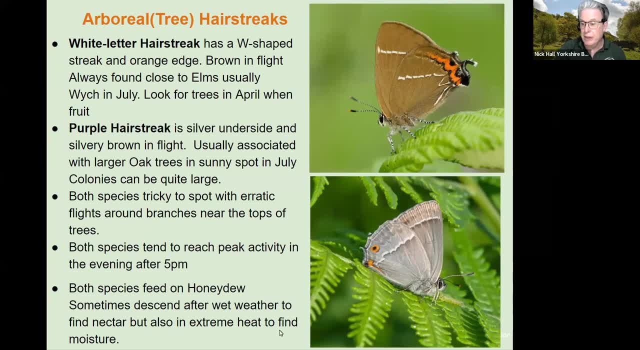 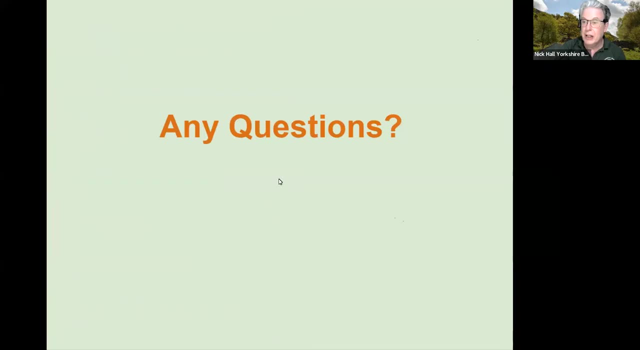 But also- and this is very common- when it's extremely hot. you'll find them on the ground, and that's quite often where you find a colony is you find a white-letter hair streak existing on the ground. So that's the end of hair streaks. 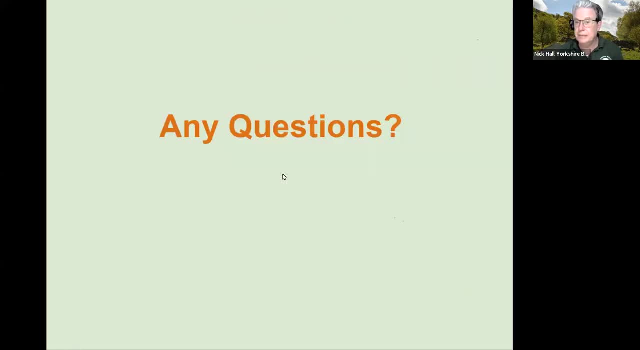 Any questions? So, Nick, I'm just conscious of time. It's 25 to nine. so, yeah, We need to speed up. Yeah, Just We're through the vanessids and then we can do a bit on the. 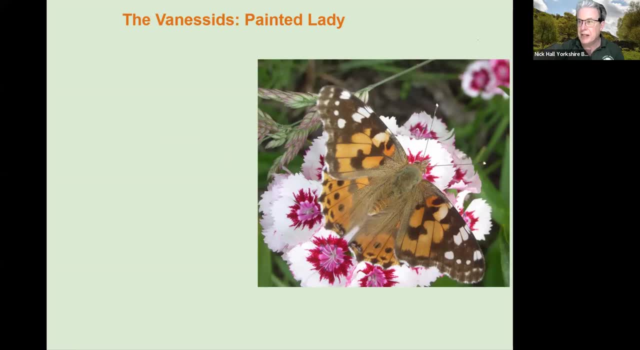 On the moss, The transect parameters and the moss. Well, the vanessids are pretty easy because they're big and they're beautiful and they're huge and they're coloured Painted Lady will be familiar to many people. 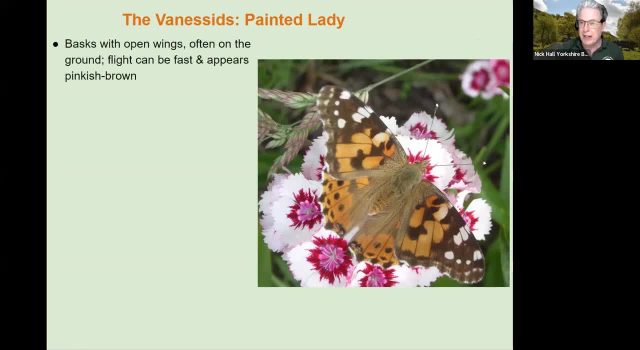 Always busts with its wings open. It's very fast. It's this lovely pinkish, salmon-y, orangey-brown colour. Some people call them the pale pink, pale pilgrims. They do come in very large numbers some years. 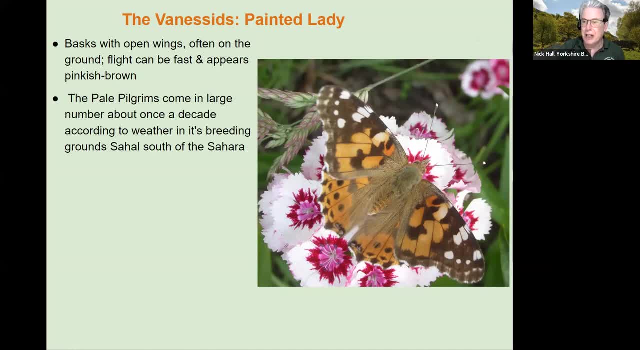 about once a decade. They're coming up from south of the Sahara. Everybody thought they used to breed in North Africa. They don't. They go way down south, right down to the West African coast. They can't survive in our winter. 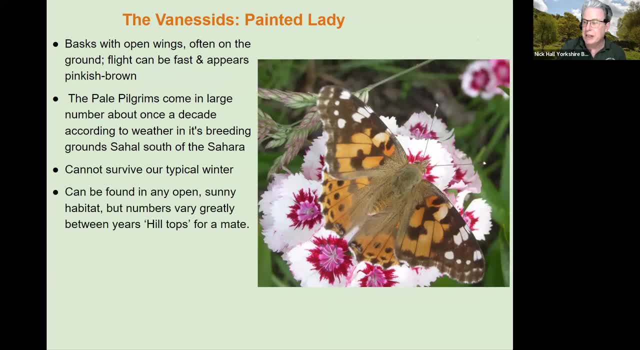 Can be found in open, sunny places. They do like hill-topping, waiting to find a mate. People at the tops of hills tend to see them more than people at the bottom. First migrants arrive in spring, So if it's very large, very fast. 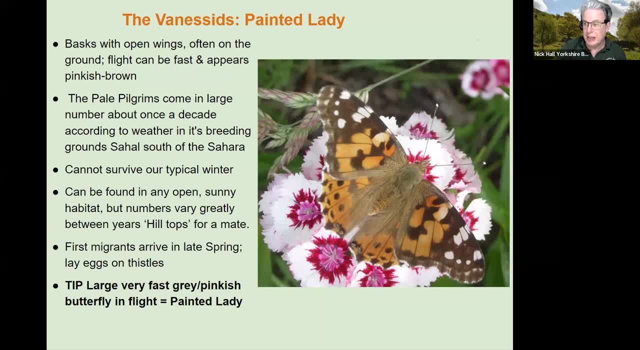 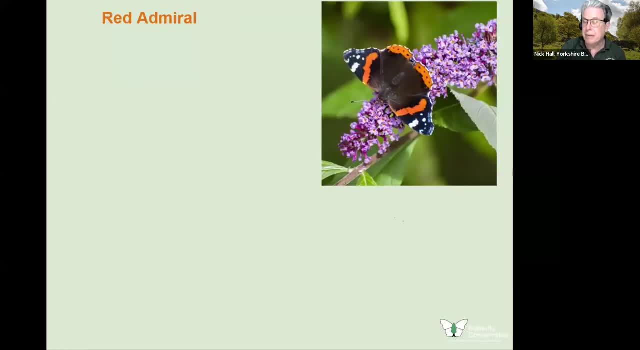 and pinkish in flight. the chances are it's a Painted Lady. Speed and size. pink, Red Admiral. Okay, Very characteristic that red stripe on our buddleia bushes. It's a migrant, Very strong flyer, A large butterfly. 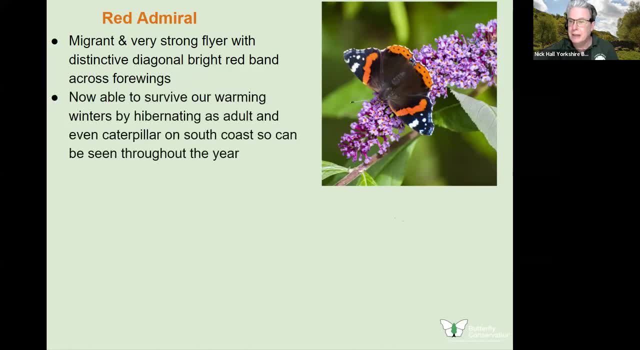 Distinctive diagonal red band across those four wings. those four wings, uh. it's now able to survive our warming winters by hibernating, as an adult and even as a caterpillar. on the south coast it now overwinters, actually as a caterpillar. 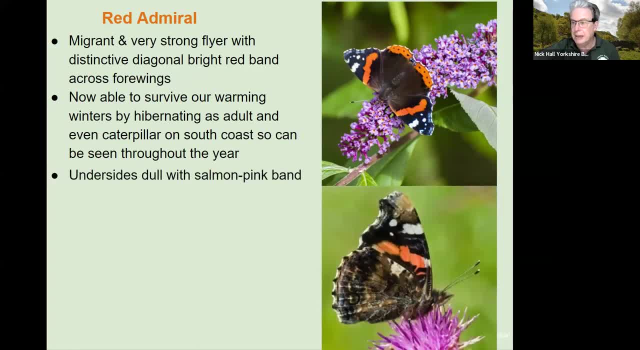 undersides are dull with a salmon pink bar. um, they say it's on common nettle and you quite often will see them on your, on your. uh, if there's a lot of them around, you'll see leaf tents in the tops of nettles like they've woven the the nettle together um. spring migration comes from europe. 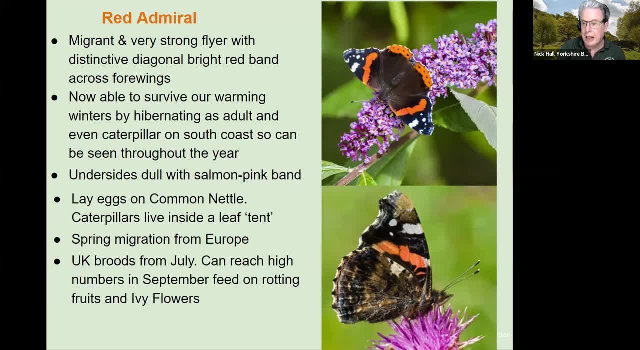 most of the most of the ones we get are european um and the brood really builds up. when we get to july, numbers really begin to build up with migrants and you see them on rotting fruit and ivy flowers when we get to september. so in flight, how you tell them it's large? 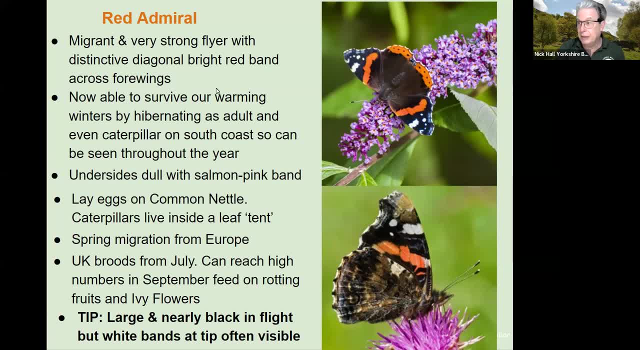 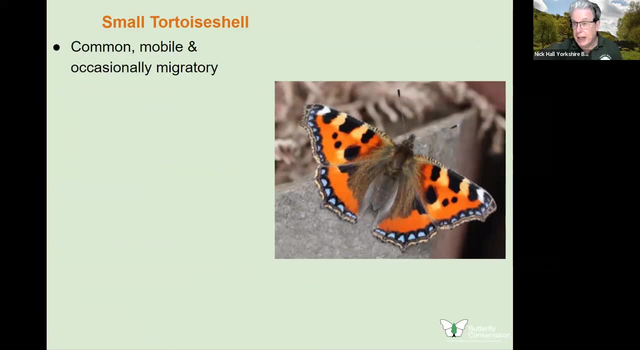 it's nearly black in flight, but those white bands here you can see as it flies usually and that's how you tell it from other species, small tortoiseshells you'll be familiar with, um, it's common mobile and it is also a migrant- can almost be seen any month of the year over. 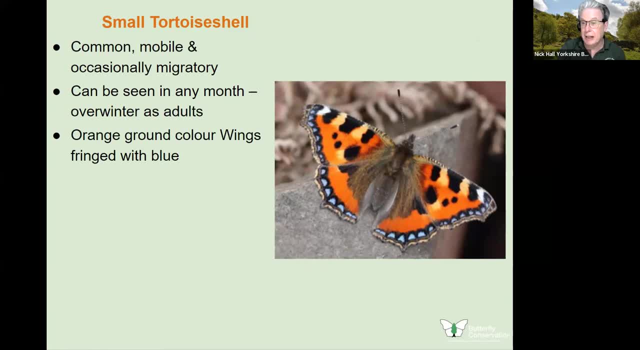 adults. the important bit is the ground color is orange and the fringe is blue. so it has the black and yellow stripes along the top side of its wing, quite characteristic of a tortoiseshell um, and the hibernations begin to breed around about now. they are looking to lay eggs around this week and the next couple of weeks they make communal larval. 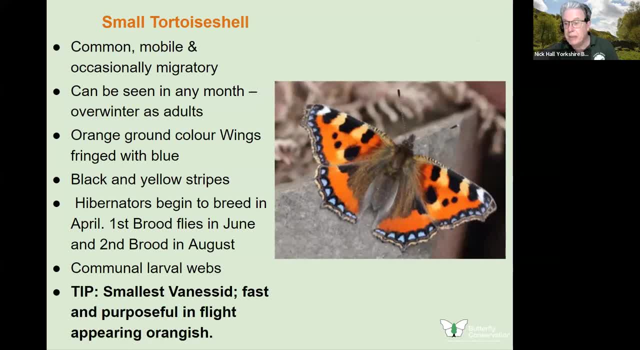 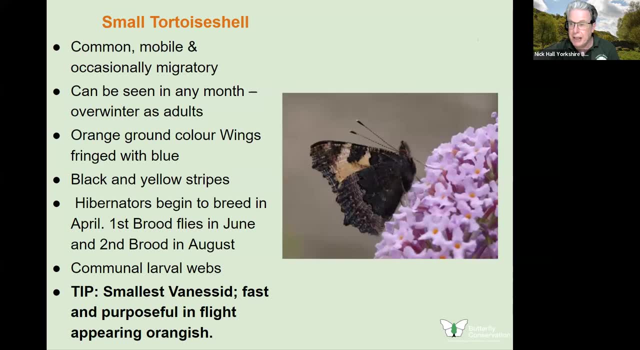 webs, so it's the smallest of all our venusid species. it's very fast, purposeful flight and appears orangish in flight. that's how you tell it. that's the underside dark because it's a hibernator, so it gives it some protection when it finds a resting spot on the tree trunk, etc. all the. 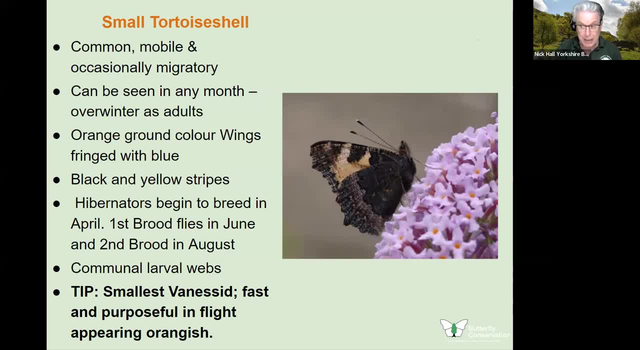 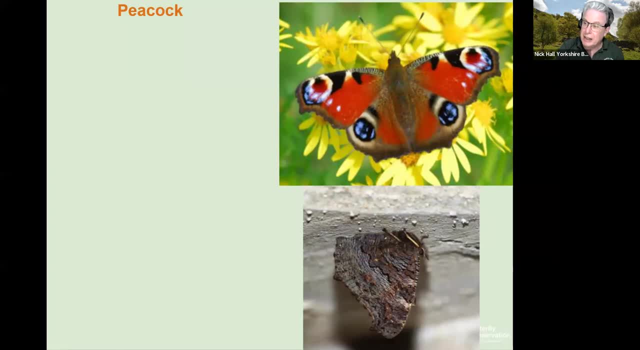 hibernators tend to share that unless you're brimstone, you go on the backside of an ivy or a bramble peacock. it's got those characteristic big eyes, and for good reasons. it's very common. particularly woodlands can be seen on the sky. 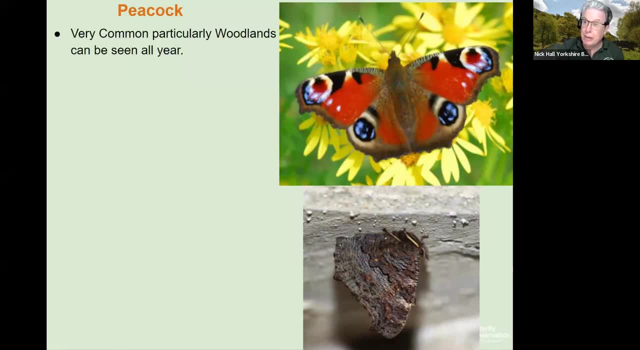 and for good reasons. it's very common. particularly woodlands can be seen on the sky, and for good reasons. it's very common. particularly woodlands can be seen on the sky, can be seen a large part through the through the year has this black underside camouflage: large eye spots resemble the eyes of an owl. if you look very closely that is an owl's eye. 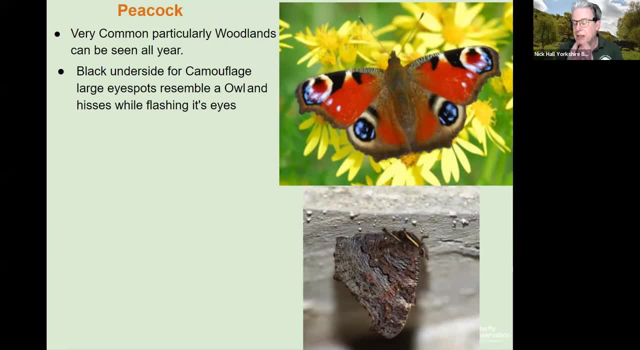 it also flashes. so when it's, when it's, you see the, the underwings there, when it's challenged, it will open its wings very suddenly, like so, when it opens it wing wings, it hisses. it's our only hissing butterfly and basically, is making it as if i'm an owl. 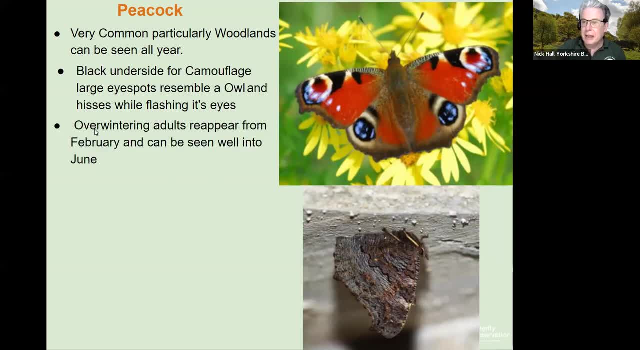 so the overwintering adults appear in february, but those same butterflies can be seen all the way into june. they're very long-lived black larvae with white dots, live in webs and they begin to emerge to the new generation in late july and they feed up and hibernate- uh, sometimes very quickly, which. 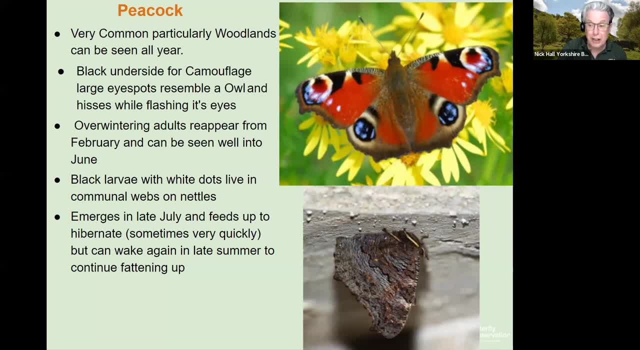 is confusing because you might only see them for a week or less in very hot weather, because they feed up very quickly and then hibernate. they can wake again, but if it's very warm weather they tend not to um. but if they do come out they'll continue to fatten up ready for winter. uh, experiencing. 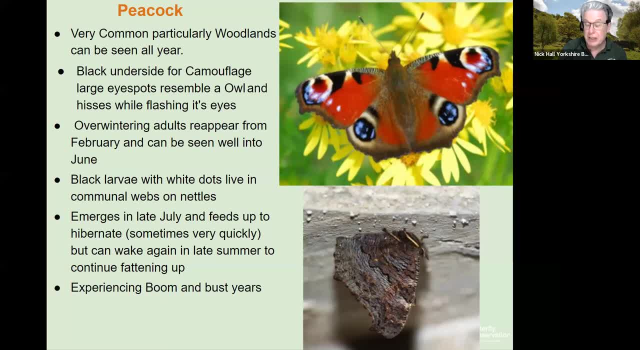 booms and busts. we've just gone through a bust year, but it's good to see that numbers this year are very much better. so coming out of hibernation this year is actually good numbers, better than previous years. so if it's a strong flyer, a large dark butterfly, which is very slightly that maroon. 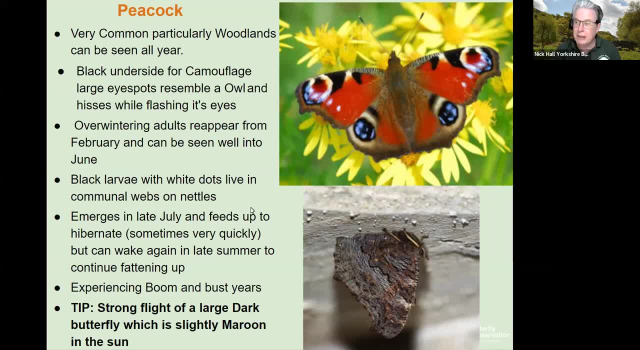 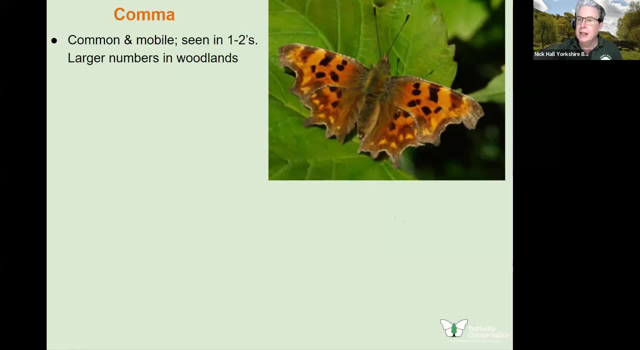 color. when it's in the sun, you know you're looking at a peacock. even if you can't see the eyes, you'll see that maroon color. so the comma. more complicated species, fascinating species. it's common mobile, usually seen in ones and twos, uh, but you find larger numbers in in our woodlands and it has these unique ragged edges. 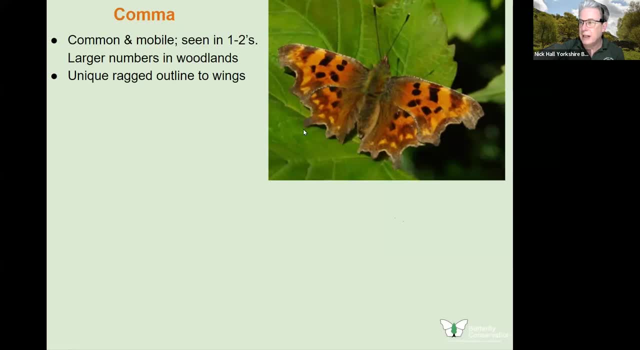 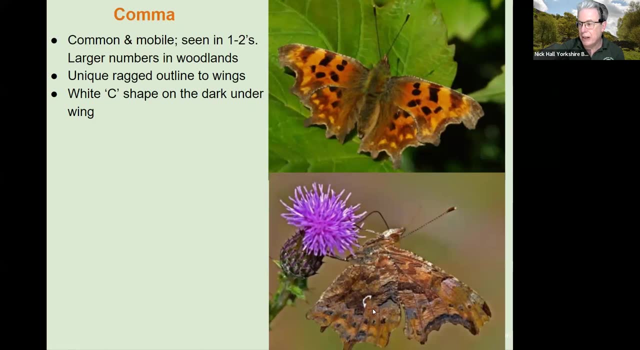 look so tatty, but that is on purpose, because it's camouflage and the other side has this characteristic comma mark the c on the bottom, the underside wing. It emerges in the spring and males are extremely territorial. They'll come up and greet you, So if you go into their territory. 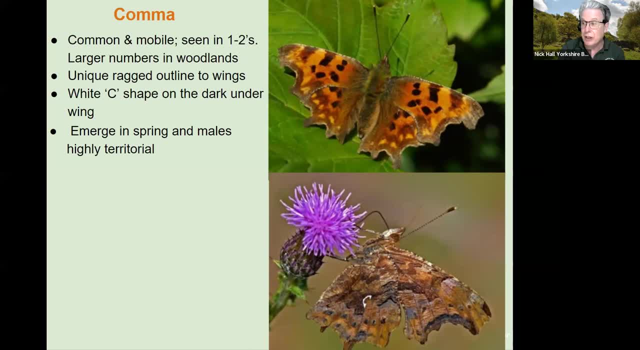 they see you, they'll instantly fly. So it gives you a clue: If one flies, usually two or three more will fly And suddenly you've got a small cloud of them. as they jostle, They use nettles, but they also use elms. 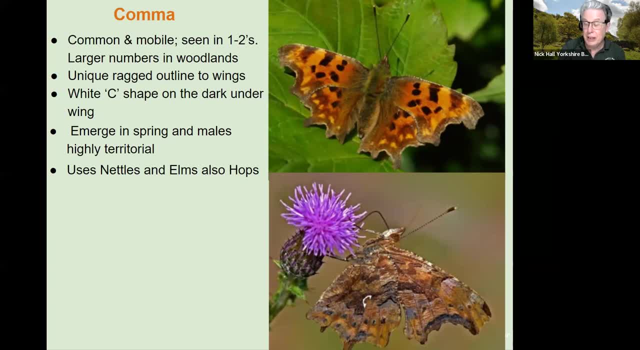 So if you have a lot of elms in your woodland, you'll see more commas The summer. adults emerge in early June. but they have two forms, which is interesting. They have a pale form that breeds and they also have a regular. 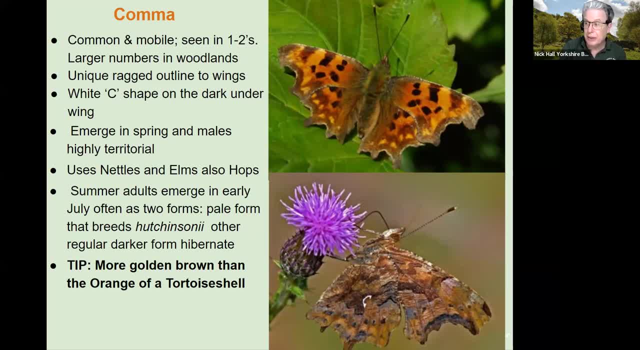 like the one on the picture there, which goes on and hibernates but doesn't breed. So it tends to be more golden brown than orange of tortoiseshell. So in flight, that's the way to tell them apart- It's not orange. 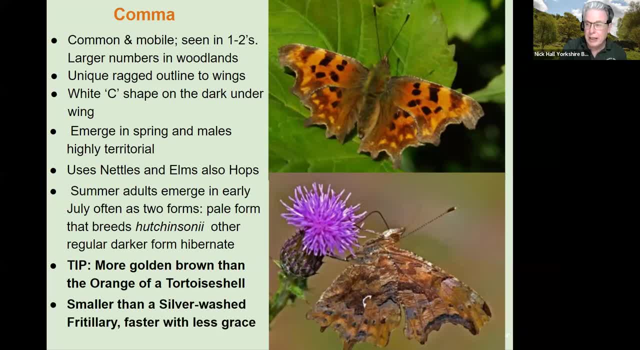 It's just a more brownie orange. It's also get you also get them confused with silverwashed fritillaries, which I have a lot of on my particular transect, But the comma is much smaller and it's generally a lot faster. 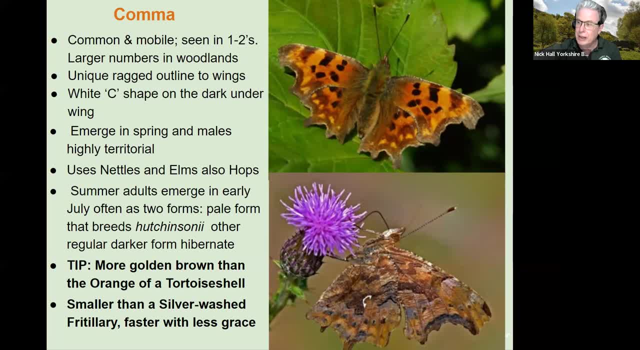 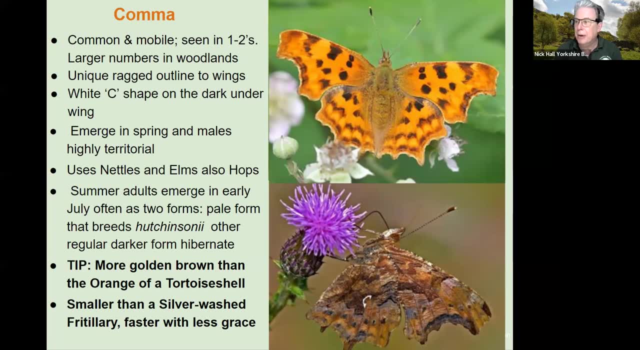 and it has no grace at all, unlike the silverwashed. So here's the second form. It's called Hutchinsoni and it's pale And not many people. we'll record them, but you can see here that the raggedness is much less. 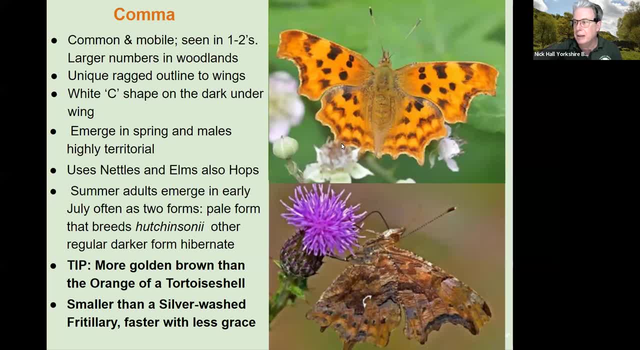 The spots are smaller and the color is brighter And, depending on temperatures, you get more or less of these. It's kind of insurance policy: If it's a warm beginning of summer is warm, they produce more of these, which then leads to another generation. 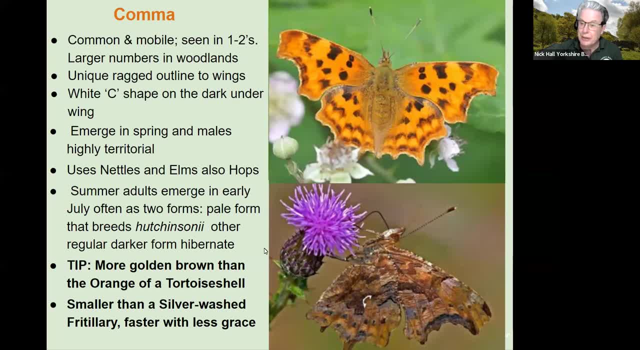 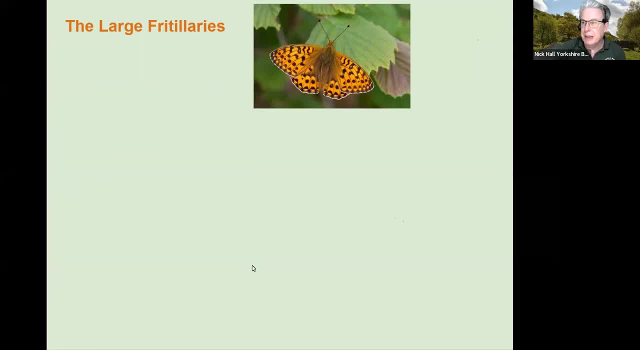 So numbers build up. So it's kind of an insurance policy, Yeah. So let's move on to the last bit. You'll be glad to hear Large fritillaries. So this is the dark green, It's our most widespread fritillary. 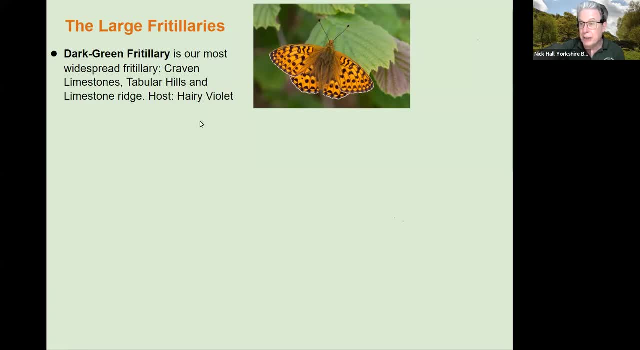 but it's quite restricted in its habitat to limestones, Craven limestones, Ingleborough, that kind of area settle Tabular Hills, which is the south side of the North York Moors and the limestone ridge like. 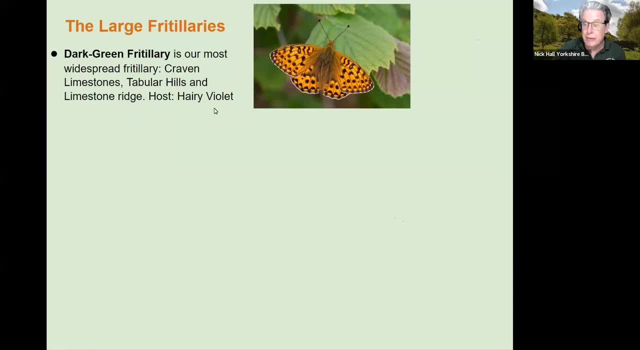 like a brocadelle, is well known And its host, generally on the calcareous grasslands, which is its preference, is hairy violet. So it's large, rapid, graceful flight. Hind wings have this characteristic silver spots on a green background. 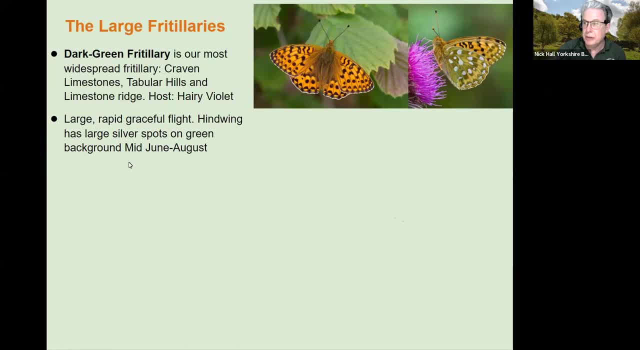 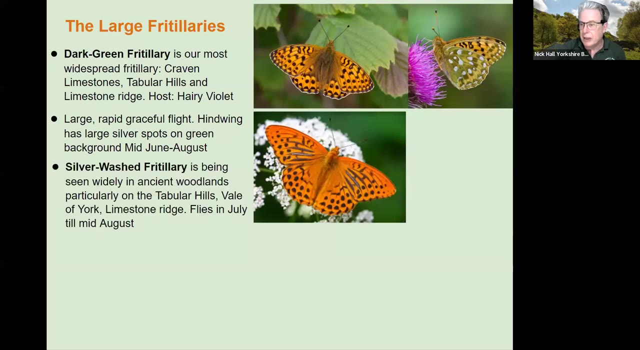 which is how it gets its name. It flies from mid-June into August. You'll still see it flying end of August just on the edge of the North York, on the edge of the North York Moors. So this is my specialist species. 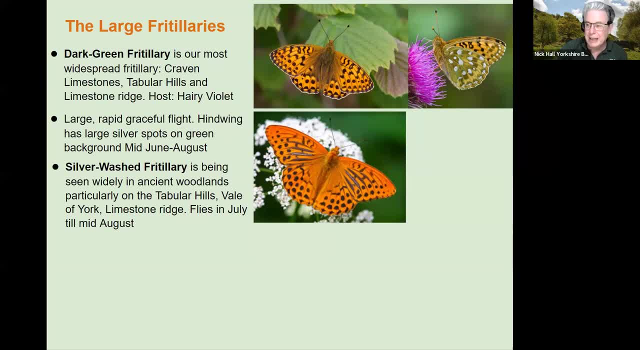 the civil wash fritillary. It first arrived in Yorkshire about 2018 and bred up to quite big numbers in 2019 and has spread out from there and now to inhabit quite a lot of our ancient woodlands, particularly along Tabular Hills. 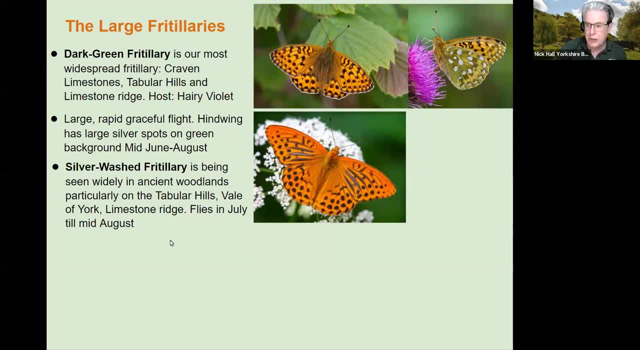 Vale of York. limestone ridge Flies from beginning of July to about the end of the year. at the middle of August It's our biggest butterfly. a beautiful thing Hard to describe as anything. It's a long range wonder as well. 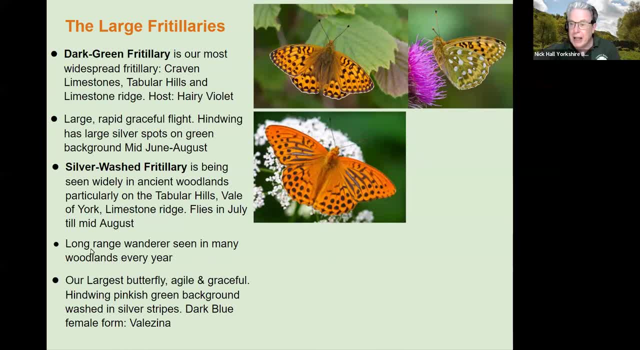 And you can see them If you have a woodland. usually you'll get a visit, one visit per year. If you're lucky, you get to see that It's agile and graceful. It's difficult to describe, but if you look at the underside, 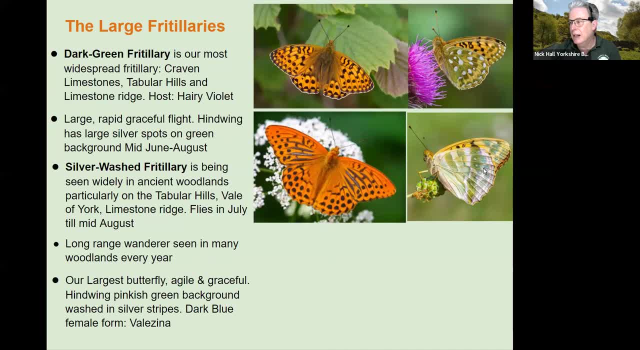 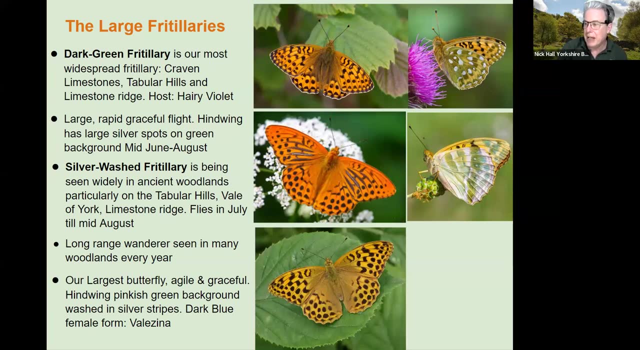 they have this pinkish underside with green and this silver flash, the characteristic of a woodland butterfly, the silver flash. And this is the female, which is quite different from the male because the spots are bigger and the colour is quite drab. 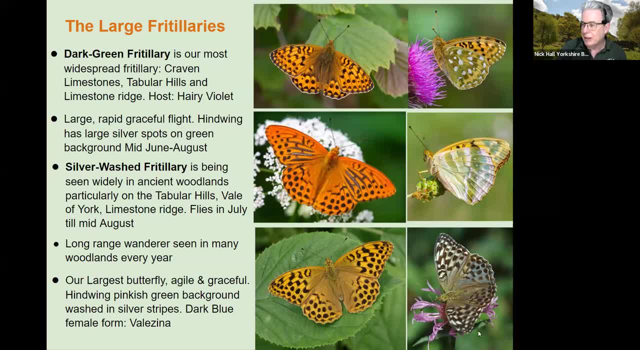 But then, if you're very lucky, you get to see this little devil. It's called Valasina, which is a blue, blue-green form of the female, Quite rare But in big colonies, and which we have quite a number now in Yorkshire. 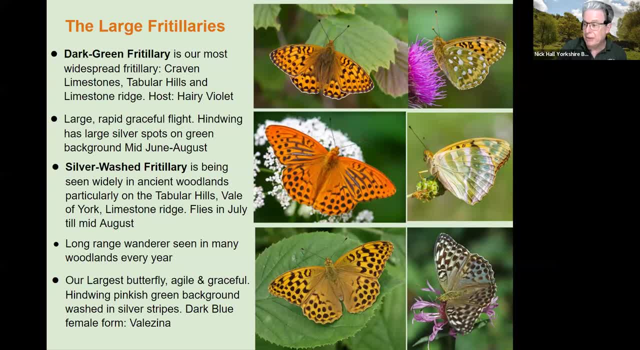 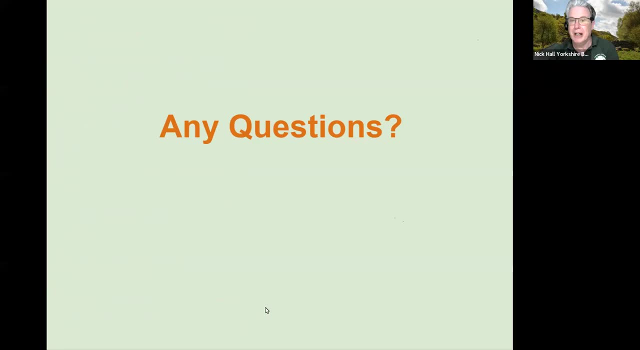 you do get odd ones appear A beautiful thing If you ever come across one. these are big, big, big butterflies. These are small plate size. They are quite enormous, So I'll finish there. Ask for any more questions on butterflies. 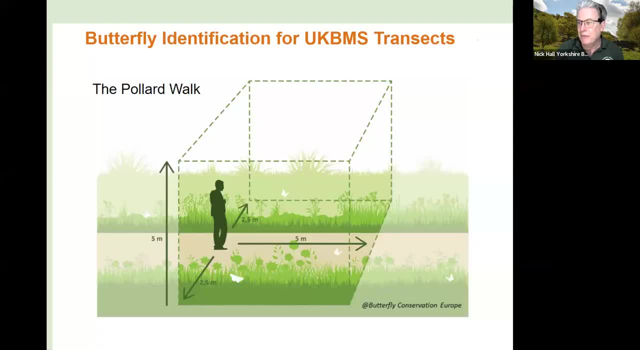 Good, Right, we'll move on And we're just very rapidly going to go through butterfly identification and the transect walk, Because I know there's quite a few beginners here tonight And I think we just need to run through the polar walk. 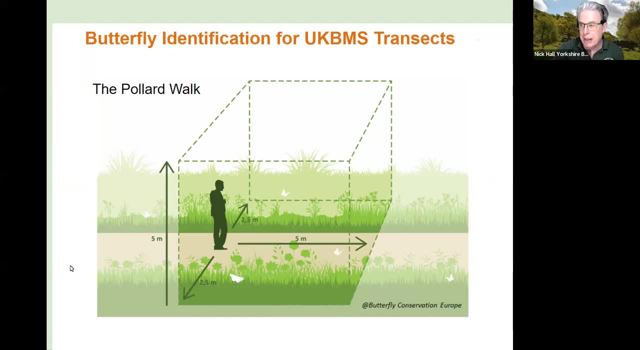 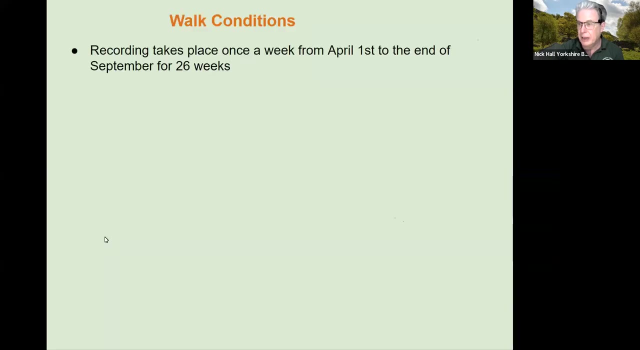 which is the basis of our UK BMS transects. So basically, we're counting everything that enters this five metre square in front of us. So not behind us, only in front of us. So we're going to start with a butterfly. The first thing we got to remember is: 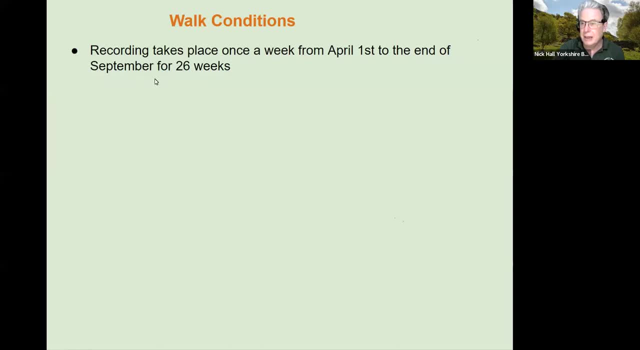 the recording takes place once a week from 1st of April to end of September, So 26 weeks. Any other day to record is interesting but will not be used. Week one always starts 1st of April, Doesn't matter what day of the week it is. 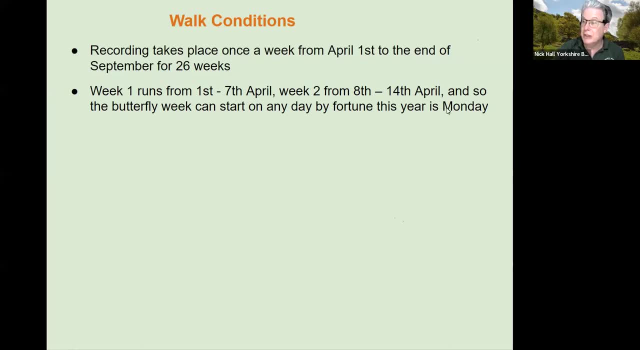 It can be a Wednesday, It can be a Sunday This week. it's handy because it starts on a Monday. So that's the butterfly week- Monday and Sunday this week, and the weather forecast. I know it's been diabolical today, but the weather forecast is a bit more hopeful for. 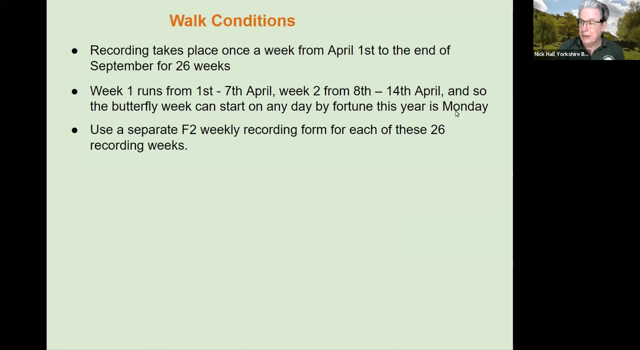 Saturday and Sunday this weekend. so if you can find some time to do your first walk this weekend, that would be great. we use a separate, what they call the f2 weekly recording form. each of these 26 recorded weeks. I'll show you what that looks like in a minute. if you miss a week, keep going, don't worry about it. 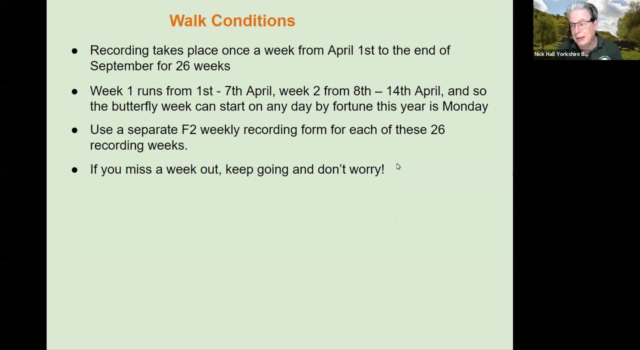 particularly this time of the year, April, it is very difficult, we can't, it's impossible to find the walk conditions. transit counts should ideally be done between 1045 and 345. between the hours 10 o'clock and 4 o'clock is okay. in summer, mornings are generally better than afternoons, especially when it's hot. 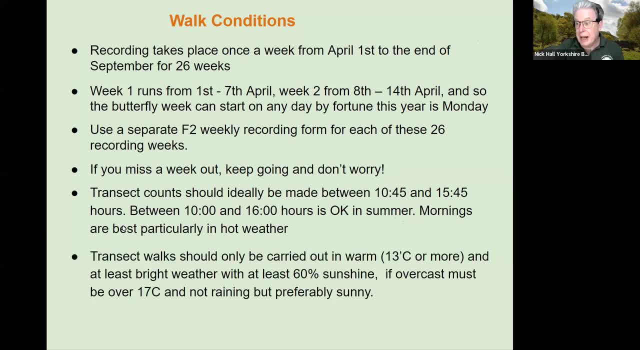 weather transect should always be carried out when it's warm, so it needs to be at least 13 degrees or more. this is the important bit. this is why we become obsessed with the weather forecasts. we're looking for that and at least some brightness, so at least 60% sunshine. 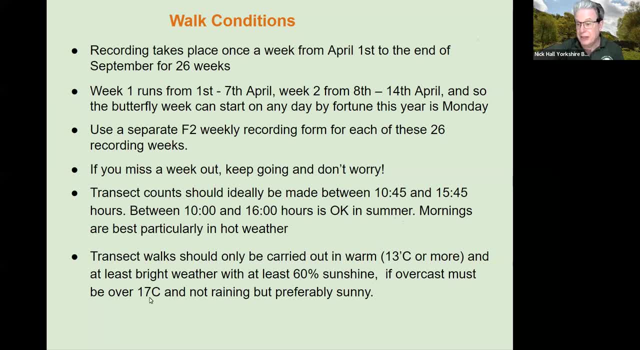 if it's overcast it must be over 17 degrees and not raining, preferably always, preferably sunny. I know it's very difficult and I take my hat off to all you walkers that one little sentence gives us the most maximum grief of any kind of occupation. I think just getting those conditions even in July last year, those conditions. 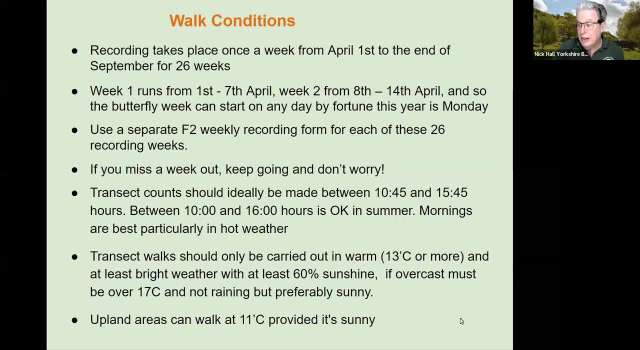 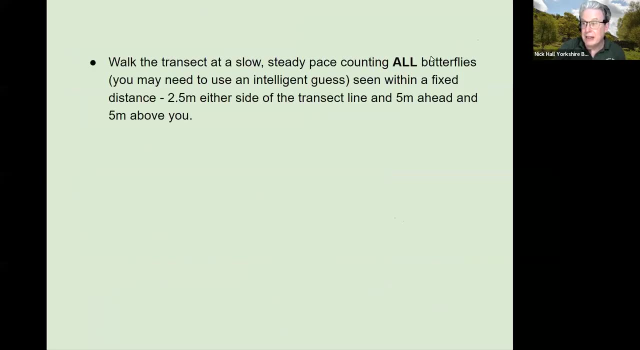 were difficult. now there is a bit of flexibility, so for upland areas you can walk at 11 degrees C, C, providing it's sunny. So we walk our transect at a slow, steady pace. We're counting all butterflies, all butterflies, And, as I've said, you may need to use an intelligent guess. 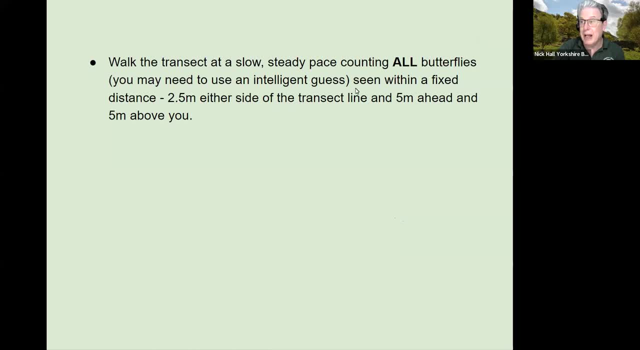 but we need to get something for everything you see, And it's within that distance: Two and a half meters either side, five meter ahead and five meter above us. We always follow the exact same route each time we make the walk And we know any sections we can't walk. 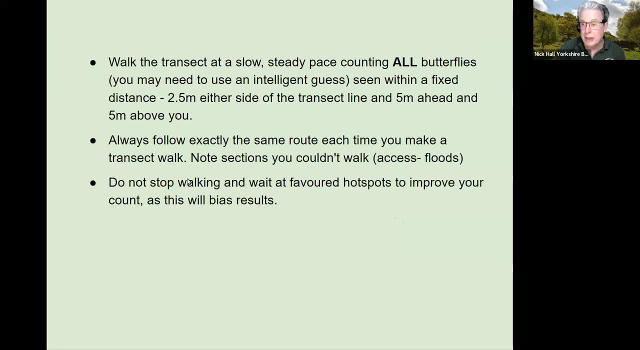 because of access issues, floods, et cetera. we make a note of those. We don't stop walking and we definitely don't wait at our favorite spots to improve our chances. That will bias your results, And the whole idea of this is it's a reproducible result. 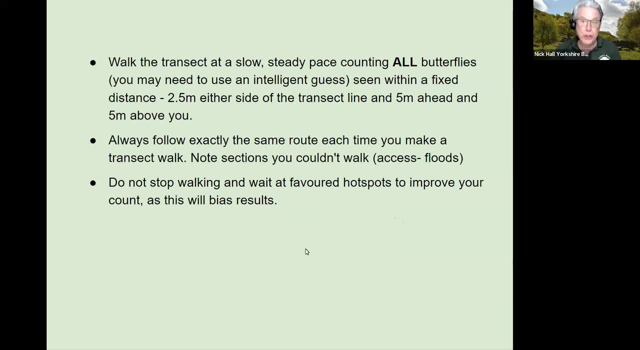 If I walk behind you, I should get the same numbers as you do, And when I have accidentally followed one of my walkers, it, surprisingly, is close within two or three butterflies, which I find absolutely amazing. So for each section we record butterfly numbers. 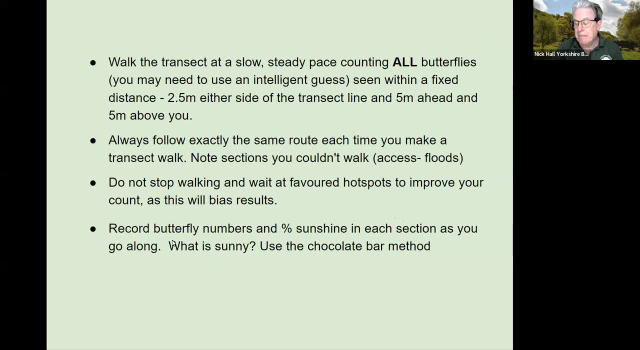 and the percentage sunshine, And how we do that. what is sunny? Well, you can use what we call the chocolate bar method. So if we divide in our head the section into 10, segments of a chocolate every time we walk through a sunny part, 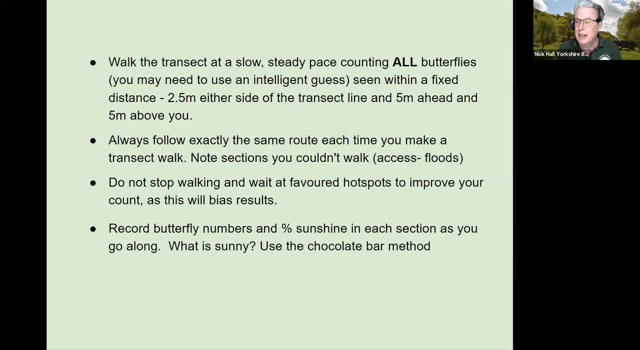 we eat one section of our chocolate. When we get to the end of the section, we just note how many pieces of chocolate we've eaten. It's kind of a way of getting your head around how we do it. Most people do it in the head. 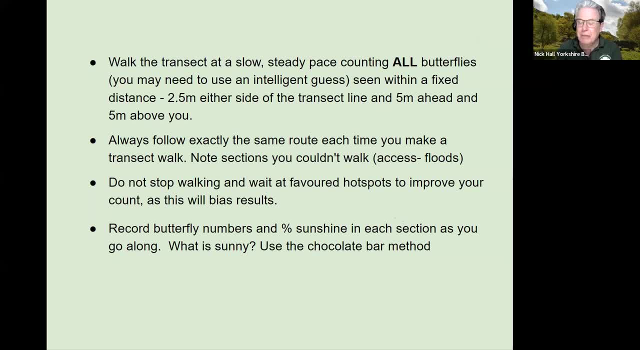 as a kind of running percentage. We're not asking for extreme accuracy, but make sure you get a figure for it Every section. Wind speed: Less critical. the low wind speeds gets critical when you've got wind speeds like we had today. 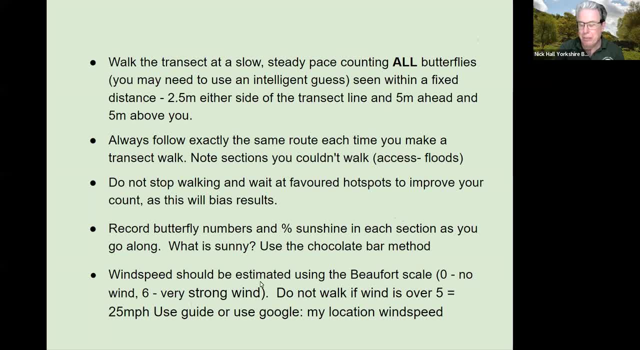 when it's 30 mile an hour and more, In other words, blowing a park gale If the wind speed is over Beaufort scale five and there's a description on the F2 form which gives you a guide as to that. 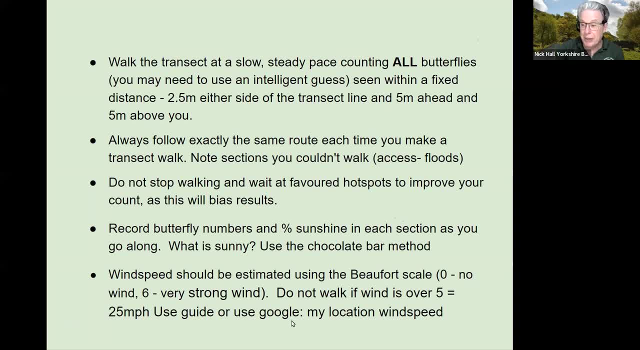 If you're not sure what it is, it's dead easy to find out If you've got your mobile phone with you. just Google in my location wind speed and it'll tell you precisely what the wind speed is at that moment in time. 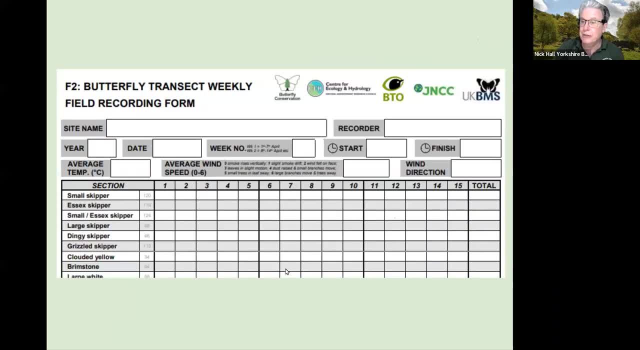 So that's a little handy tip, And when I'm talking about the F2 form, I'm talking about this chap. Very good idea to fill this in when you're a beginner. Site name, recorder, name, year. the date, the week number. 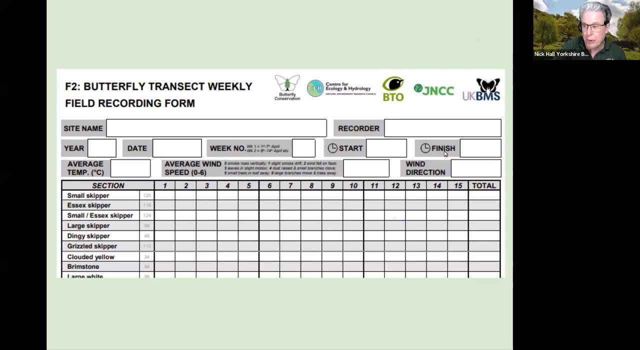 the time you start, the time you finish. That's really important. They need to know the speed at which you're walking. So the distance is fixed. And these are two variables: speed of your walk, The average temperature. I tend to 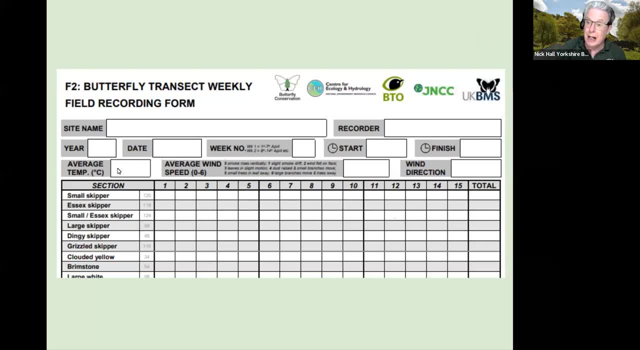 as I drive to the site I look at my temperature on the car And when I get back to the car I look at the temperature again and take the average of the two Wind speed. I've already done. Wind direction is optional, handy to know. 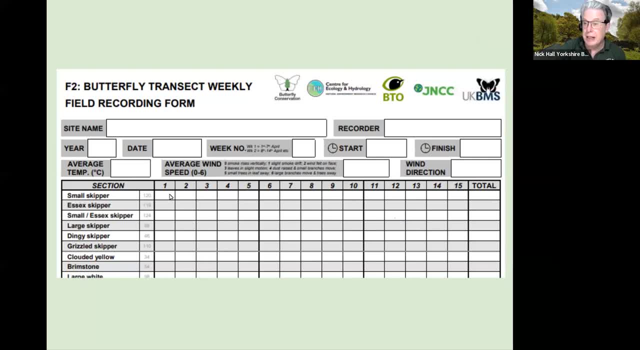 And then you write down your different species number in each of this. These are the sections across the top And these use species down and then below. How most people do it is on a notebook and they do it in groups of five. 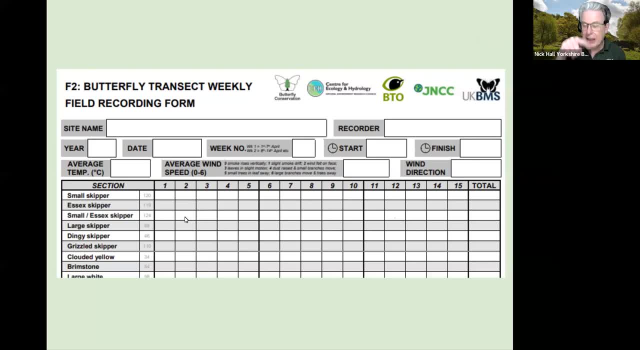 and they put the dash, a horizontal, a vertical line, and then, after four, the fifth one, you put a slash line through it. If you're very, very numerous, I count them in groups of five in the head to save on paper, make it easier. 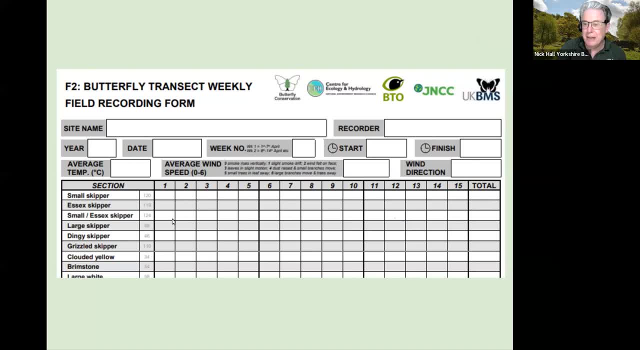 Just put five down, five down. It keeps it very compact. You keep it on a small notebook then, rather than carry this big form around with you, which is a bit cumbersome. Yeah, so that's recording. Any questions on that, I can help anybody with. 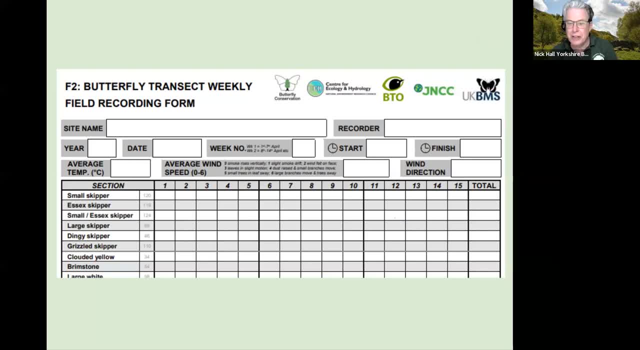 That's a very fast rundown and I've only got 10 minutes left and I have to finish, So any questions, Okay. So Julia asks: do you submit a record for a week that was too cold, et cetera? 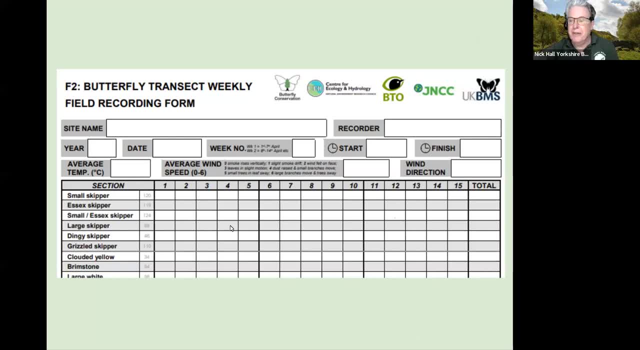 No, If you never find any walk conditions, then you record absolutely nothing. You just leave it blank. Please don't be tempted to walk in conditions which are not suitable, because they will immediately be disregarded by the other end. So you have to try and meet those conditions. 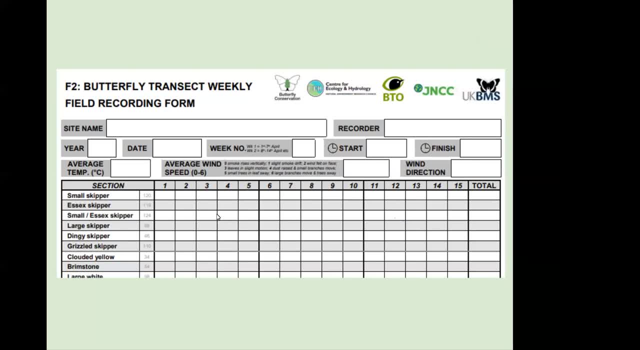 through part of your transect. Can I just ask about something that I think I'm guilty of? The transect that I walk is Up on the top of the hill. Well, no, I suppose it should be lowland raised bog. 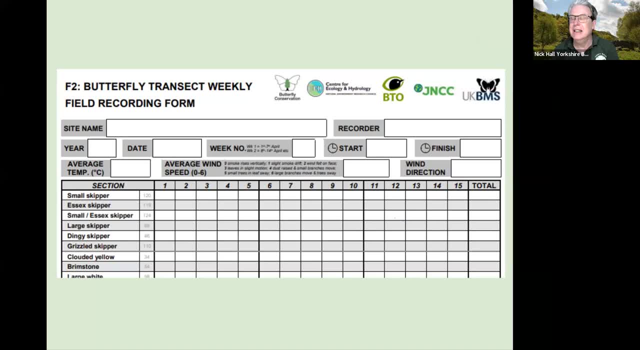 but a lot of it is very tussocky, very rough, Yes It's. you know, sometimes it's really hard just to stay upright on your feet as you walk. Yeah, And I don't think I do very well at looking up. 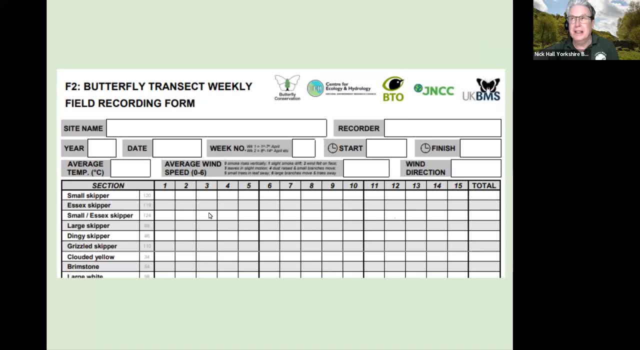 Five meters, Okay, Because you know I'm looking down to see where I'm walking. Any tips? Oh yeah, Rely on instinct. So your instinct, which comes as you develop your skills, Tamsin you suddenly and probably totally unaware. 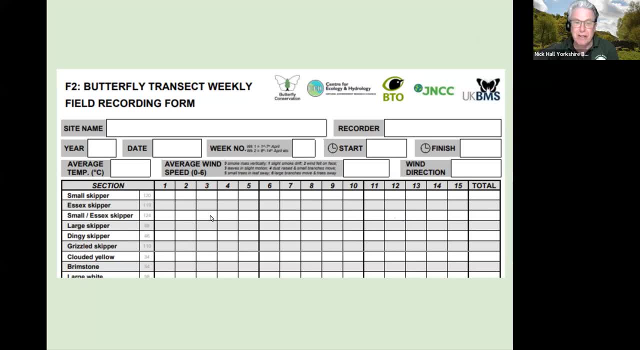 that your peripheral vision becomes super sensitive to movement, And I think I don't. I don't ever look up, unless I'm looking particularly at looking for a hair streak, you know a purple hair streak or a white-letter hair streak. I never bother to look up. 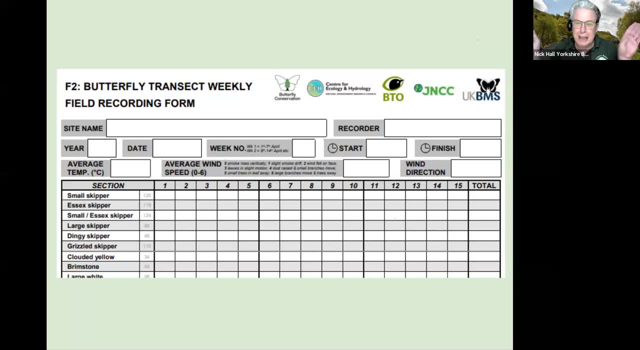 Because I'm relying on my side vision, which is incredibly sensitive. As you record butterflies, I think it's one of those great feelings that you get is this heightened sense of awareness. So I wouldn't worry about it And you don't. 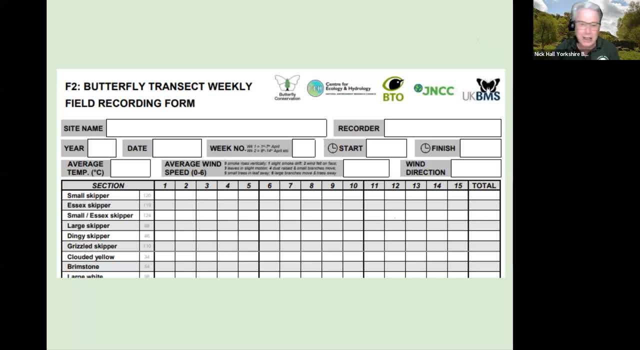 I tend to just walk with my head going slightly side to side, like I'm watching Wimbledon somewhat, But only a little bit. Only so my side vision. I cover the whole 180 degrees. No, rely on your instincts, Tamsin. 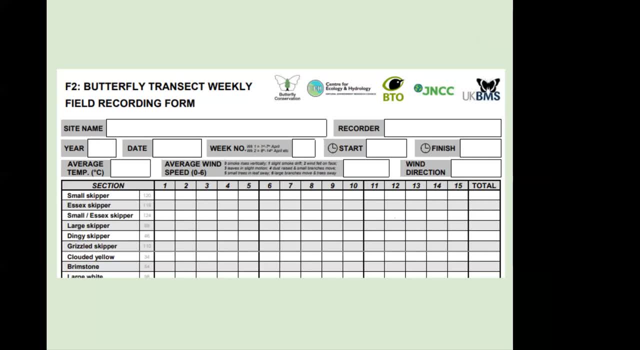 Don't worry about looking up, You don't need to. Okay, thanks, That's reassuring, But yeah, If you see movement and it looks like a butterfly, your brain will quickly compute. I think that you should then alter your focus to something that's flying higher. 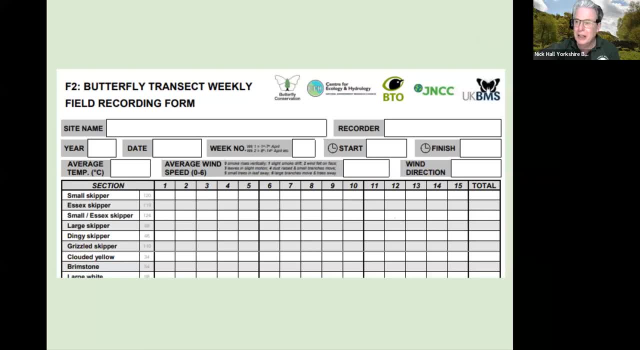 So rely on your instincts. So, Nick, we've got a few more questions. So Ricky asks: how would you manage maintaining the speed of the transit walk if you are bombarded by lots and lots of butterflies? That's a really good question, isn't it? 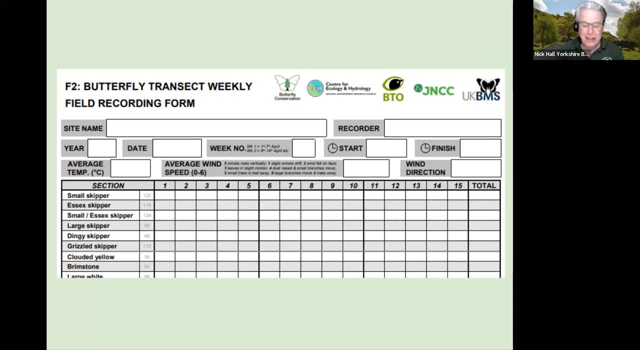 The first rule is you've got to record everything. Develop shortcuts, like I was describing, with using your notepad and dashes and slash, you know, put four vertical, then put a line through. You can almost do it without looking down, So you keep your eyes focused. 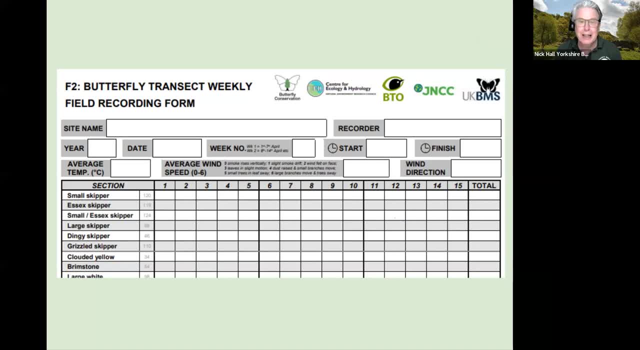 The more time you can spend looking and the less time you spend writing, the better able you are, The more able you are to maintain your speed. But you will slow down. The important thing is you don't duplicate as you slow down, Because there is the temptation as there are more butterflies. 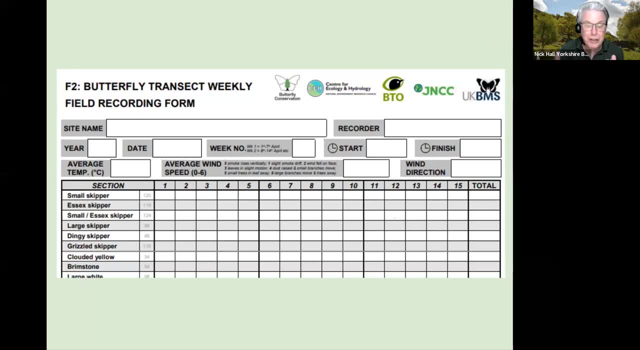 is, there's more activity around you, There's more likelihood of double counting. So I classify them as bouncers. and there's more likelihood of double counting Once they go up and down where you're walking, particularly if you're on a long open area. 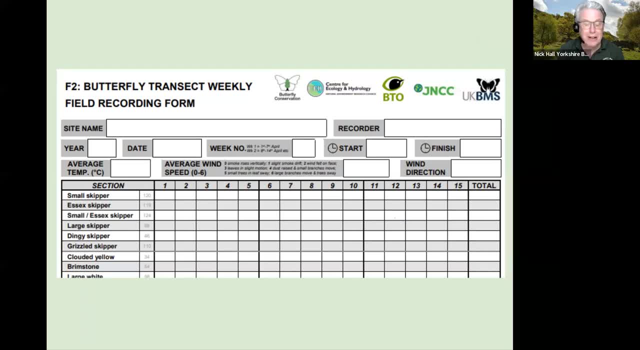 you get patrollers going up and down, And if they're in large numbers you need to have a strategy to deal with duplication. So I suffer with large numbers of silverwashed fritillaries which tend to go up and down and up and down. 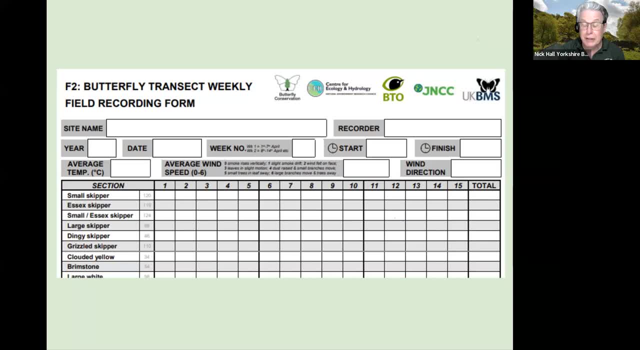 And brimstones that go up and down and up and down, And brimstones that go up and down and up and down, And brimstones that go up and down and up and down, And so, if they're in large numbers, 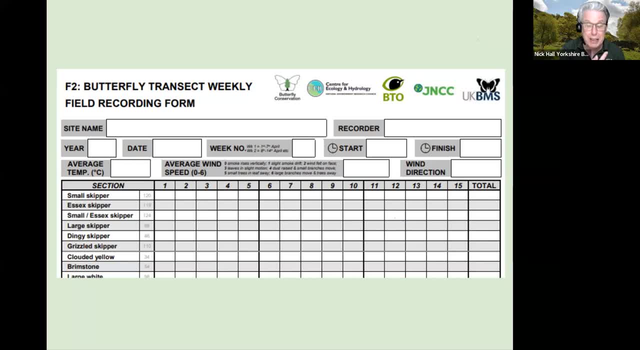 I only count them when they're coming towards me, So I'm not recording ones that are coming from behind me. By the way, you should never turn round to count the ones behind you. That's cheating. You can follow one with your eyes. 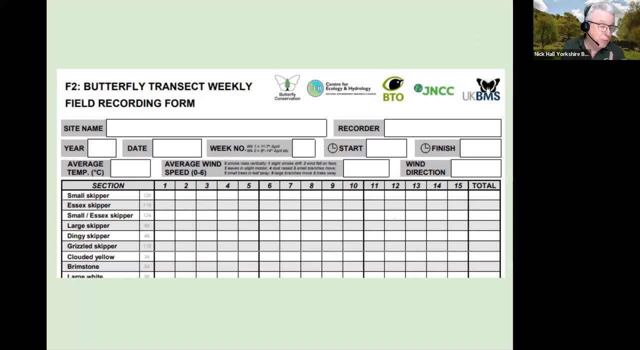 So when it goes behind, you follow it to see what the ID is, But it must have flown through your box before you count it. That's the important thing: Bouncers. Bouncers are, and peacocks are devils. 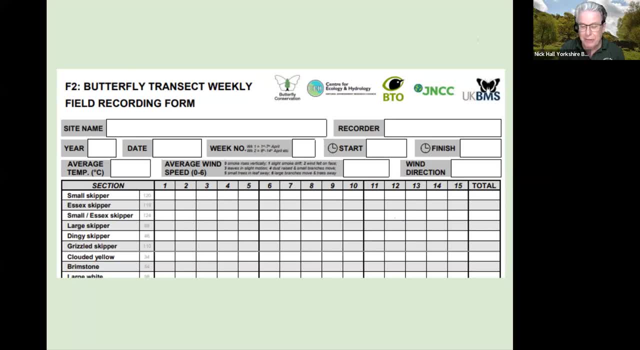 Commas are devils. They'll land a few feet in front of you. You walk to them, They take off and they bounce to another spot about another two yards in front. Somehow, you need to keep a mental note of those species that tend to do that. 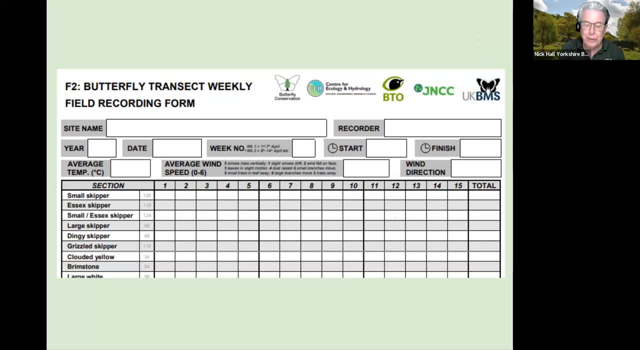 The bouncers, The Vanessa's, tend to be devils for it. Just bouncing, Bouncing in front of you. It is a skill and it's important that you keep moving forward, because the more you move forward, the less likelihood that you're going to double count. 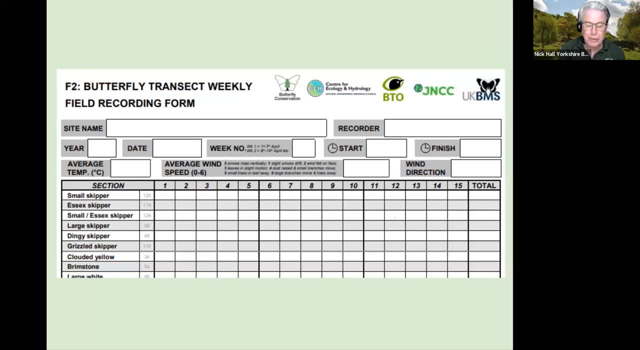 So try and keep it steady, Try and find shortcuts with writing stuff, Try and keep your eyes alert, Be aware of patrollers, Be aware of bouncers And keep going. That's the best I can do. There will always be a bit of duplication. 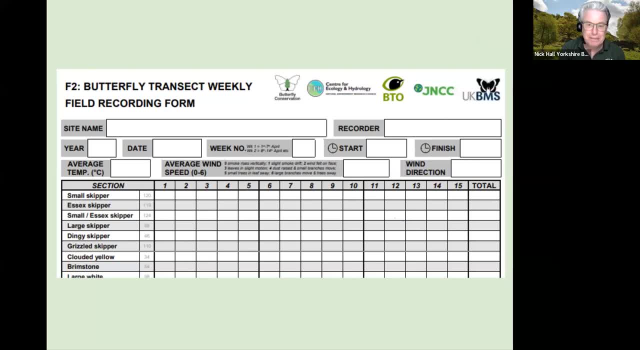 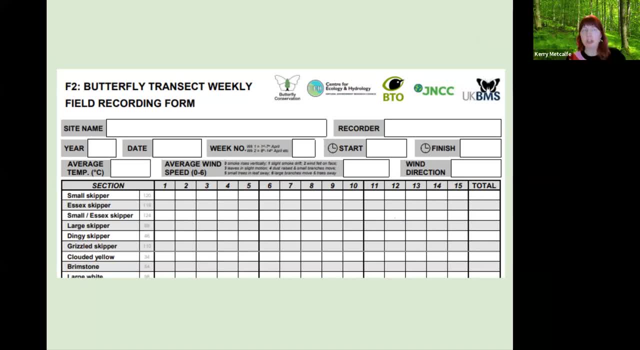 And hasn't done a transect before. So he gets the principles, but he's just wondering if it's possible to get out and go and have a walk around. Walk around With a potential patch: Is strands all common? I think that's one of yours, isn't it, Nick? 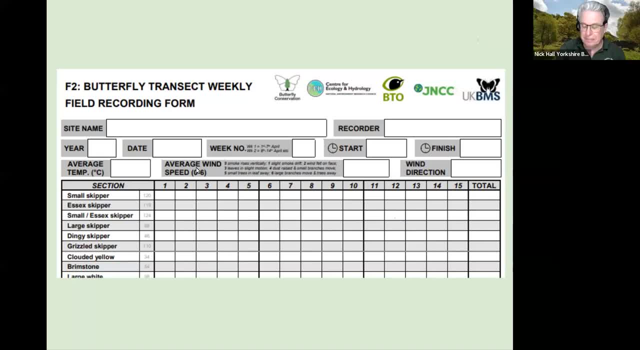 Oh right, Yes, Yeah, Um, Um, Get out there and yeah, if you want to join and just shadow somebody on a team, then it's up to me and you, me and Kerry- to put you in contact with the team and get you some experience. 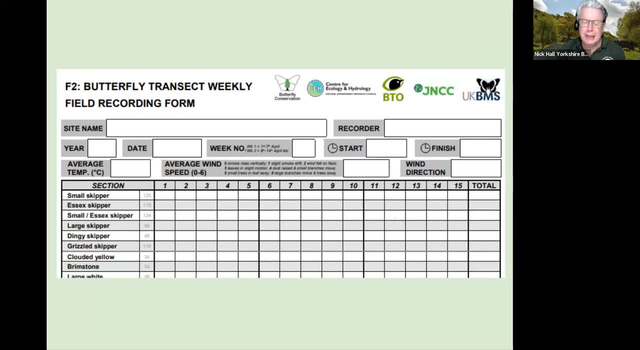 I think I know the Jeremy in question. Yeah, So very happy to put you in contact with the team there. They are actively looking for helpers, by the way, Jeremy, So it'd be great to have you on board. Uh, thank you very much. 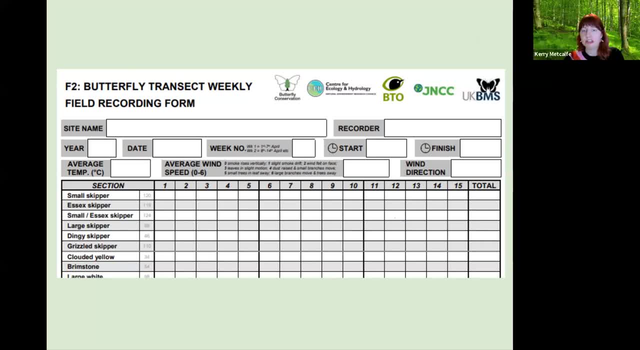 Definitely. Yeah, It's really helpful to get out and go around with somebody and just get it's. it's easy talking about it in um, in a, in a, a meeting like this, but nothing beats actually going out and doing it. 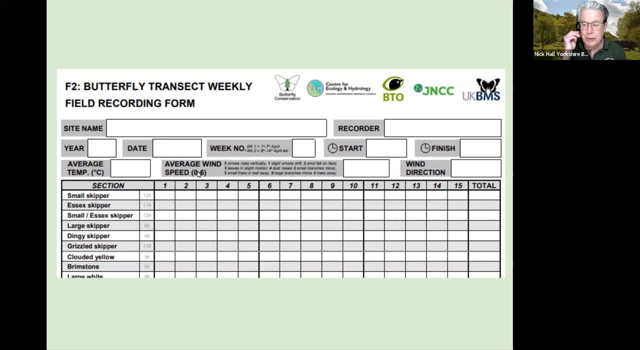 Some people walk in pairs because one is social and two you. you learn from one another. Um, it's important that only one person does the actual observation and the other one does the recording, but it's a nice way of working. It's working as a pair and you learn much quicker from each other. 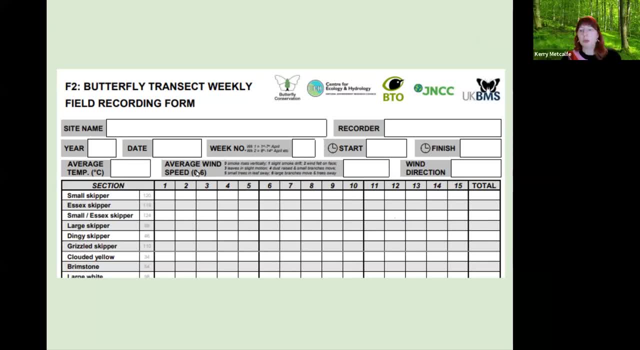 Yeah, Yeah. Um, Nick, we're at just gone nine. I'm just wondering whether you want to. I know you've done all this moth. Um, I have. I spent hours on this moth thing. We we're we're happy to send the presentation. 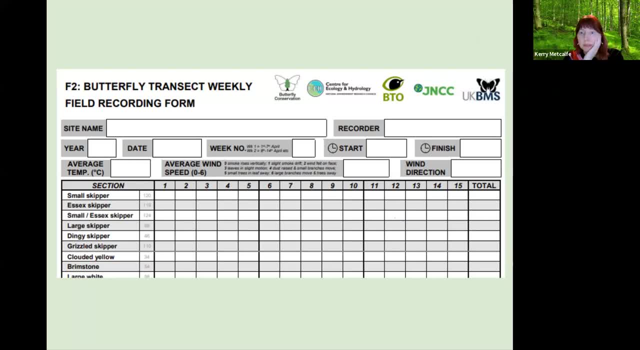 The slides are out as well, aren't we, So people can benefit from them. Yeah, I mean we could also run another session on day flying moths. We could, Yeah, Yeah, Yeah, Yeah, Yeah. Once people can put it in the, put their comments at the end there if they would like to. 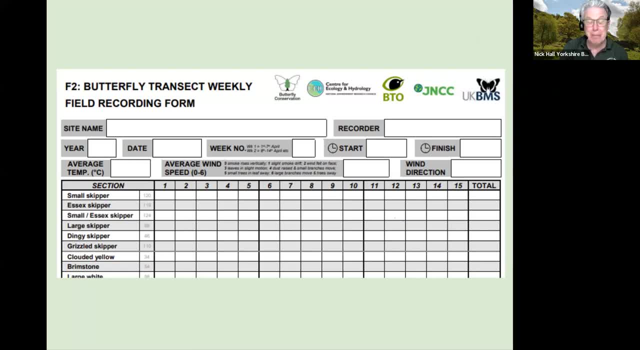 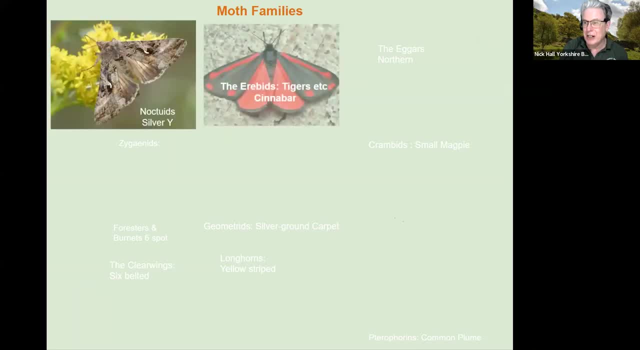 Um, oh, but I'll just do. I'll just do the first slide and then then pack in immediately. Yeah, Carrie, be assured I'm not going to carry on, but, um, how, how we're going to do it is actually go through. 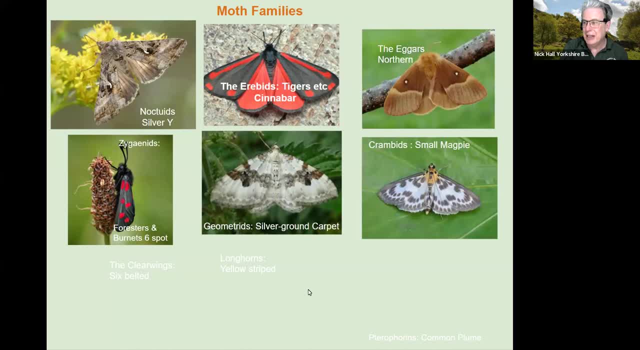 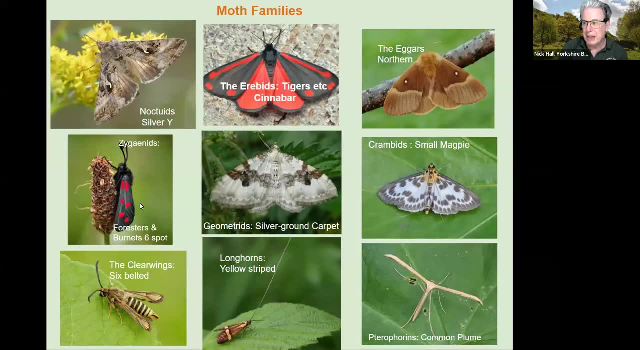 the families, Like we did the uh um, the uh, the butterflies. uh, we're only going to cover, uh, four of the families. So these four here, um, basically highlight, uh, uh, how we tell them apart. 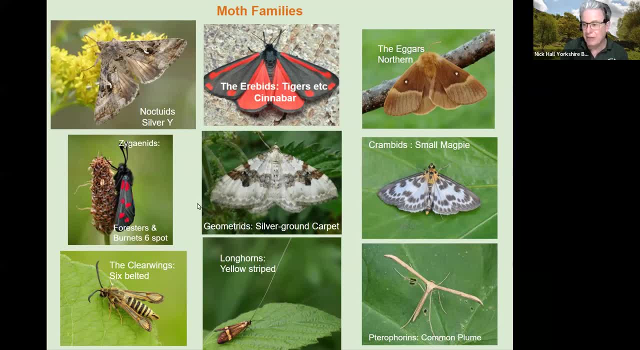 Um, it'd be a lot quicker than the the butterflies. I've done 31 species, of which I experienced all of them in my uh on my transect. So if anybody wants to to learn those, then we'll run them. uh, rerun it a different time. 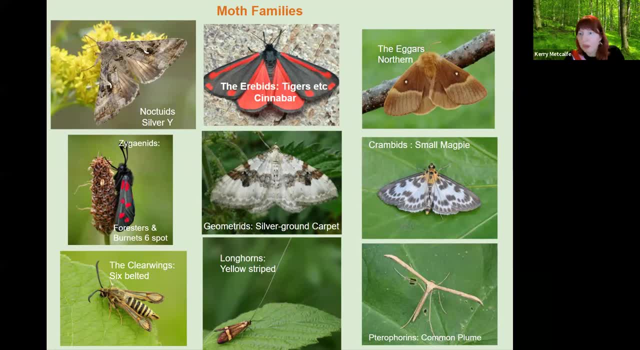 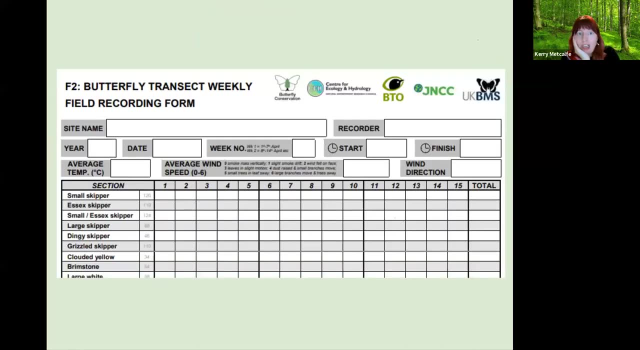 Oh, back to you, Carrie. Um, yeah, thank you very much. everybody There's, um, we're saying in the comments that session on moths and yeah, I think it's worth doing that. You've gone to all that, that work, and it's actually quite interesting and also quite 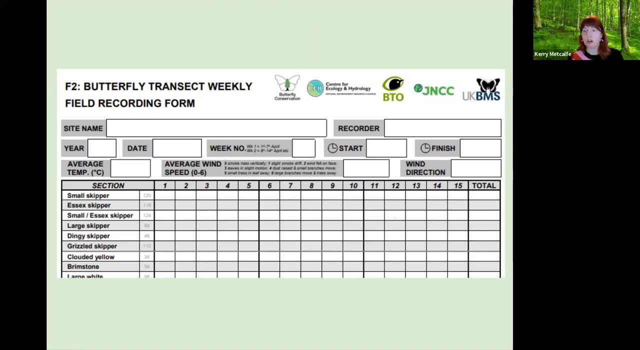 important data to to be gathering. So shall we? shall we get that organized and and send another invite out? Yes, Lovely, I think. then, unless anybody's got any more questions, we'll wrap up there. So any more for uh, for any more. 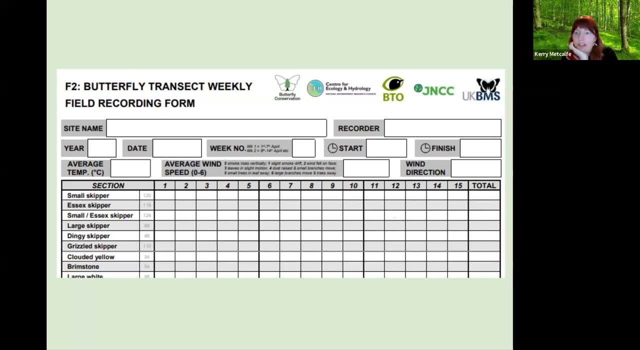 Nope, I think we're sorted All right. Thank you very much for coming, everybody, Nice to virtually meet you, and we'll send out an invite to the moth session shortly. Thank you very much, everybody, Until next time. Bye for now.